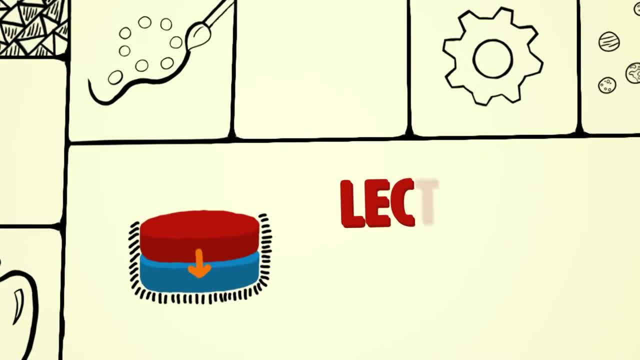 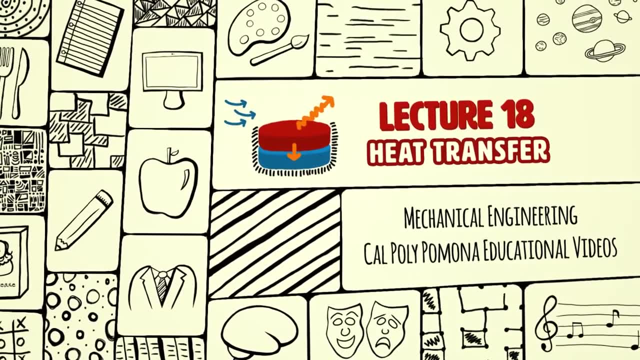 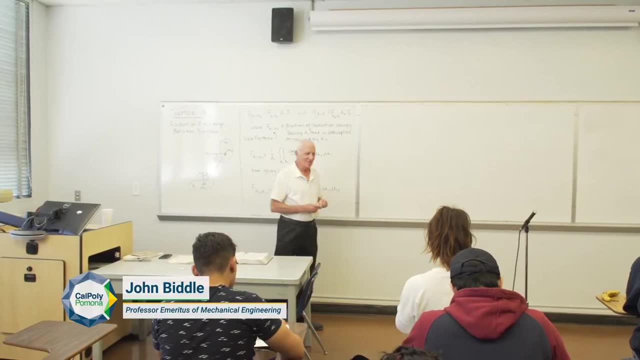 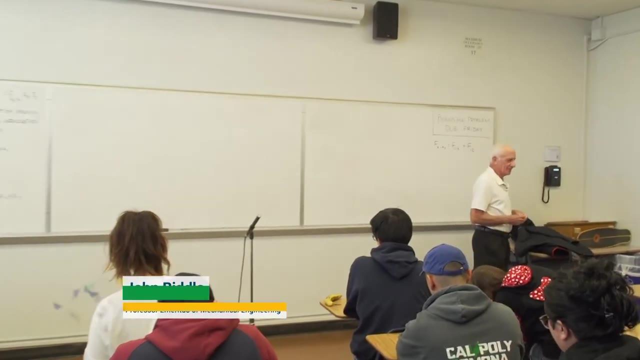 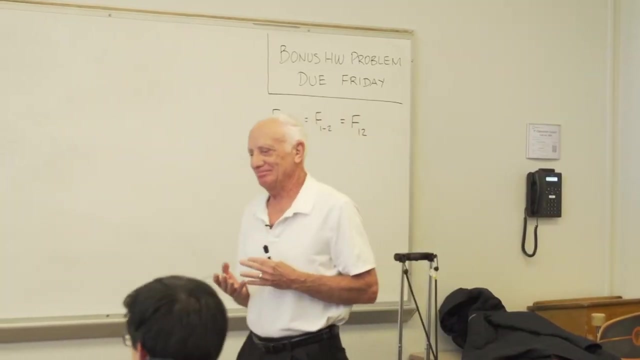 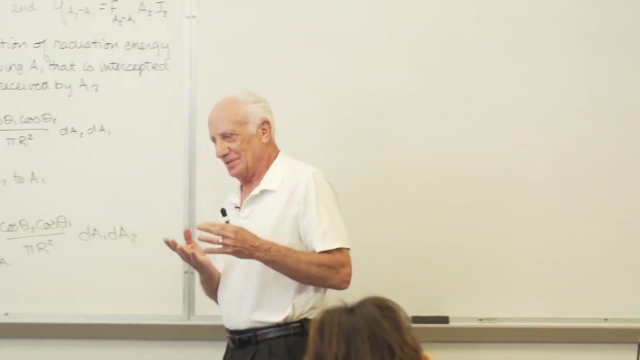 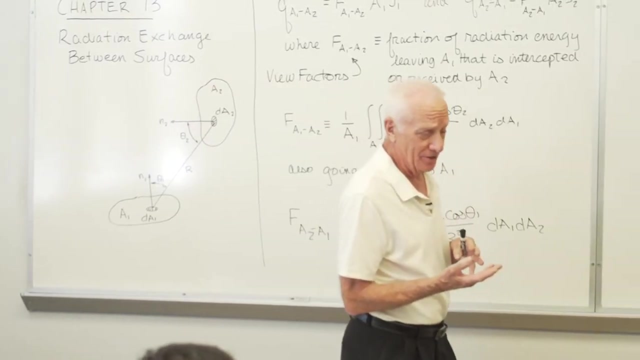 As we said, on Monday we finished Chapter 12 on radiation and today we begin Chapter 13.. Chapter 12 was heavy on the science approach to radiation physics. Chapter 13 is more inclined to be the engineering part of radiation. Chapter 12, there was a lot of definitions. 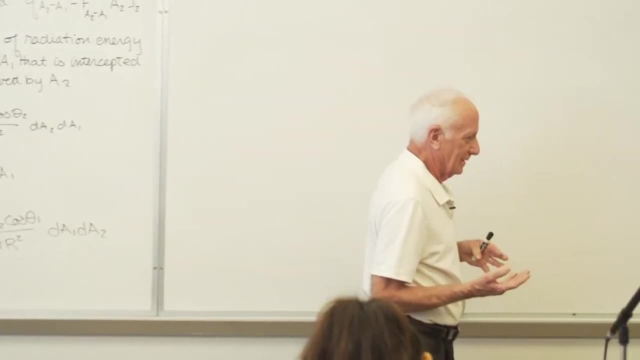 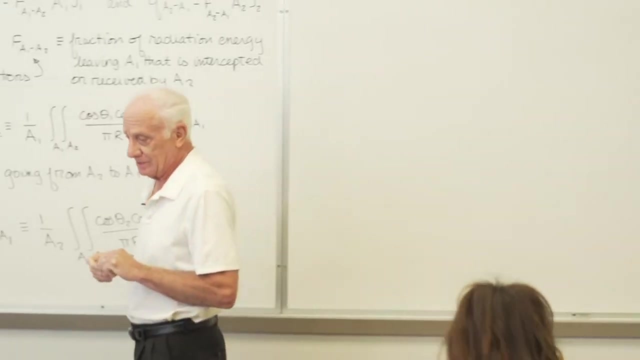 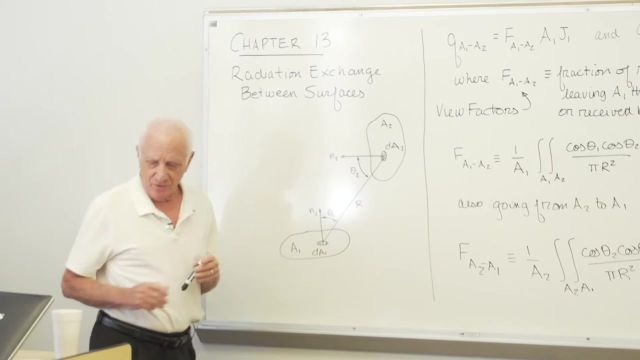 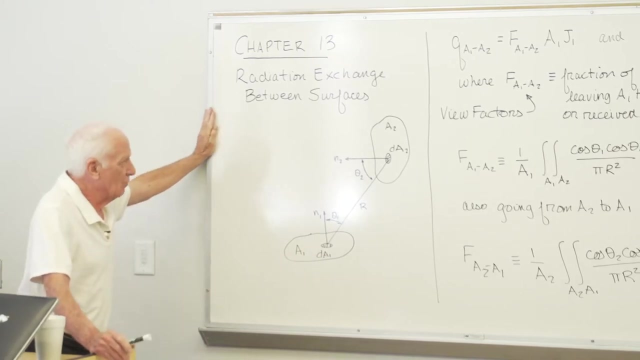 a lot of vocabulary and Chapter 13 is titled Radiation Exchange Between Surfaces. So now we get into some of the real engineering applications of radiation heat transfer. To begin with we're going to look at two surfaces exchanging radiation surface, A1 and A2.. 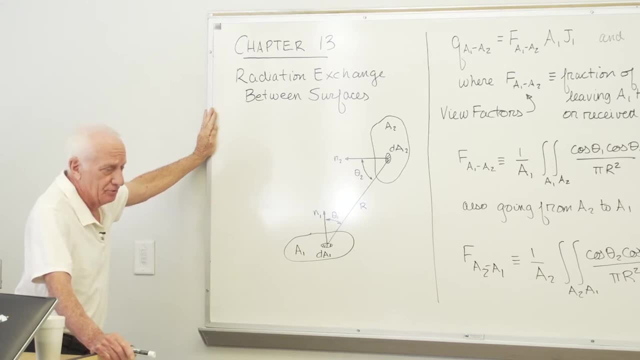 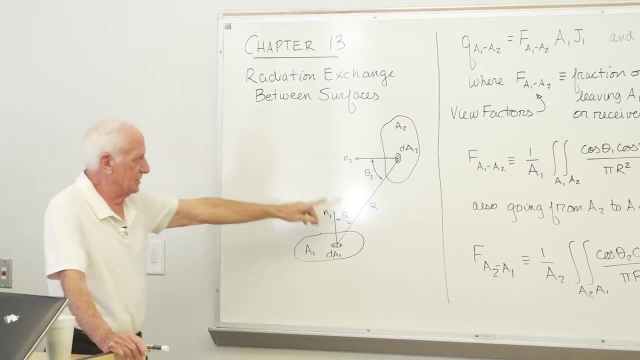 We identified differential areas on those two surfaces, DA1 and DA2.. They're separated by a distance, capital, R, and they're oriented with different angles. theta, Theta 1 is the angle between the R distance and the normal distance to surface DA1, called N1. 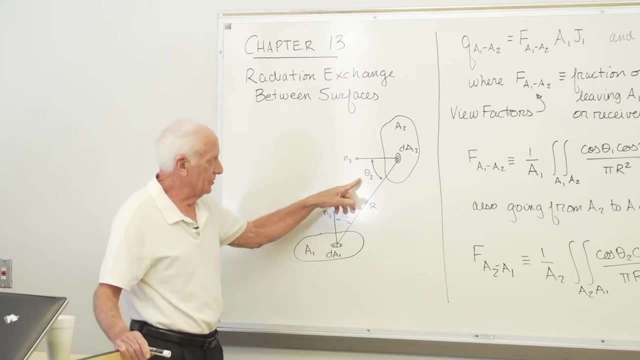 N1 is normal to surface DA1.. Theta 2, the angle between R and the normal to surface DA2.. N2, normal surface DA2.. We want to find out how much energy leaves surface A1 that reaches surface A2.. 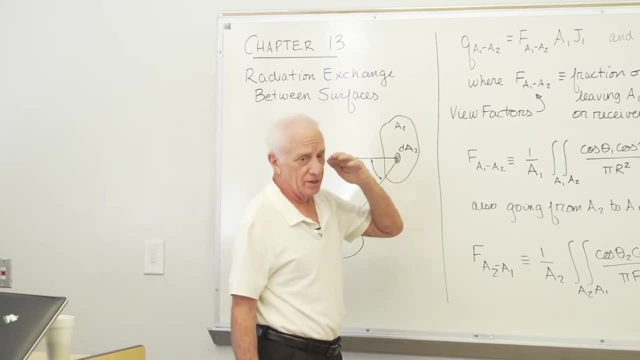 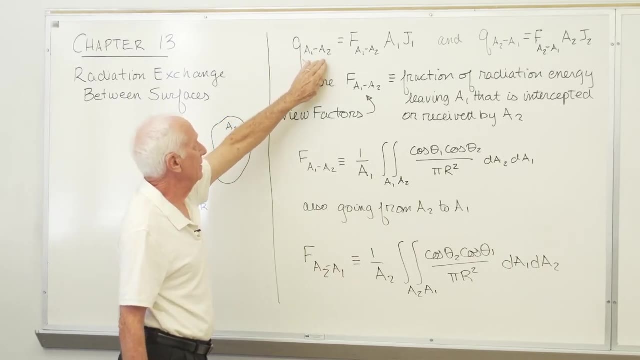 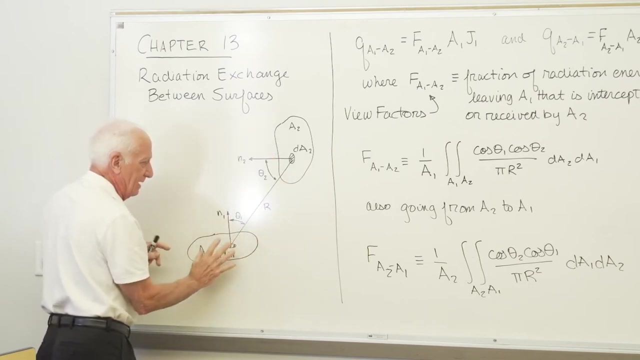 So here's the equation that we're going to use Q, the energy leaving surface A1 that gets to strike surface A2, we can say: intercepted by A2, received by A2.. But this energy leaving here in all directions, some of the energy leaving A1, is going to end up going to A2.. 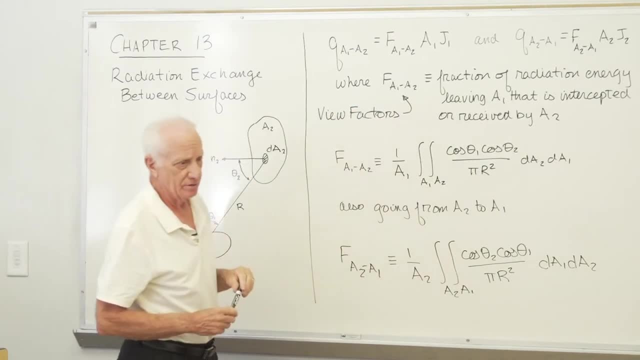 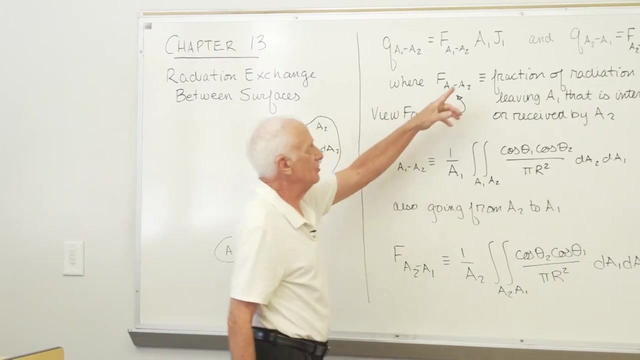 That's FA1-A2, the fraction Fraction means between 0 and 1, 0 percent, 100 percent or something between. I multiply that fraction by the total amount of radiation leaving surface A1.. J1, the radiosity, Chapter 12.. 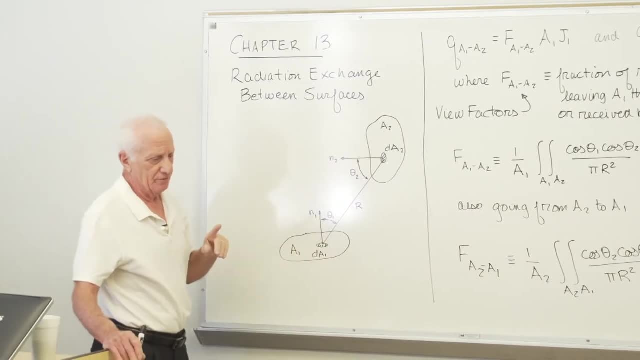 What's radiosity? The energy leaving surface A1, the radiation energy leaving surface A1.. By direct emission: E emissive power plus the reflected amount from some source. G irradiation: J1, watts per square meter multiplied by A1 square meters. 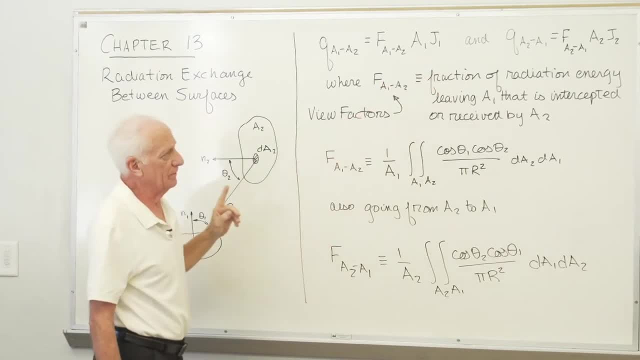 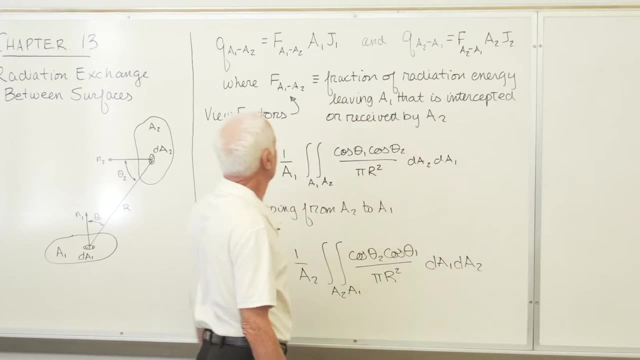 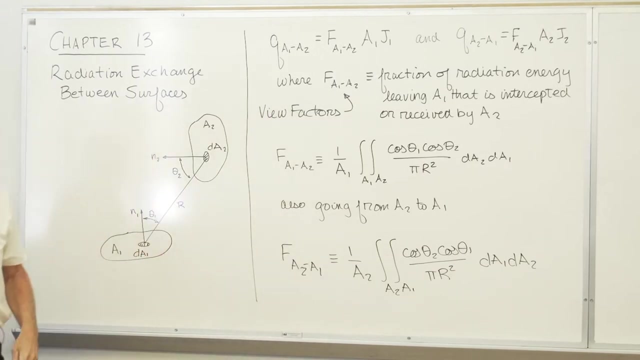 A1, J1, the watts leaving surface A1. A fraction of that ends up reaching surface A2.. That's FA1-A2.. Those guys are called view factors. The F factors are called view factors. We'll get more into the Y in just a minute. 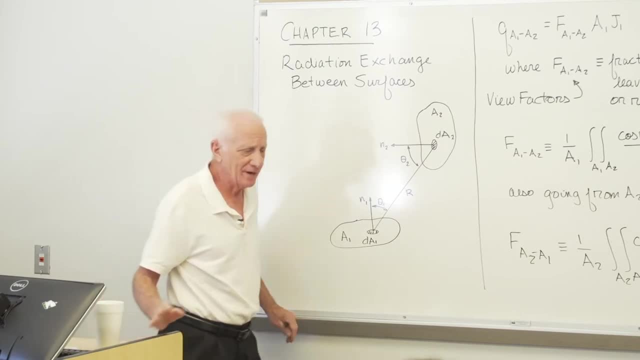 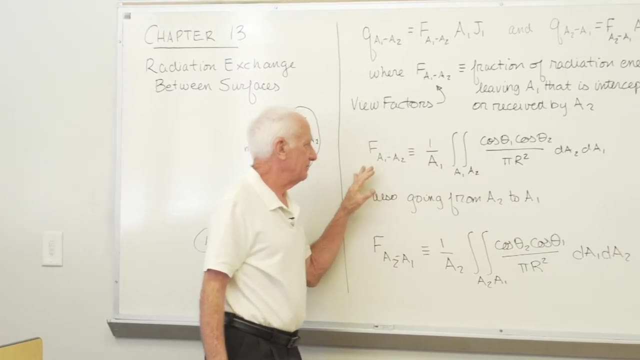 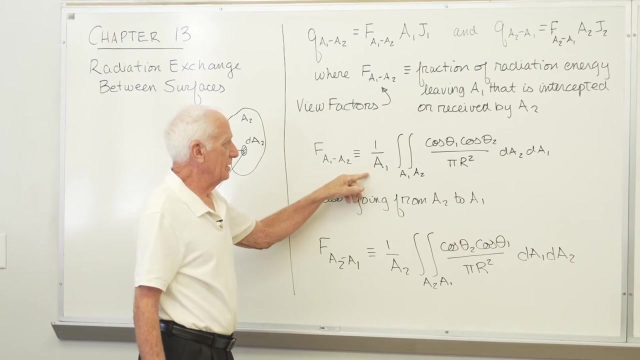 Mathematically. here's how you would find a view factor. Now the book derives this. We're not going to go into that lengthy derivation, But here is the equation that you could use to find the view factor: One over A1 times a double integral A1 and A2.. 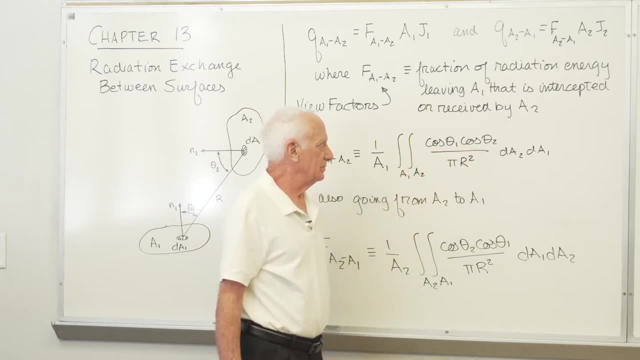 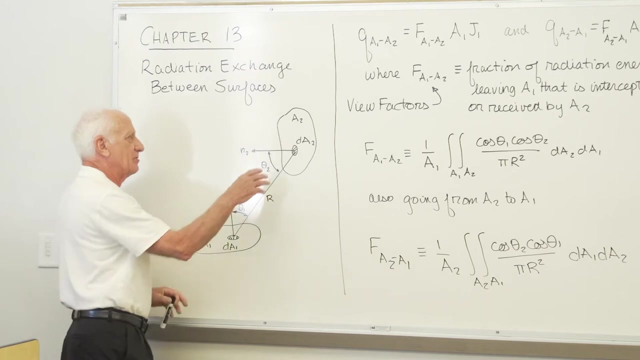 Numerator: cosine theta 1, cosine theta 2.. Denominator pi r squared dA1, dA2.. Double integral rather complex, obviously. Now you can also go the opposite direction. How about the fraction of energy? 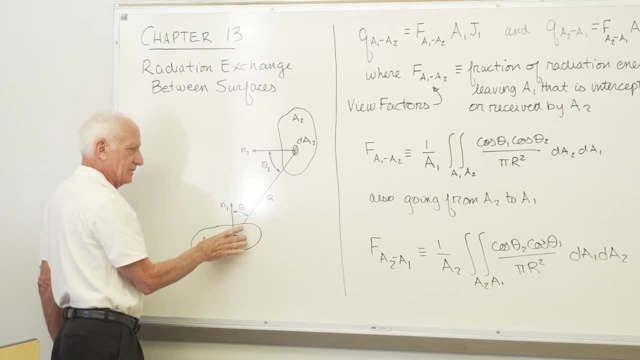 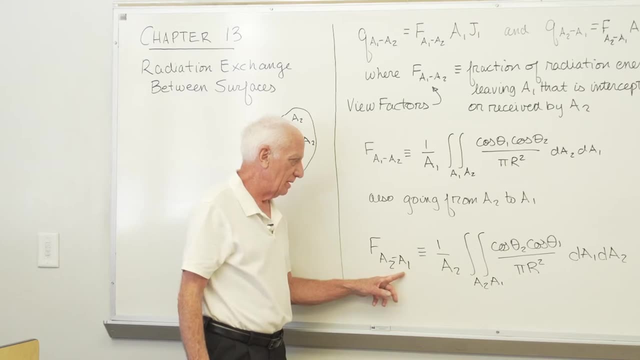 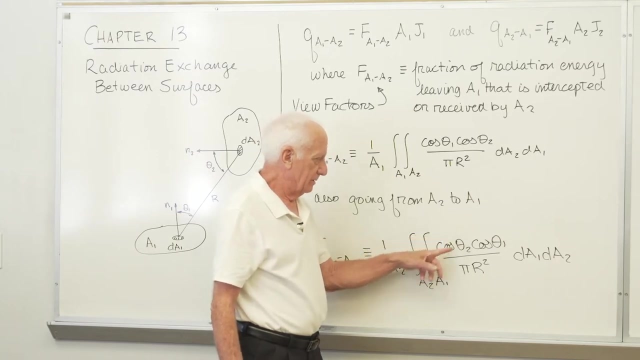 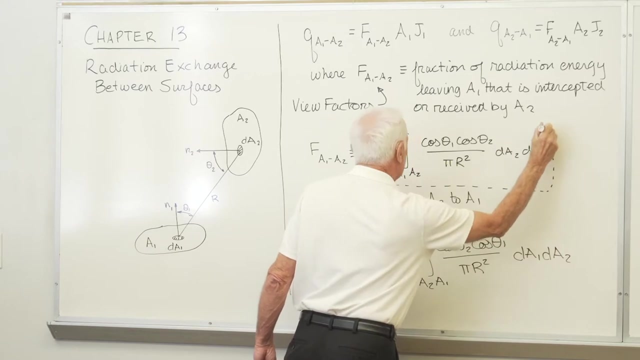 leaving surface A2 that ends up reaching surface A1? Fraction leaving A2 that ends up reaching surface A1. That's 1 over A2, double integral, Same numerator, same denominator there. Then you can notice that this double integral are identical. 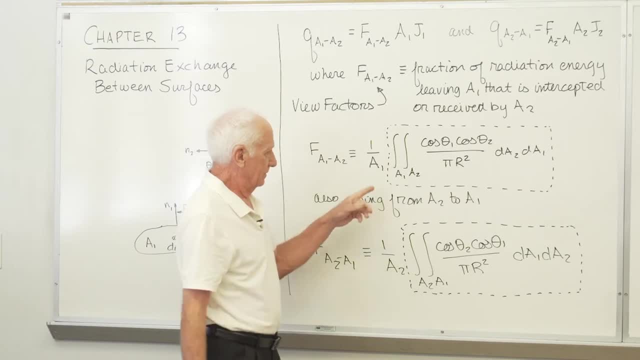 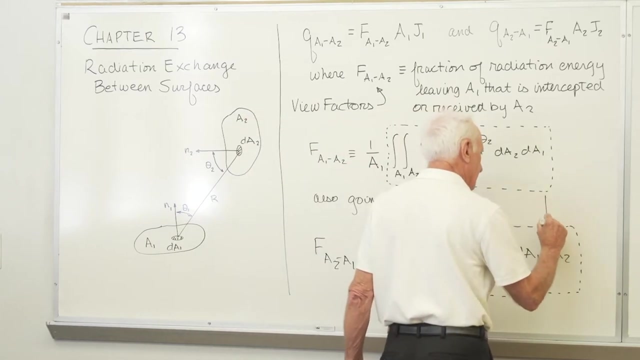 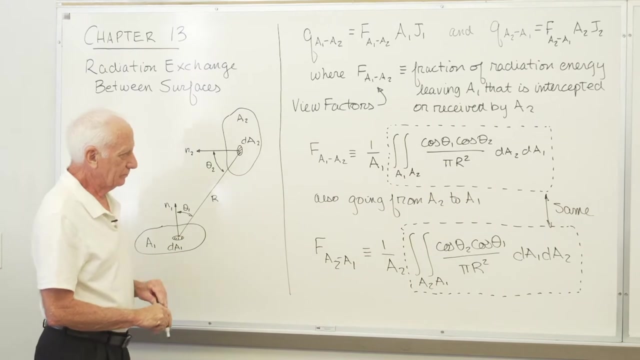 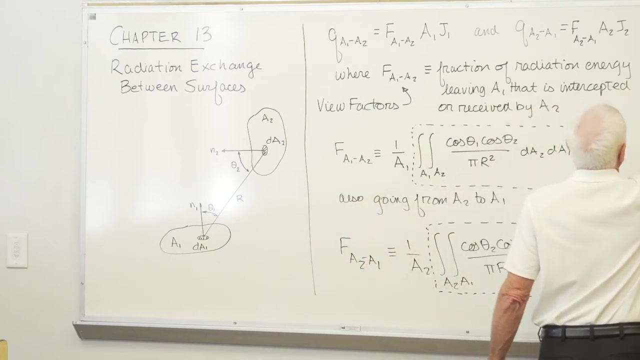 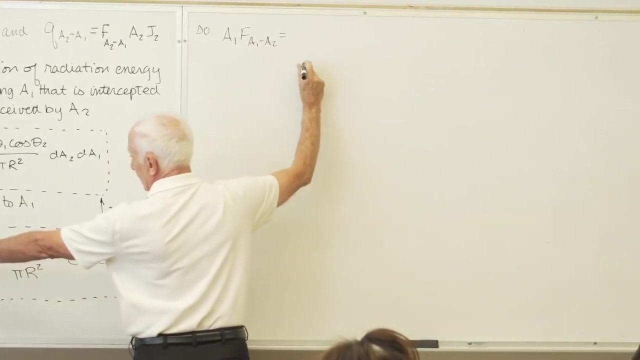 I don't care the order of integration: A2 first, A1 next, A1 first, A2 next. I don't care about that. What's under the double integral is the same. So these two guys are the same. So A1, F, A1, A2 equal, second one, A2.. 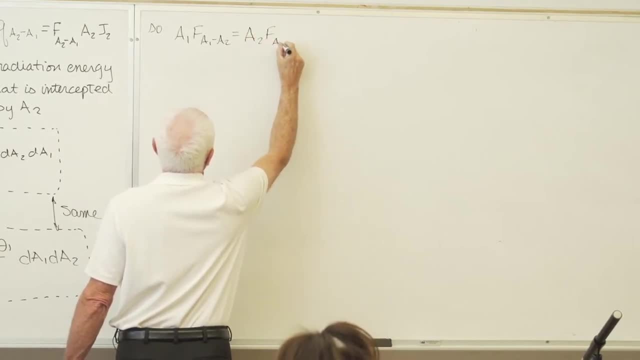 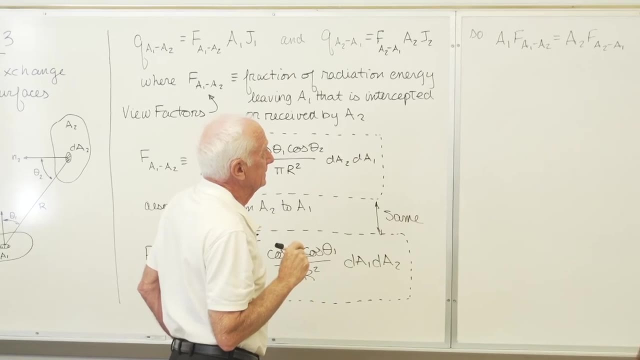 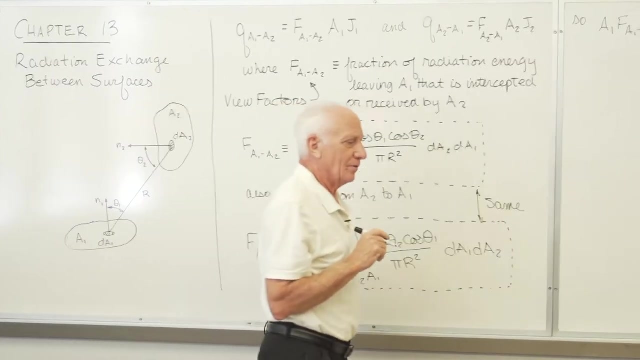 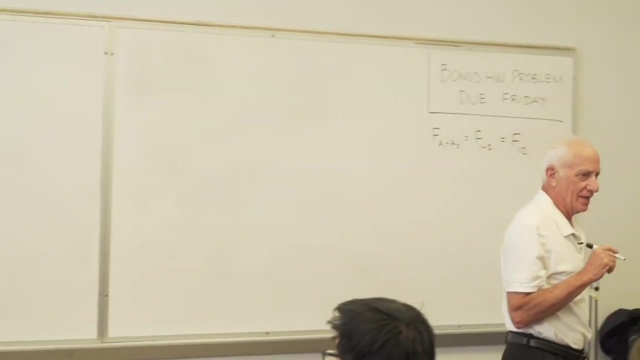 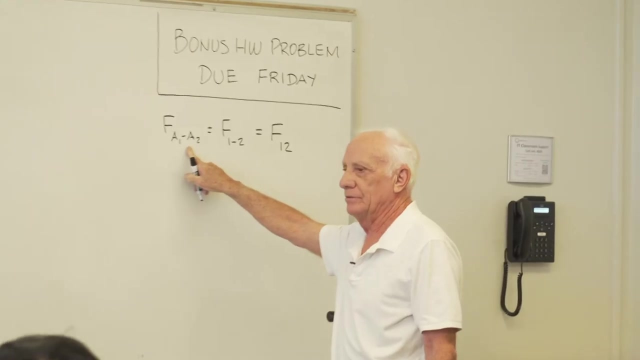 F. F. A2 to A1.. We get tired of writing that A1-A2.. So we take a shorthand notation. Here it is. I'm going to replace the view factor A1 to A2, with F from 1 to 2.. 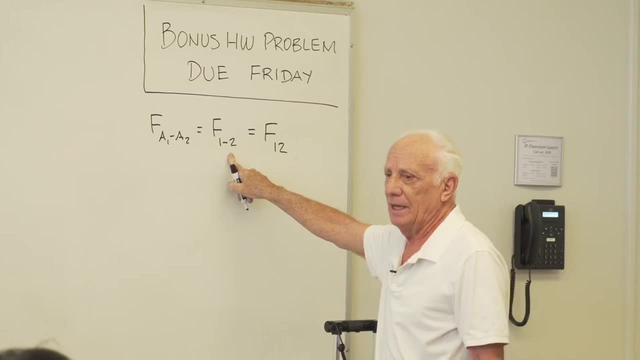 I know that means area A1 and area A2.. I don't need to put the A subscript on it. I don't like the dash. I'm going to call that F12. Don't say F12. It's not F12.. 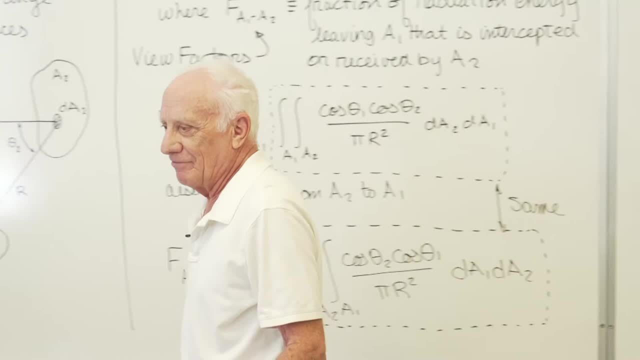 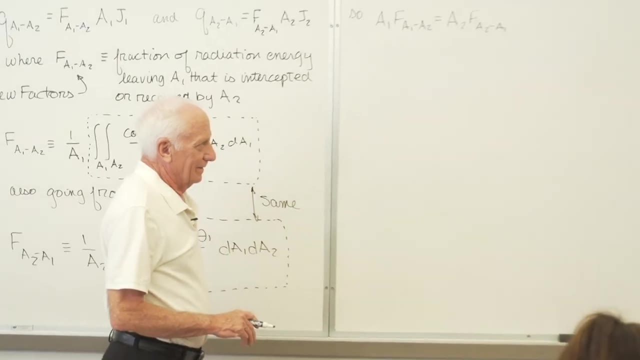 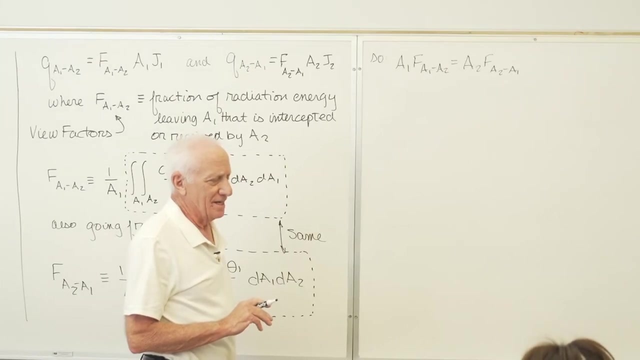 You say F12.. What does that mean? F from surface A1 to surface A2, we call it F12. Especially like when there's maybe six surfaces F56. It's not F56. It's F from A5 to A6,. 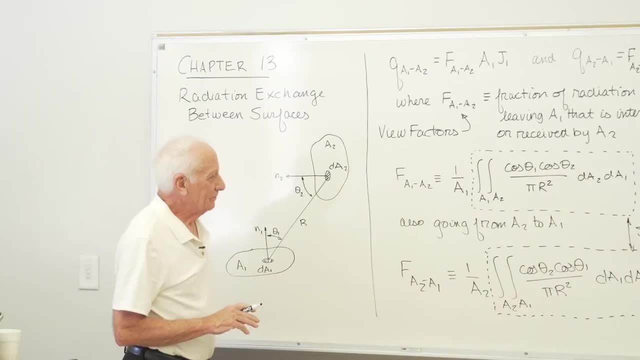 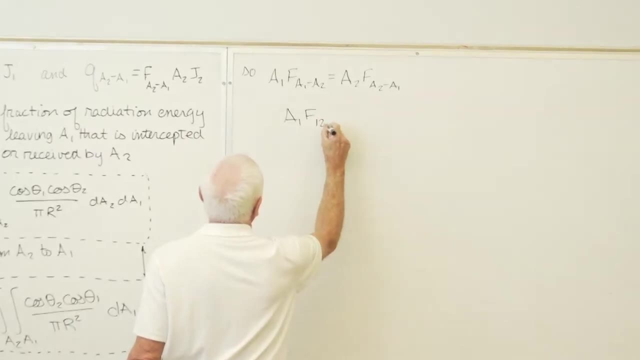 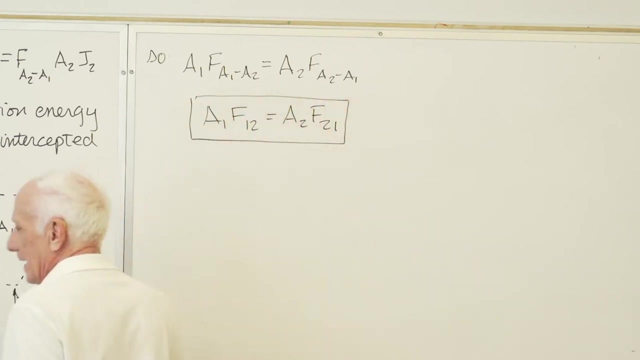 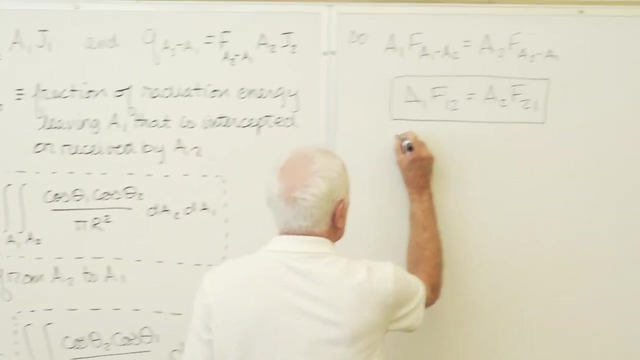 but we say F56.. Okay, So take the shorthand notation A1, F1 to 2, equal A2, F2 to 1.. All right, So that's with our shorthand notation. This guy is reciprocity. 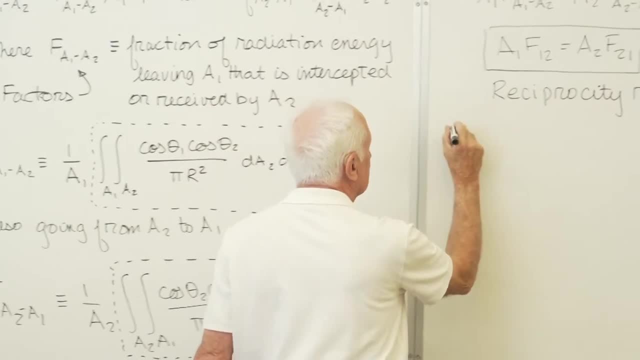 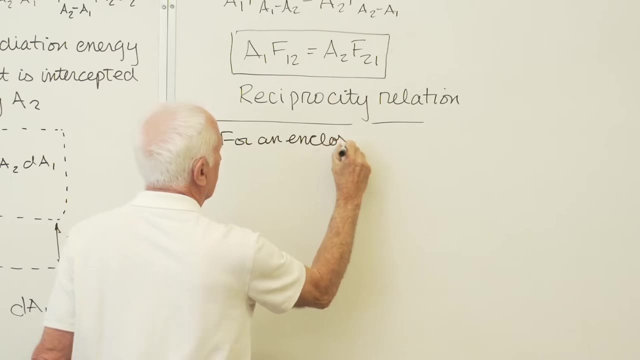 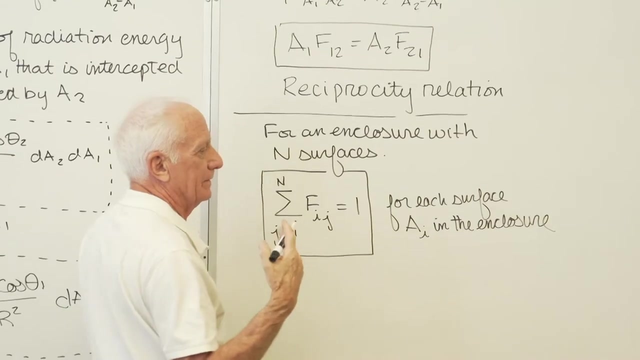 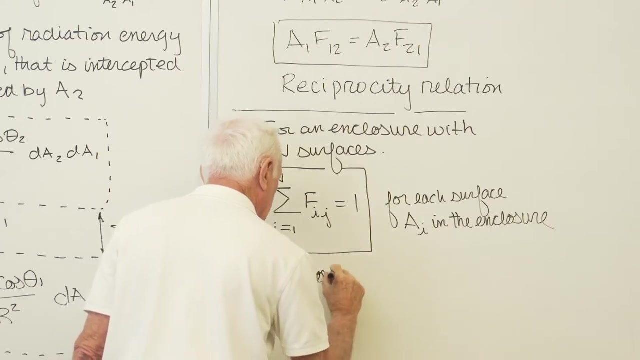 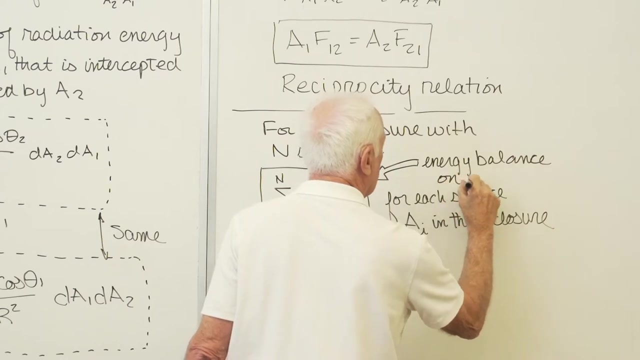 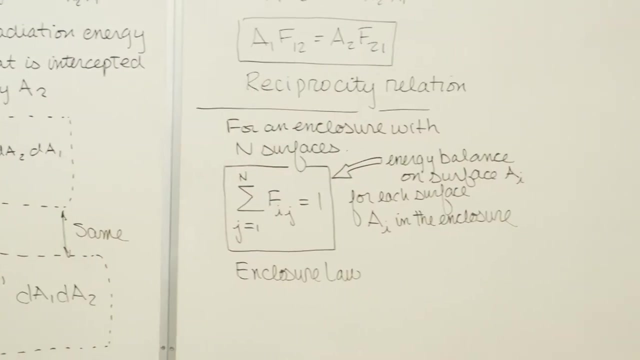 Then, for an enclosure with N surfaces, capital N surfaces, Summation j equal 1 to N, Fij equal to 1.. This guy is called the Enclosure Law. It's the energy balance. So I'm going to. 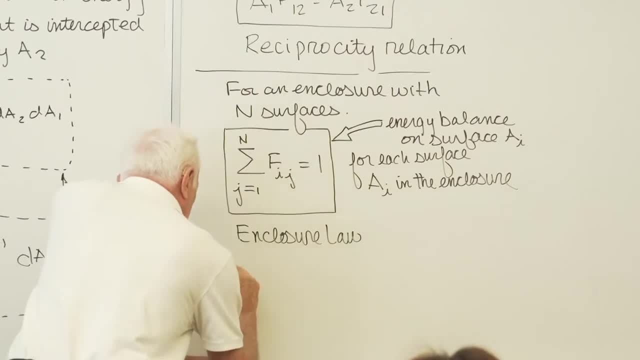 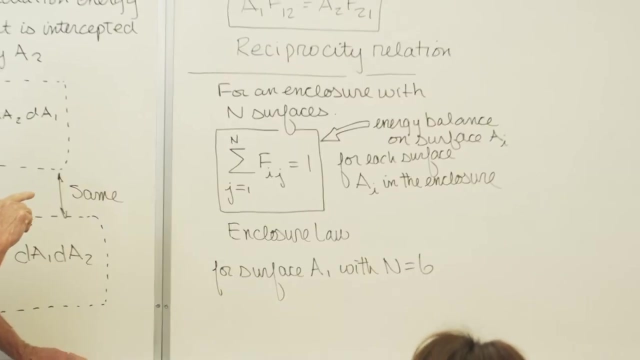 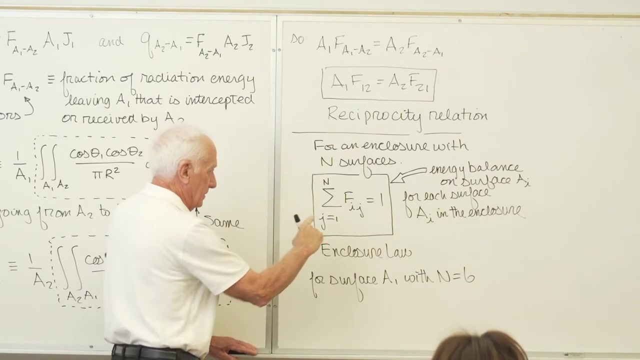 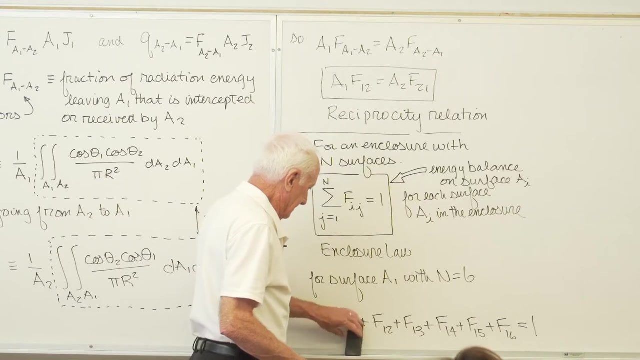 take surface A1 with N equals 6. surface enclosure. I'm going to write this energy balance, the Enclosure Law for surface A1.. So I equal 1.. I'll get to F11 in just a minute, For right now, ignore F11.. 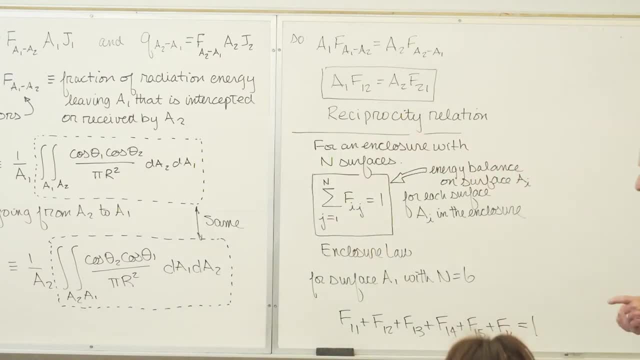 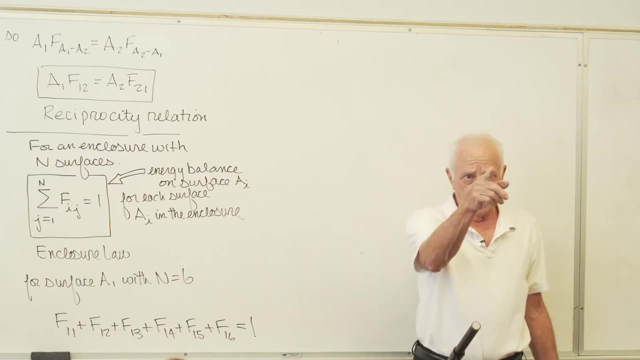 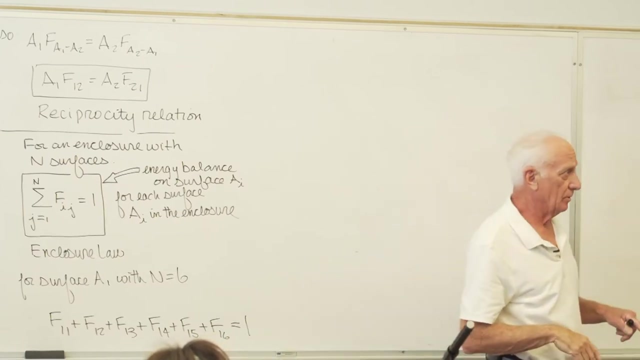 So this is what it says in words. Let's assume in this classroom that the front wall is area A1.. The back wall is A2, ceilings A3, A4 floor, A5 window wall, A6 hall side wall. This is an enclosure. 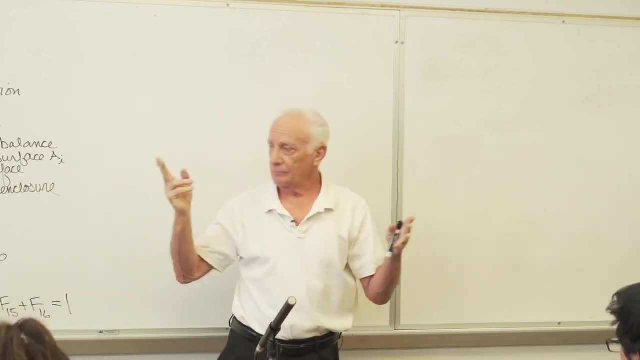 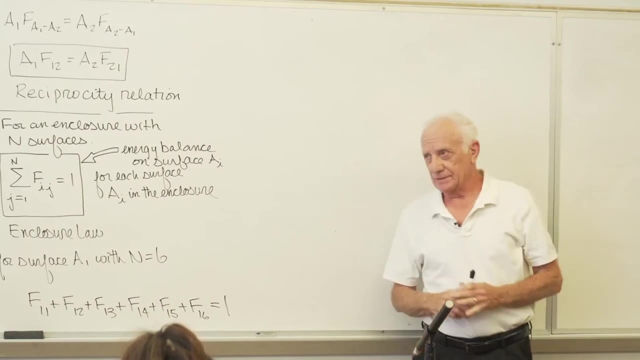 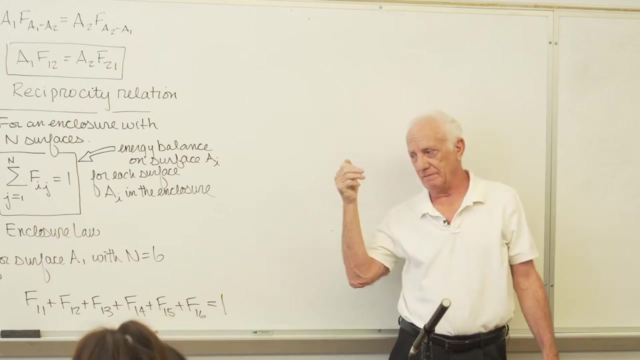 This is a six surface enclosure. Forget the F11 right now. This is what it says: The fraction of energy leaving the front wall that hits the back wall, plus the fraction of energy leaving the front wall that strikes the bottom, the floor. 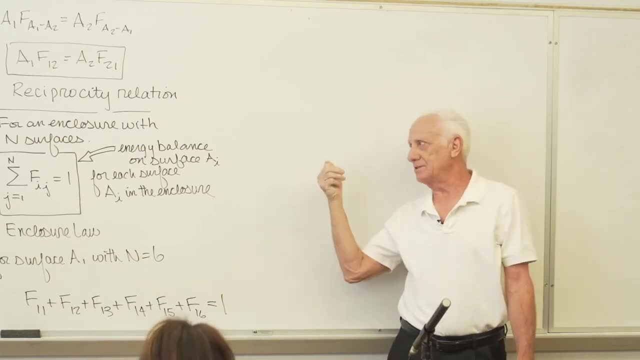 The fraction leaving the front wall strikes the ceiling. The fraction leaving the front wall strikes the window side wall. Fraction leaving the front strikes the hall side wall must be a 100 percent. Where else can it go? Got it? Enclosure law, energy balance. 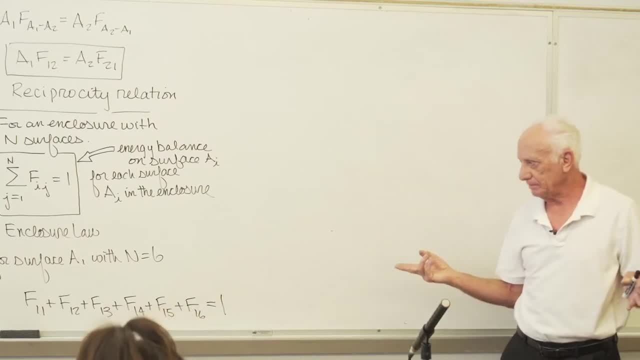 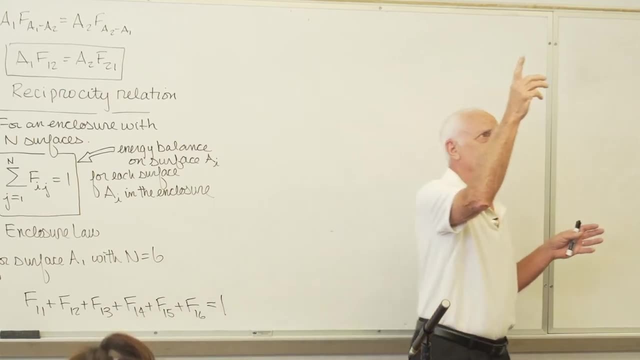 Those fractions must add up to 100 percent Every surface in this room. I'll write it for surface four, the ceiling, The fraction of energy, leaving the ceiling that strikes the front wall strikes the ceiling, front wall plus the back wall plus. 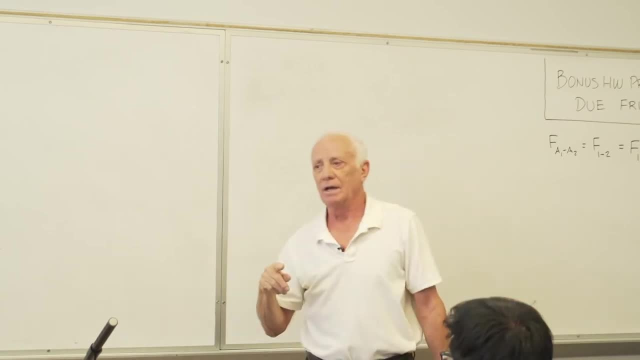 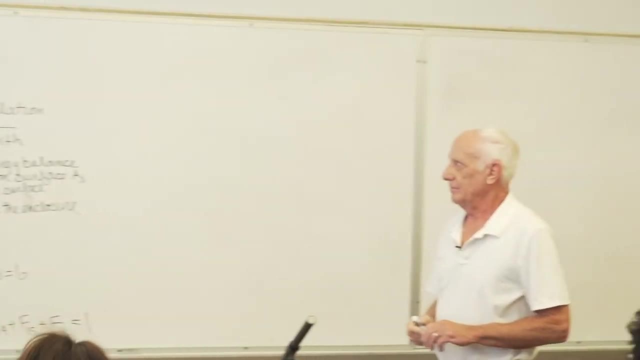 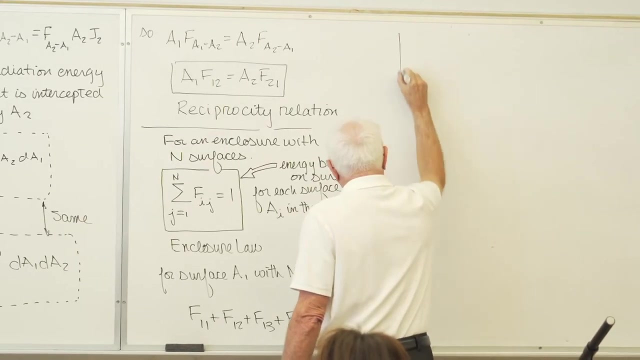 the hall side wall plus the window wall plus the floor must be 100 percent 1.0.. Yeah right, So we have two algebraic expressions we can use: reciprocity and enclosure. Now let's talk about F11.. 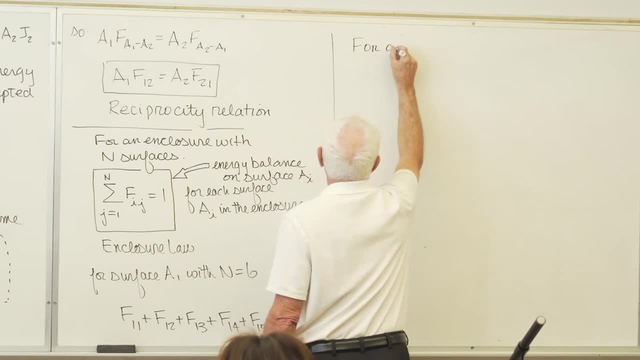 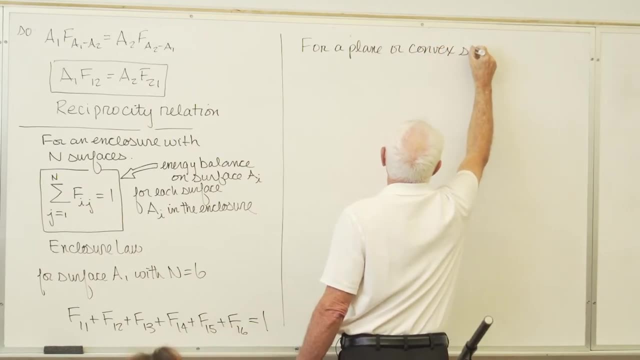 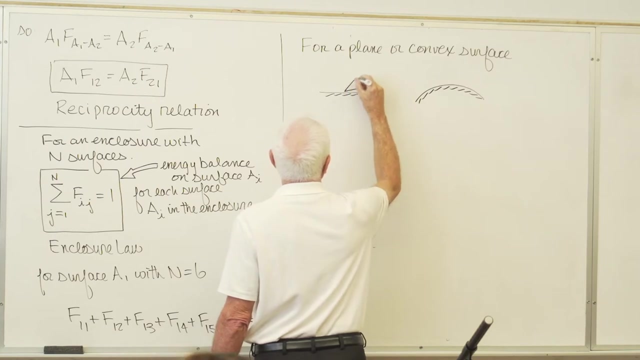 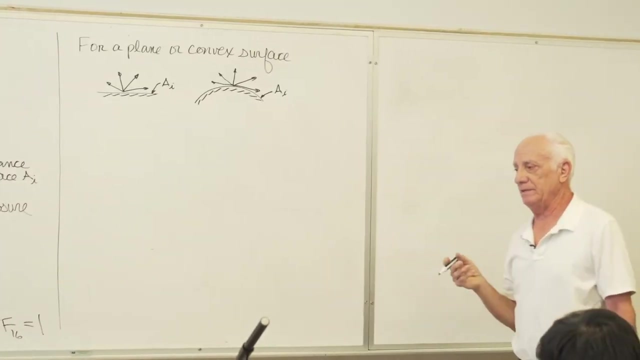 For a plane, our convex surface. Take a plane surface first, Take a convex surface. Radiation, leaving this surface Radiation, leaving this surface. This is surface Ai, This is surface Ai. So what's the fraction? again, Fraction of energy, leaving a surface i. 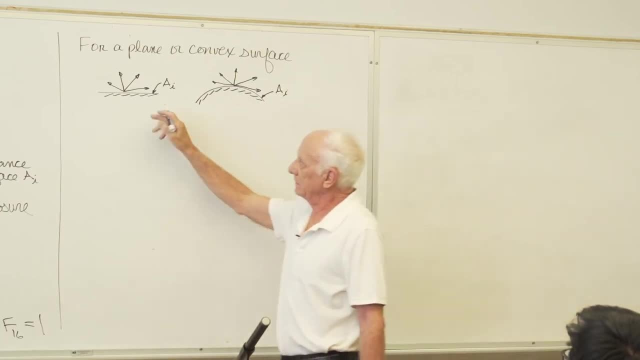 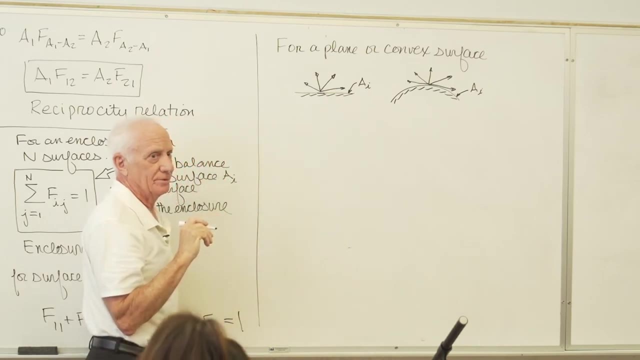 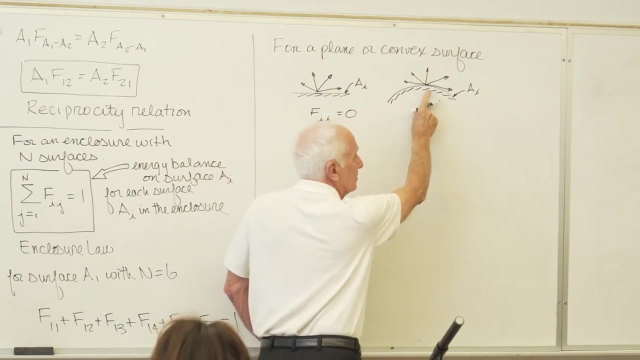 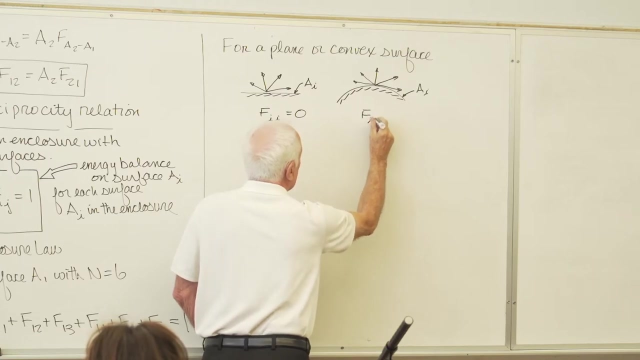 the strike surface i. How much energy leaving this area here ends up hitting that area? Well, look at the arrows zero. How much energy leaving surface i ends up striking directly surface i Look at the arrows zero. What's this front wall? 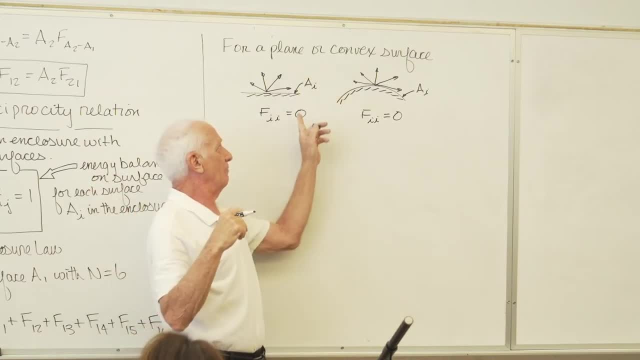 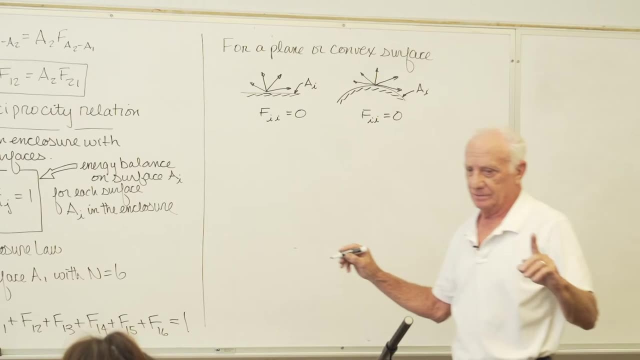 A plane surface. What's F11?? Zero. That's why I said F11 is zero. This is illegal Radiation. doesn't do this, make a u-turn. No, no, no. It goes out straight lines: The fraction of energy leaving. 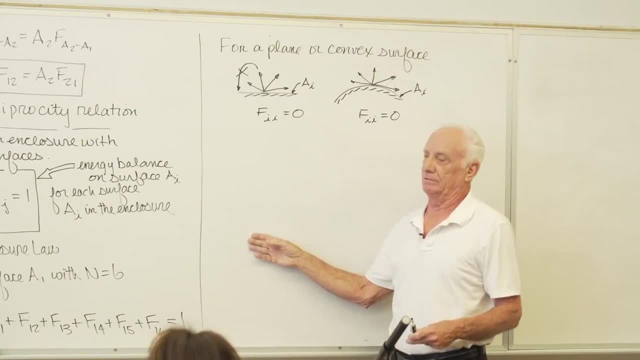 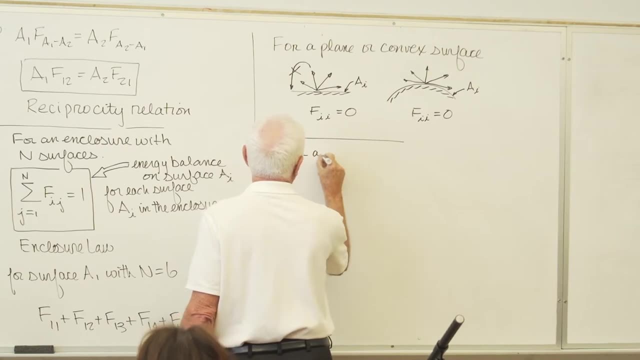 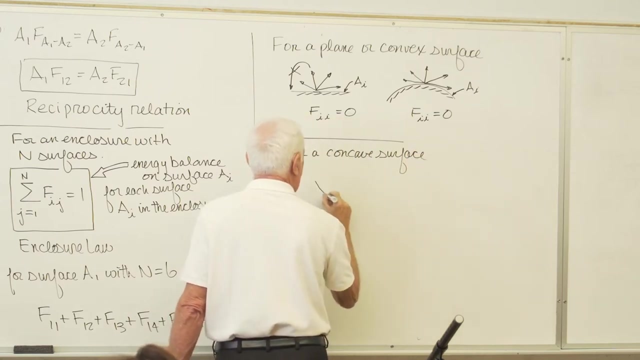 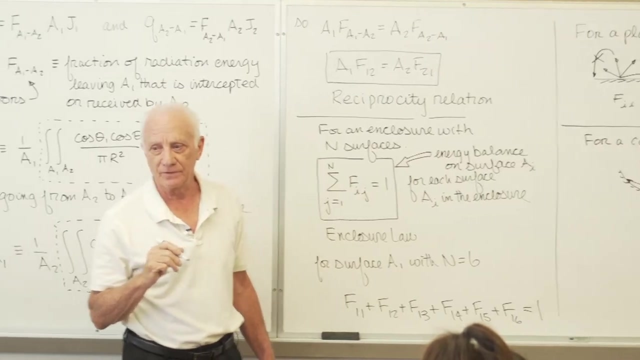 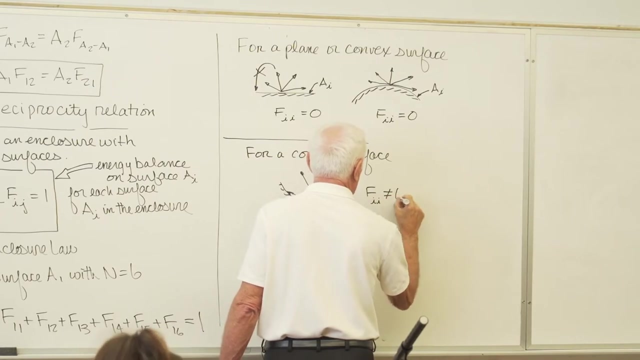 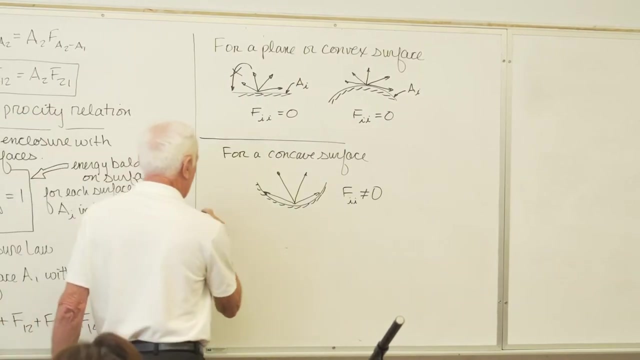 the front wall that directly hits the front wall. zero, Right For a concave surface. Oh yeah, Some of the radiation leaving that surface hits that surface. Fii is not zero. Okay, So now we have some idea Of these guys. 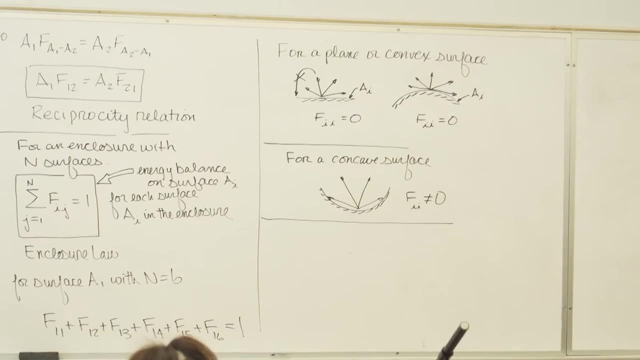 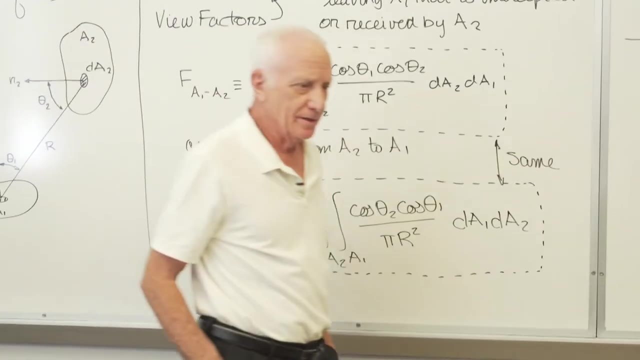 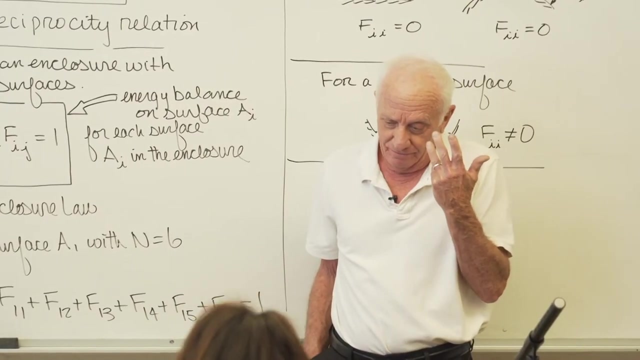 Now, where did it get its name, view factor? Well, there's other names to configuration factors- geometric factor, but the textbook uses view factor. It in a way relates. relates to your view, from your eyes, If I pretend, I'm surface A1,. 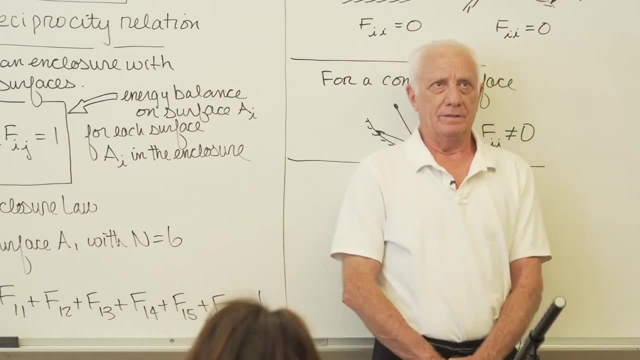 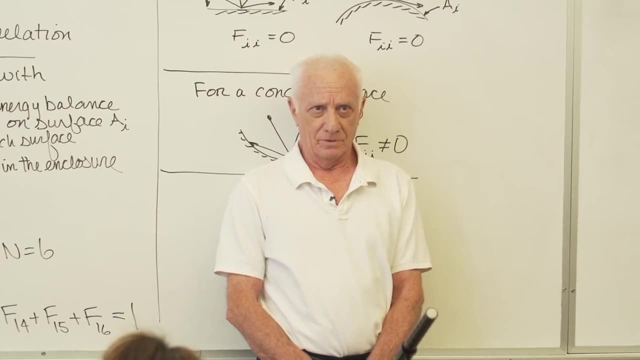 the front of the blackboard and I look straight out. what do I see? the most of The back wall? What do I see the least of The hall side wall and the window side wall? Okay, What's my view? What percent of my view is the back wall? 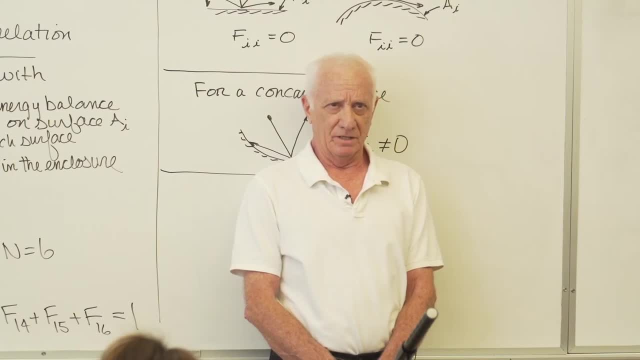 I would guess about 60 to 65 percent probably. Okay, That's a view factor. How about the hall side wall? Look straight ahead. Oh gosh, 10,, 12,, 15 percent, Yeah, View factor. 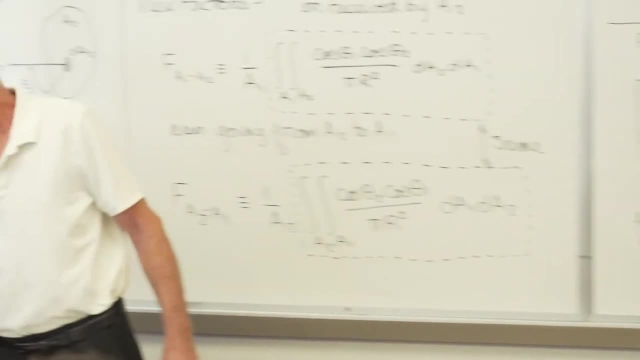 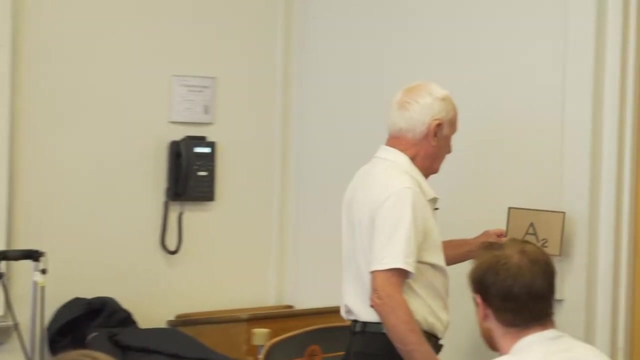 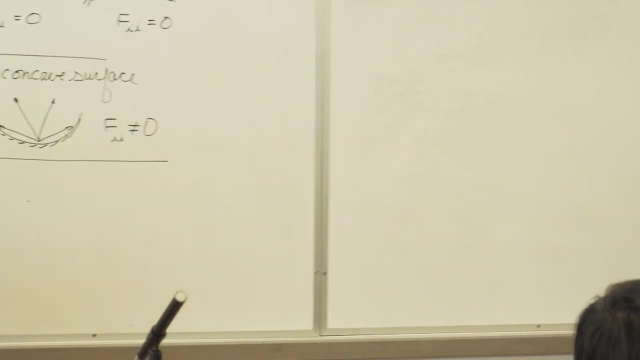 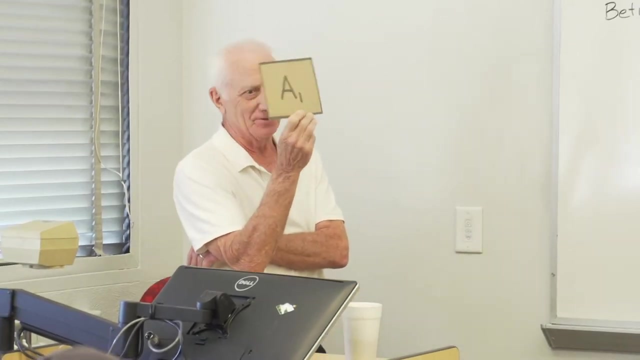 That's what it means in words. So two surfaces, A1 and A2, and I put A2 here. Here's A1.. Let's start way over here. What fraction of energy leaves leaving surface 1 is going to end up reaching surface 2?? 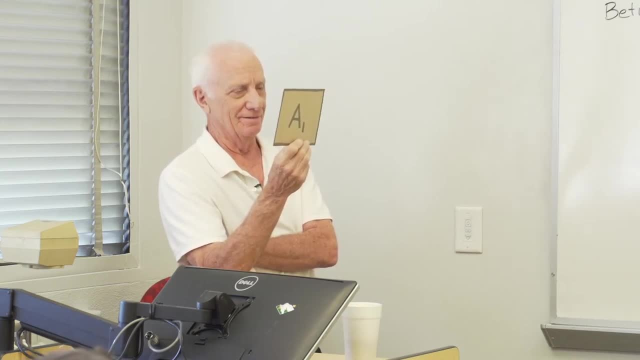 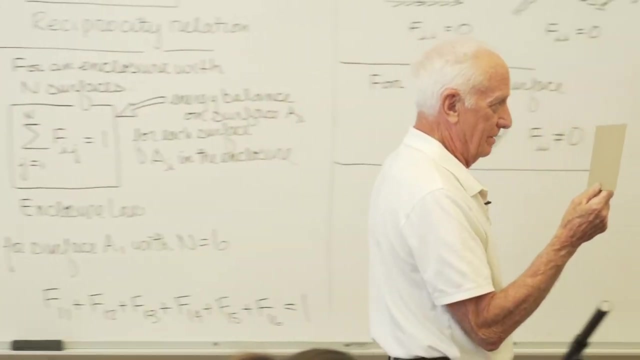 Not much. I'm guessing less than 5 percent. Most of it goes that way and that way and that way and down that way into the clock over there. No less than 5 percent Here, I don't know, Maybe 8-10 percent here. 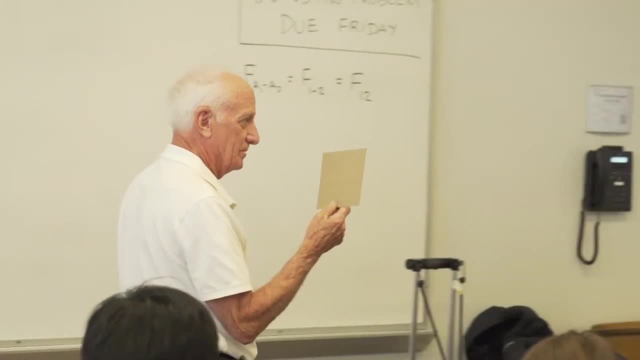 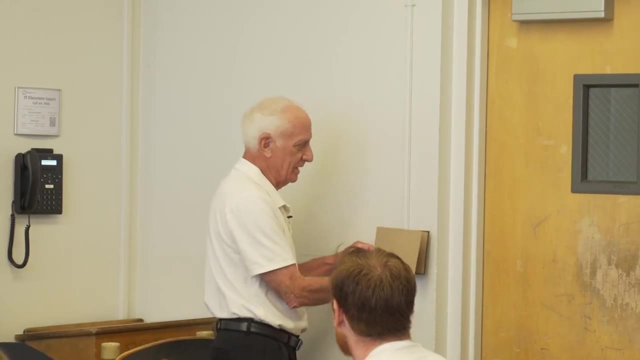 Maybe 20 percent, 30 percent, 40 percent, 50,, 60,, 70,, 80,, 90,, 99 percent, leaving A1 hits A2.. It's called the view factor, These two guys right here. 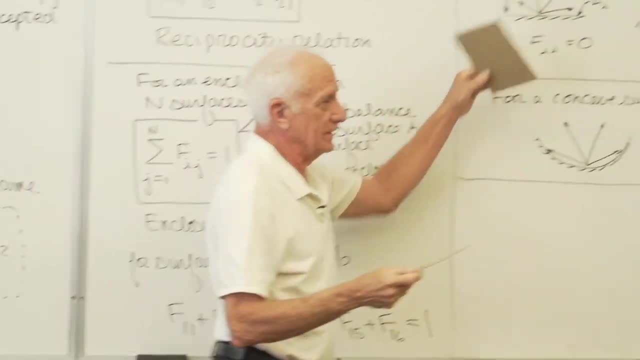 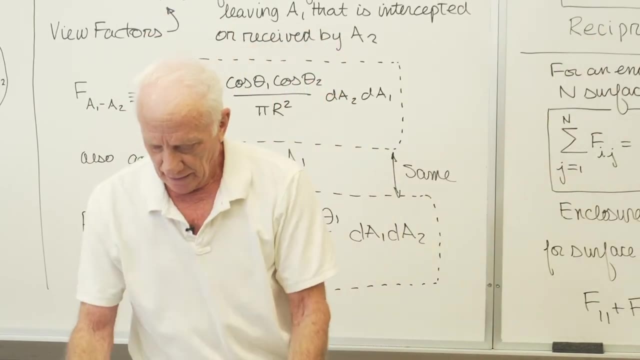 Okay, Let's take this guy right here. a plane surface? Well, let's don't take that, We'll put these up here, These two guys here. How much energy leaving surface 1 ends up directly striking surface 2? I'll give you a big guess on it. 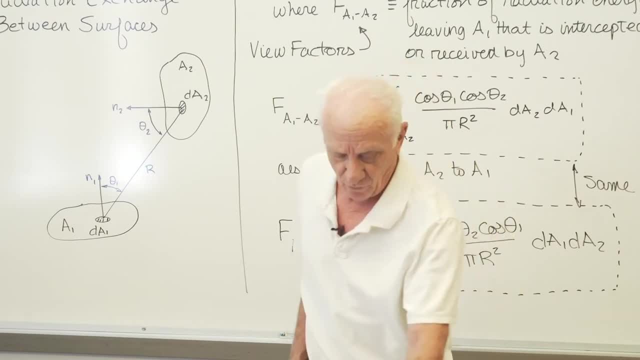 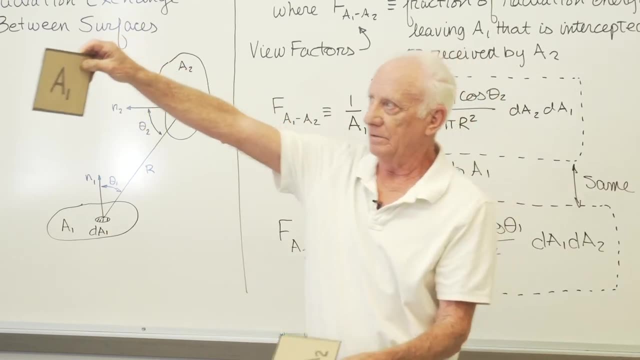 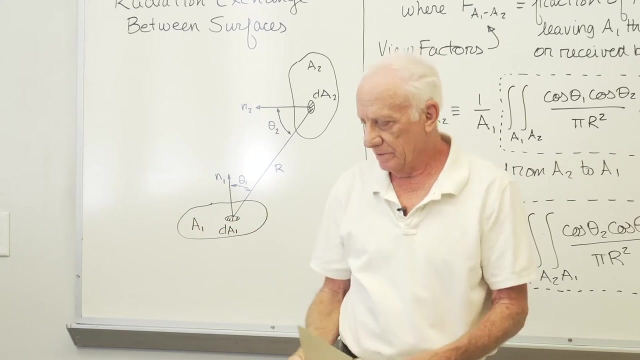 I think 0 percent. You got it Right-o. F1-2 is 0.. So you can have them like this rectangular room. What fraction leaving the window side wall strikes the floor? Okay, 1 is the window wall, 2 is the floor. 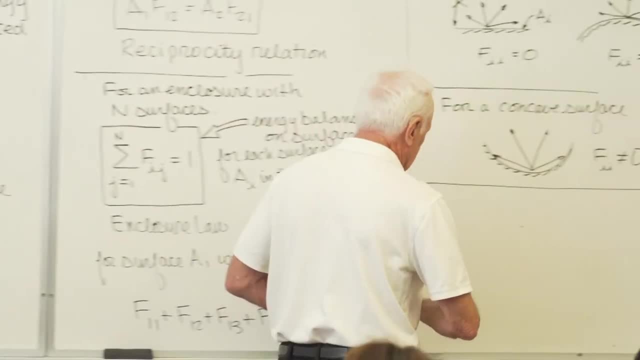 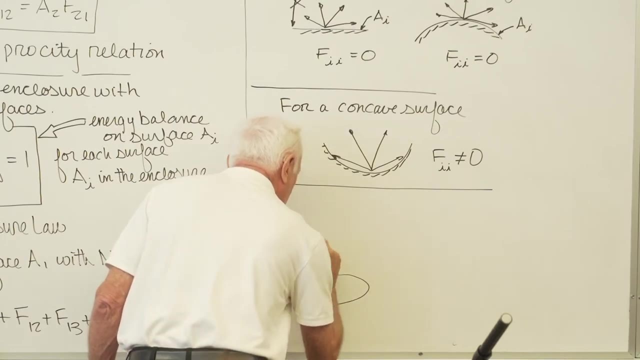 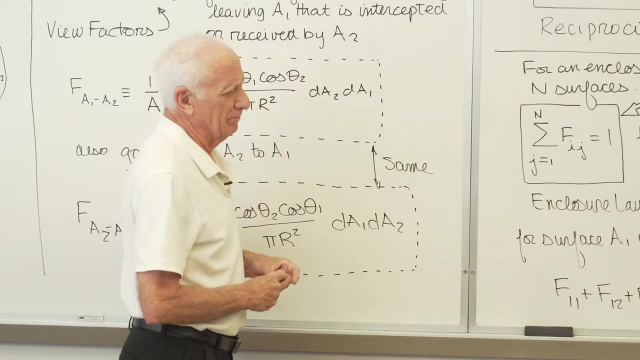 Okay, Let's take a simple example. Let's take a circular area, call it A1, and the hemisphere above it, call it A2.. A1,, A2.. Now we'll just take the general problem. Find all the view factors. 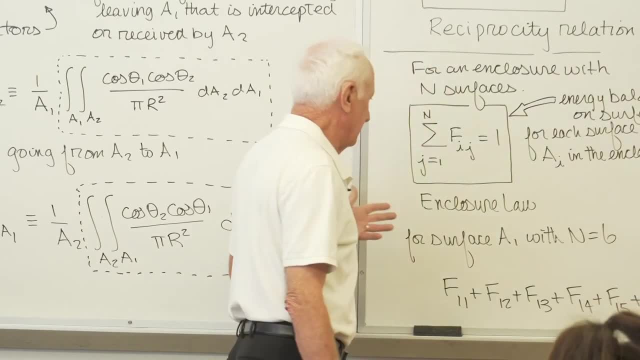 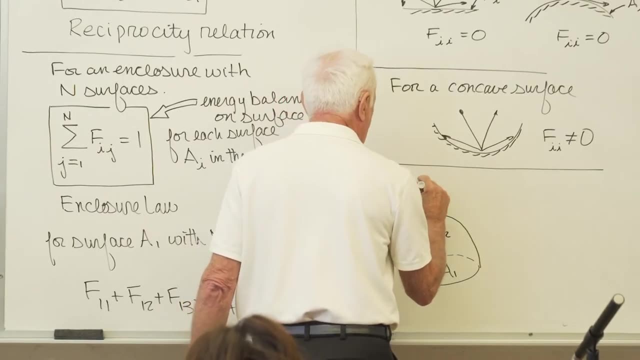 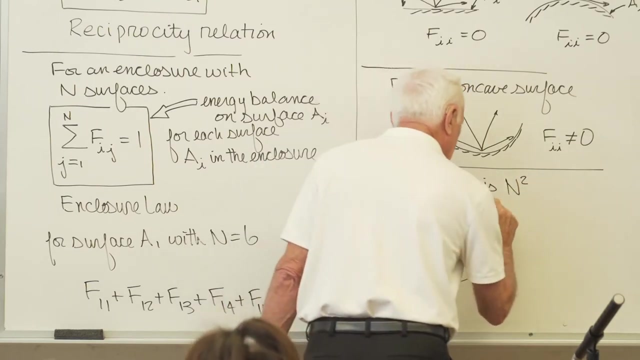 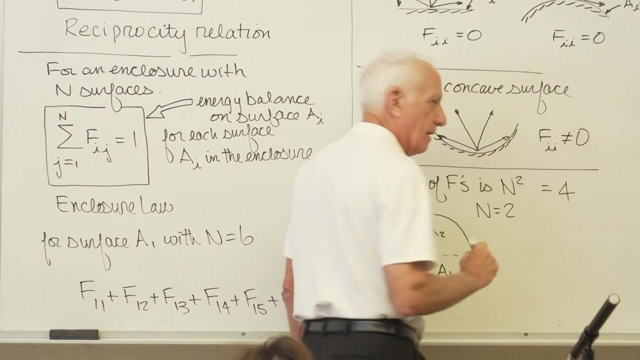 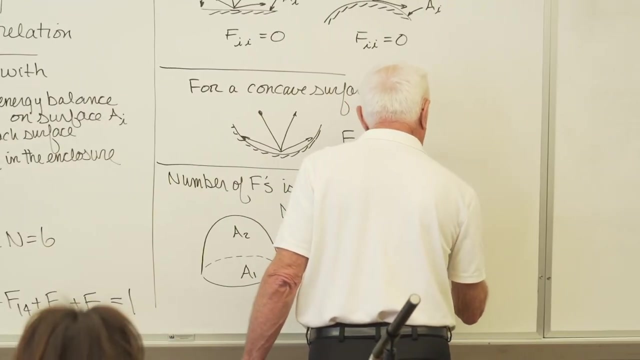 What does that mean? Well, there's two surfaces, So number of view factors N squared. For this problem, how many surfaces are there Two? Number of view factors 2 squared 4.. Sometimes it helps to write them in a matrix format. 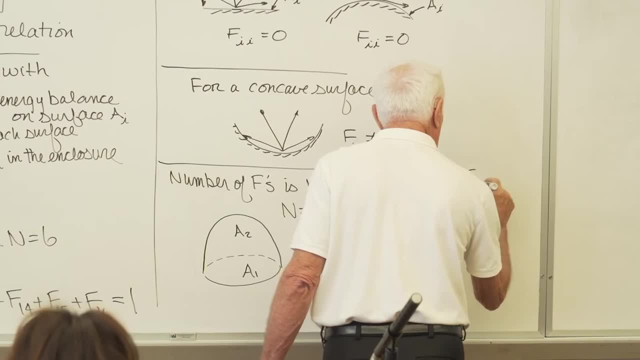 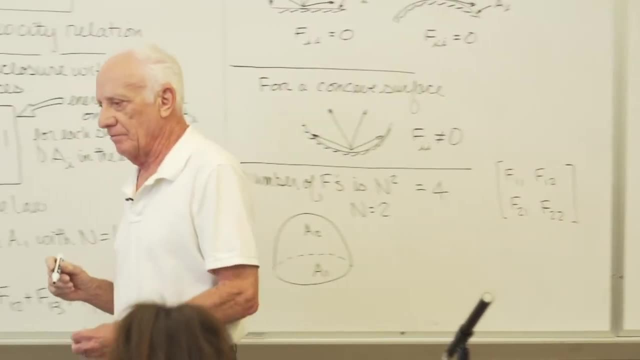 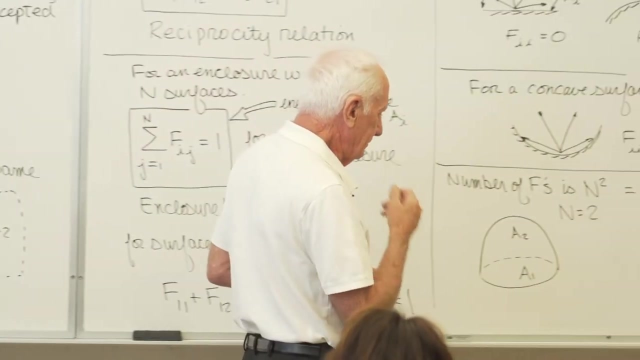 What are they? F1, 1.. F1, 2.. F2, 1. F2, 2.. So the problem said: find all the view factors. there they are. Let's do the easy one first. 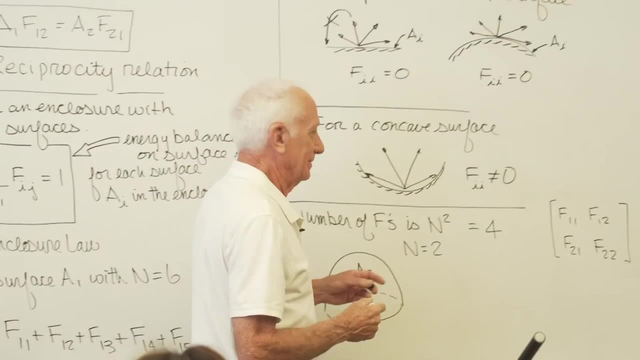 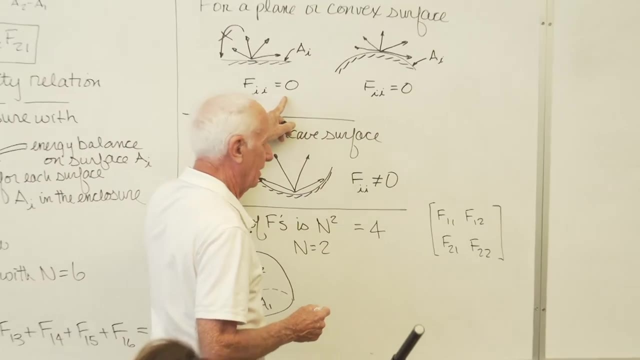 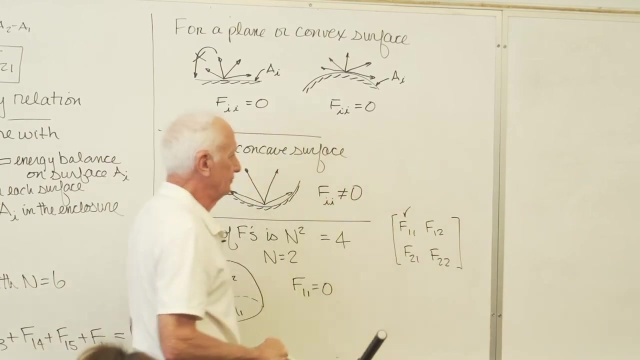 Do I see any plane surfaces? Oh yeah, Surface 1.. If I see a plane surface, FII is 0.. F11 is 0.. Check mark got it. I'll do another easy one: What fraction of energy leaving? 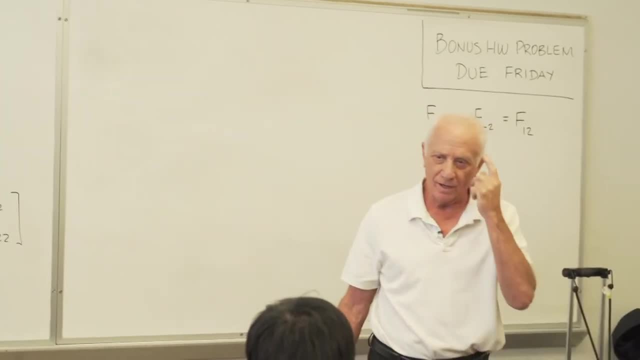 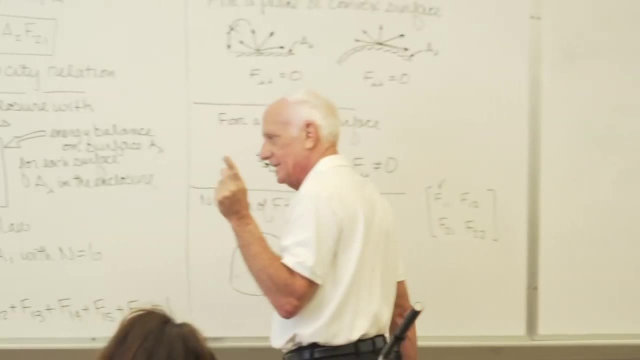 surface A1, do you think ends up reaching surface A2?? My best guess is 100 percent. Right By observation. no equations, no graphs, no tables. you see it, F1 to 2, or, if you don't want to do it that way, 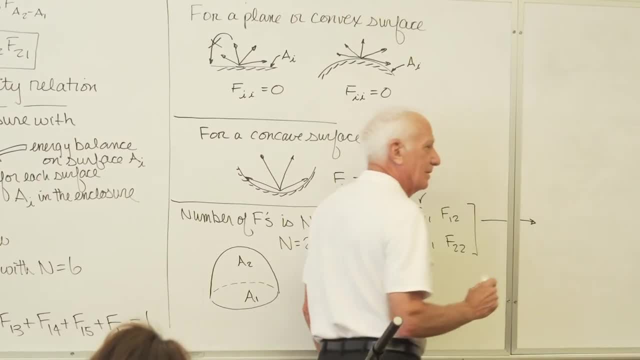 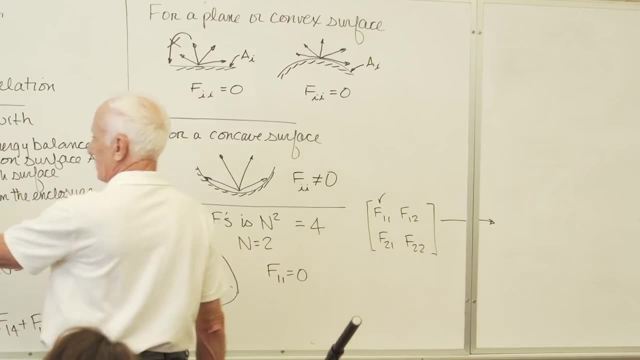 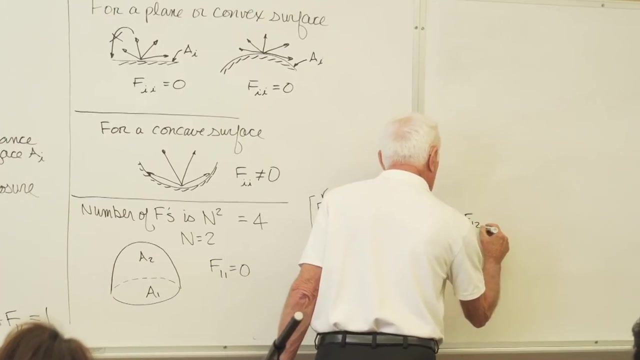 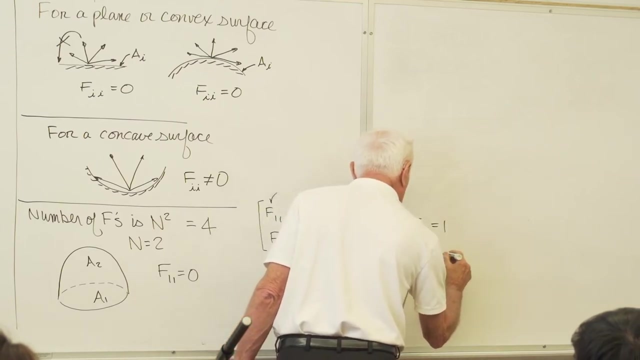 is that an enclosure? Yes, it's an enclosure. What does that mean? That means every row in that matrix, every row when you add them together, equals 1.. So F11 plus F12 equal 1.. For this row, F21 plus F22 equal 1.. 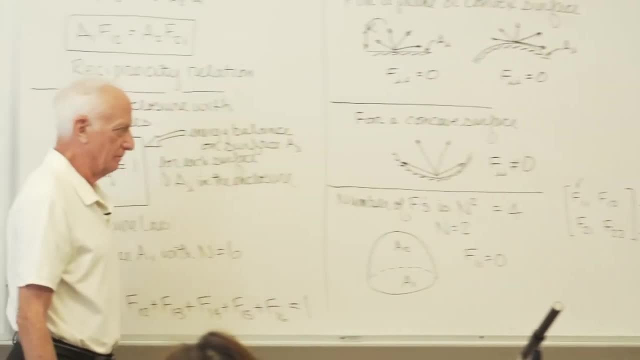 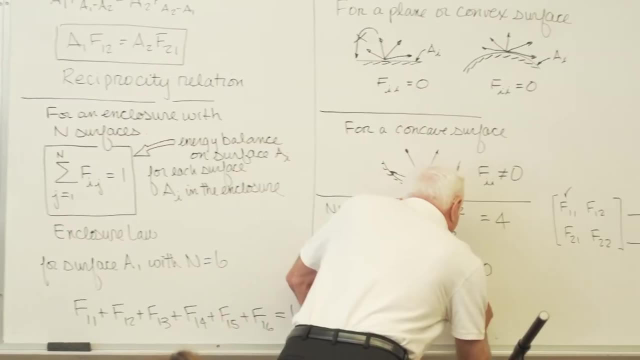 Every row you can write the enclosure law. So either you see it directly- oh, I see it, it's 100 percent. F12 is 1.. Or if you don't see it immediately, then you say I'm going to write. 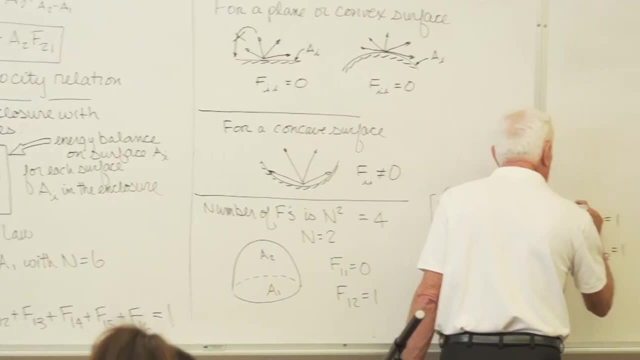 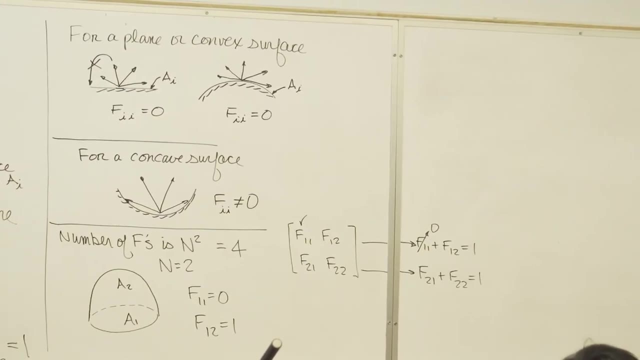 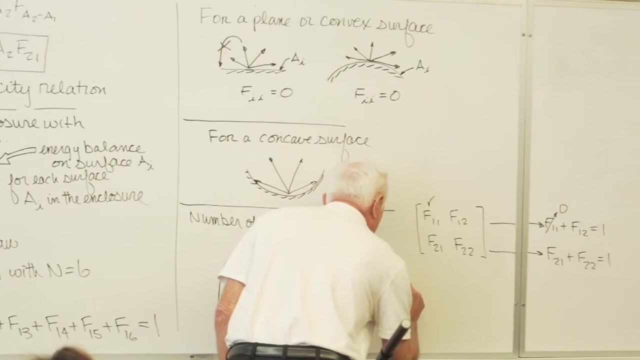 the enclosure law for this row. What's F11?? I just said 0, plane surface. So what does that mean? F12 is 1.. F21, oh, right there, right there, Reciprocity: F21, A1 over A2, F12.. 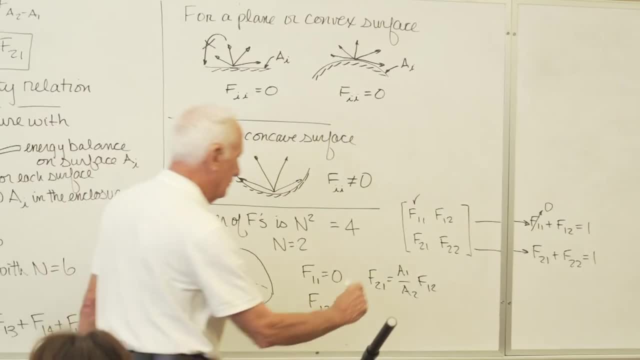 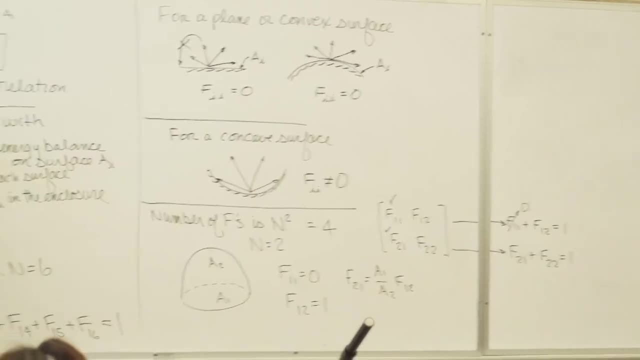 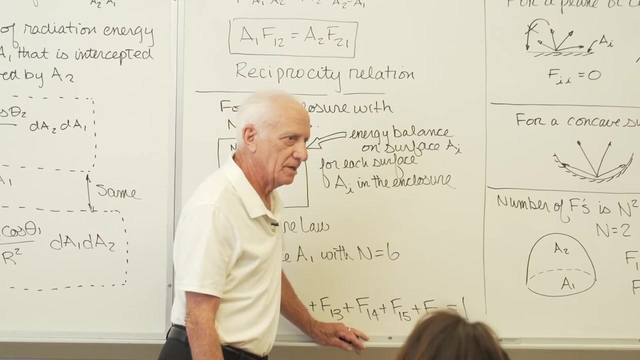 F12 is 1.. I got it F21.. What's A1? Pi R squared Pi D squared divided by 4.. What's A2? Half of a sphere, area of a sphere. Pi D squared A2, Pi D squared divided by 2.. 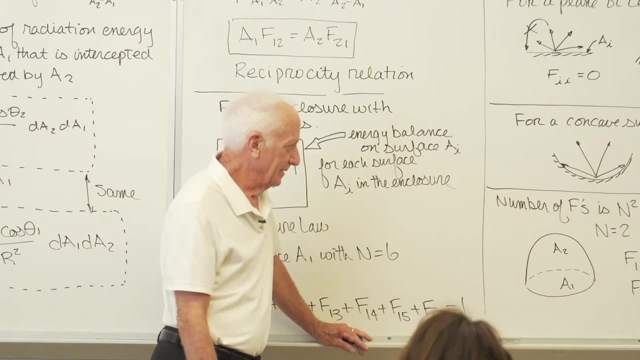 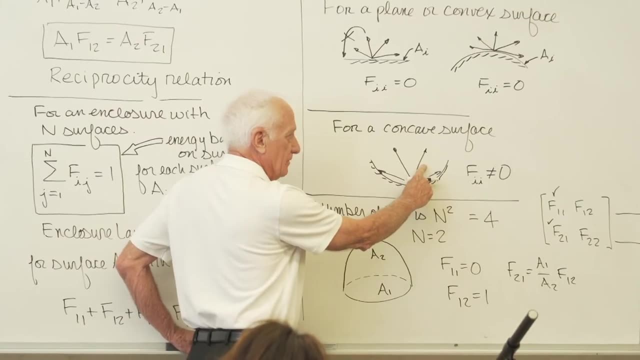 You got it. The Pi's cancel out, and so on and so forth. Once I got F21, how do I get F22?? Well, here's one thing: That's a concave surface. F22 is not 0.. If you want to prove it, 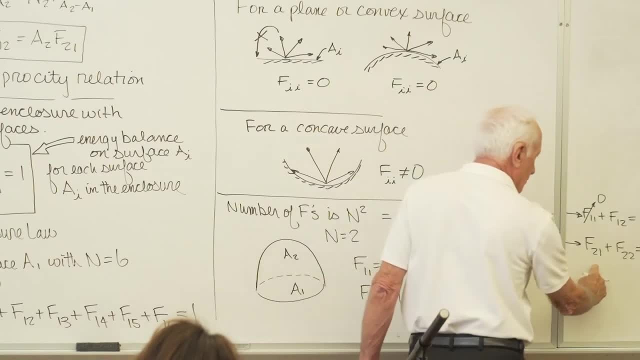 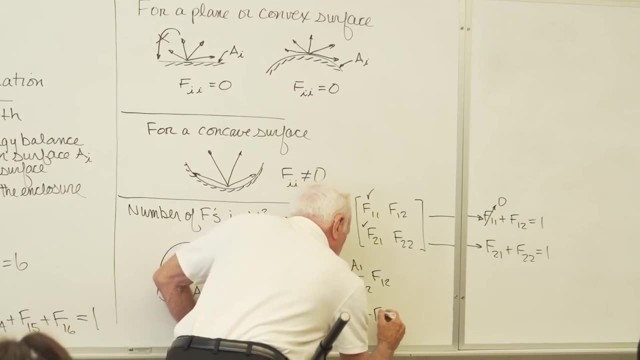 go over here. second row: F21 plus F22 equal 1.. So F22 equal 1 minus F21.. I know F21, I just found it. I put F21 in there and I've got F22.. Okay, I've got all four. 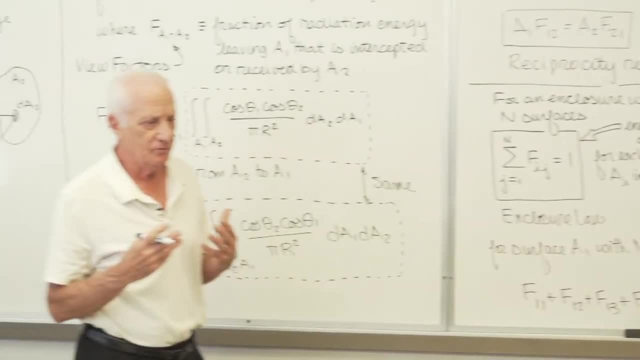 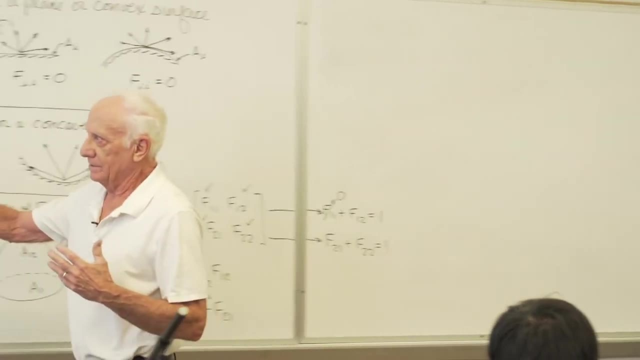 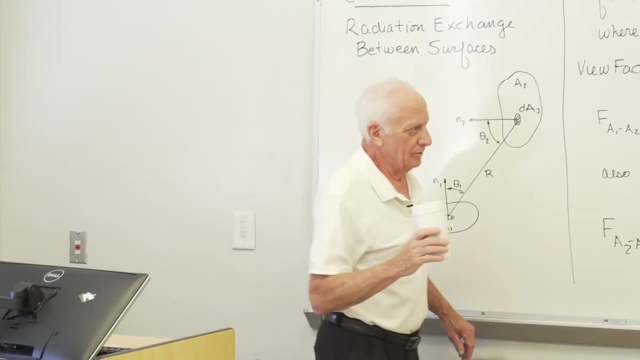 That kind of exercise is called view factor algebra, Because all we're doing is we're solving algebraic equations. We're not going back and solving this big, horrendous double integral equation- No, not in this class- But we are using view factor algebra. 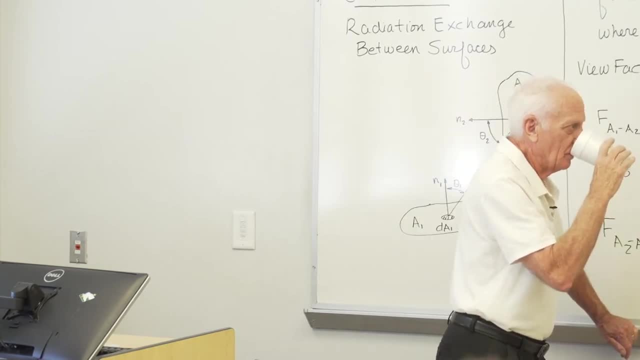 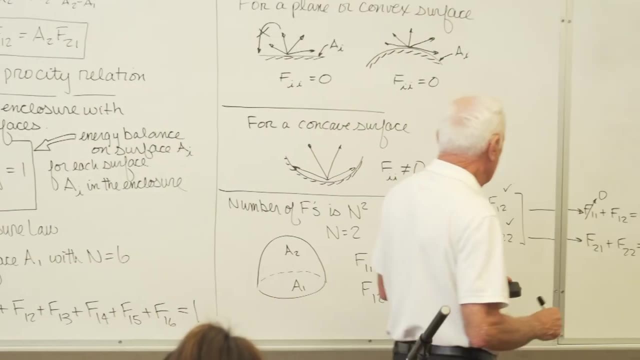 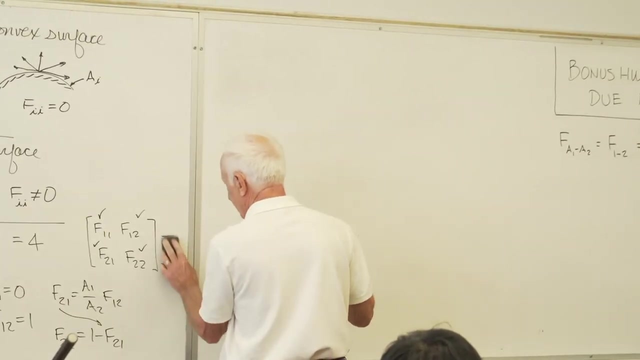 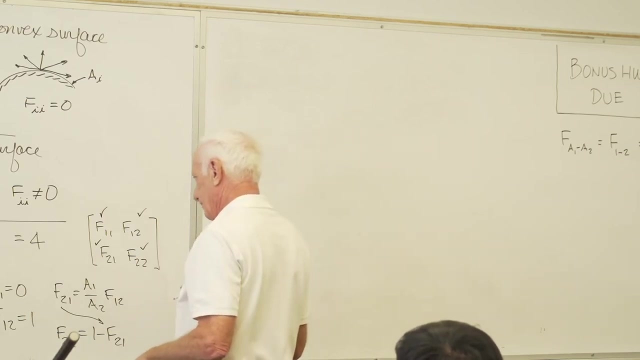 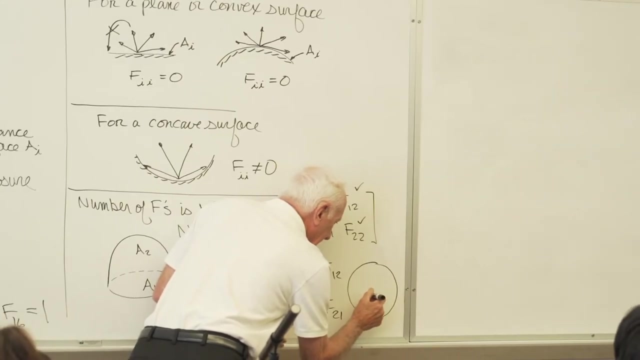 to solve for the view factors. Okay, Let's take another one. Let's take that same, I'll do this one, that's okay, I'll put it here. So this is a big sphere and a little sphere, two spheres. 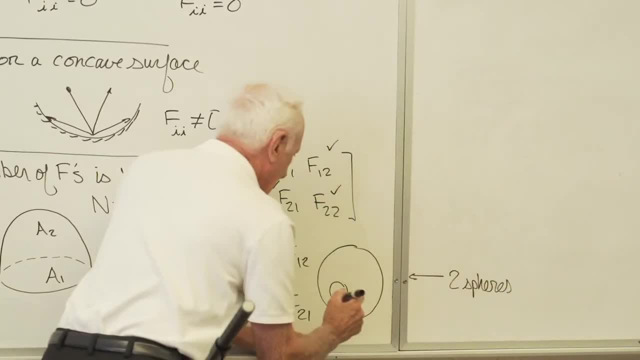 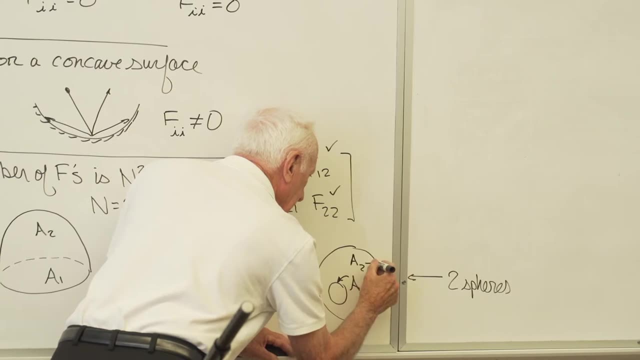 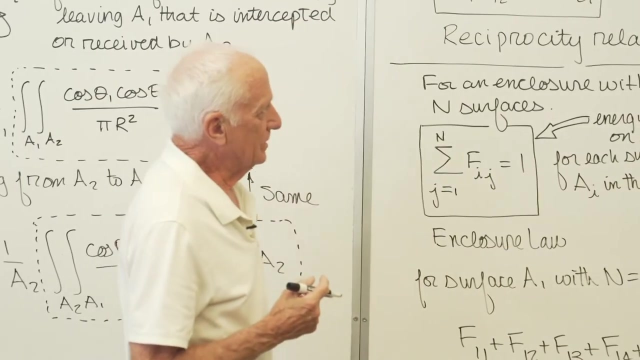 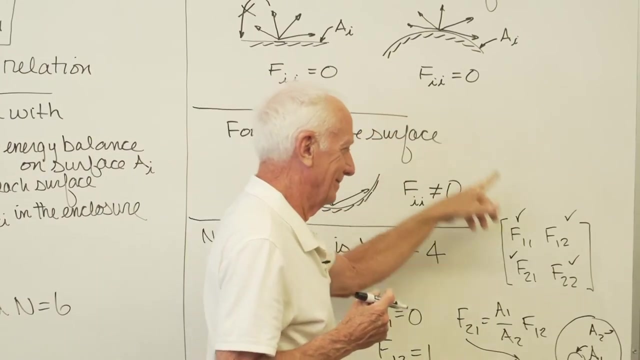 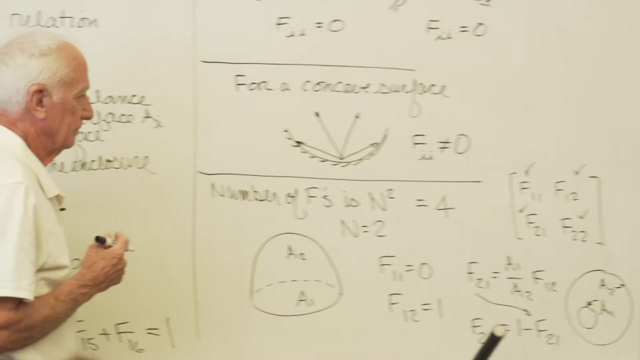 Call this guy A1 and call the big sphere A2.. Is that an enclosure? Yes. Do I see any plane surfaces? No. Do I see any convex surfaces? Yes, F11 is 0.. Got it If F11 is 0,. 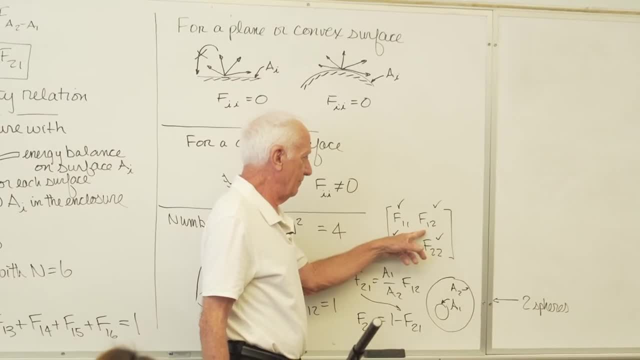 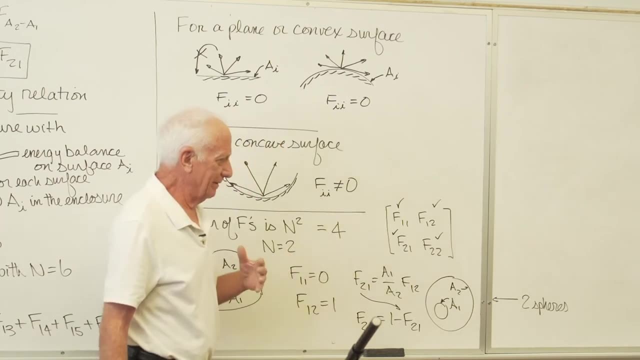 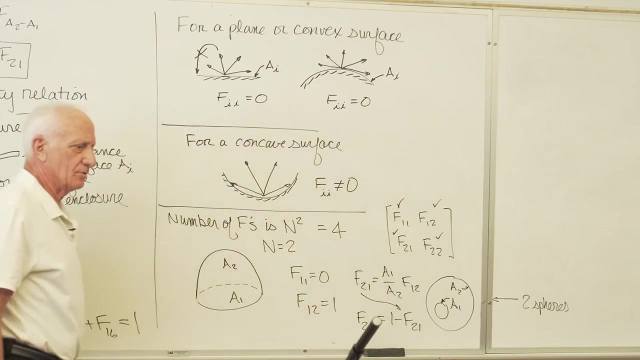 can I look at this and see what F12 is? Yeah, F11 plus F12 equal 1.. So I can say: it's obvious to me. I see what F12 is. All the energy leaving the small sphere ends up directly hitting the big sphere. 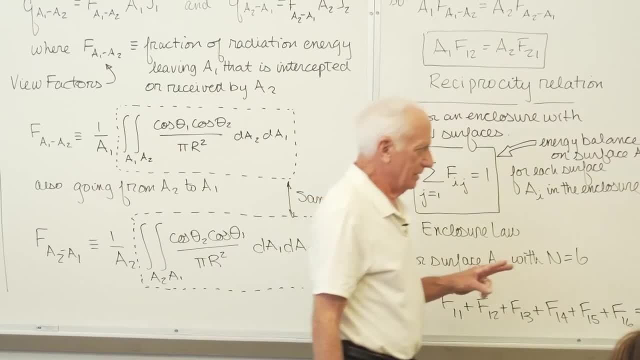 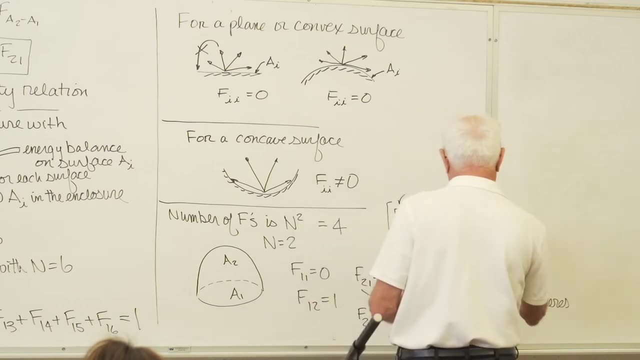 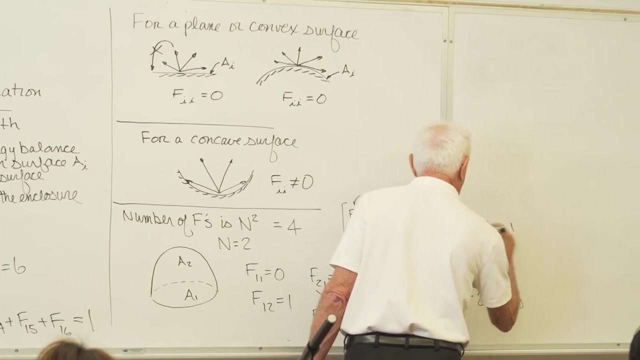 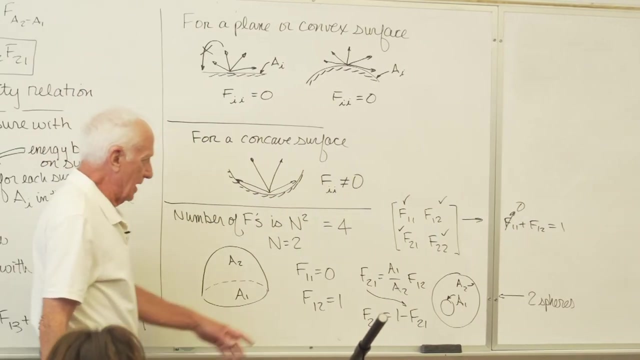 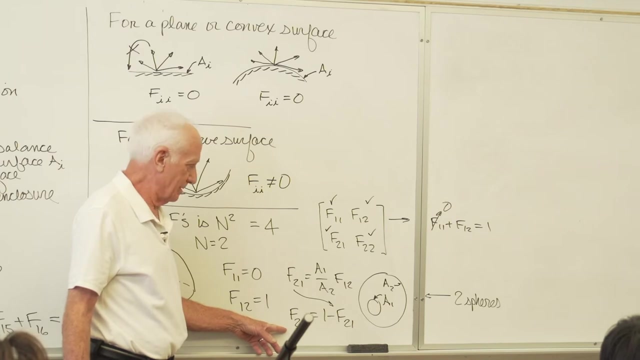 Right, Two ways of doing it. Just say: I see it, it's obvious. Or you say I use this equation: F11 is 0. Got it? I want F21.. There's the equation. I want F22.. There's the equation. 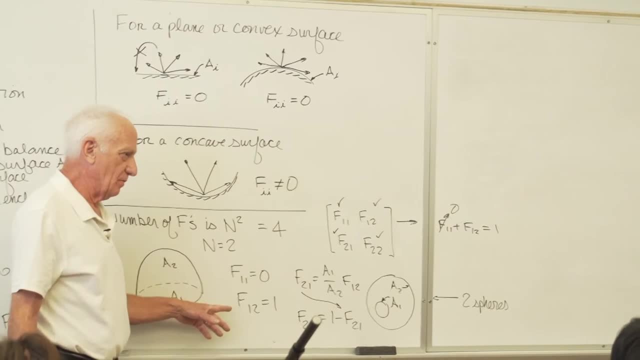 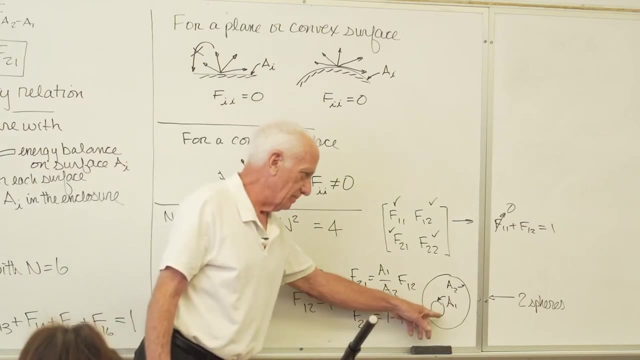 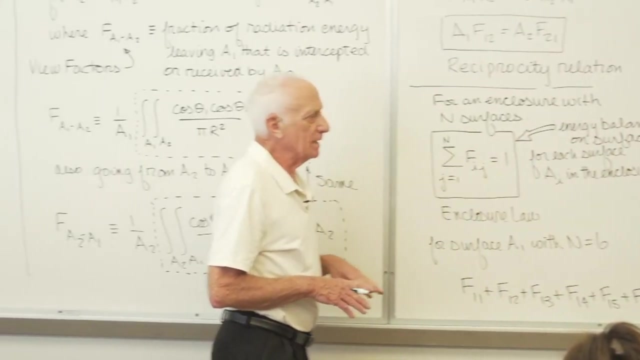 I use the same equations. whether I'm solving this problem- the hemisphere- or this problem- big sphere, small sphere- I use the same equations. The solution technique is the same. The numbers are slightly different because the areas are different: A2, hemisphere. 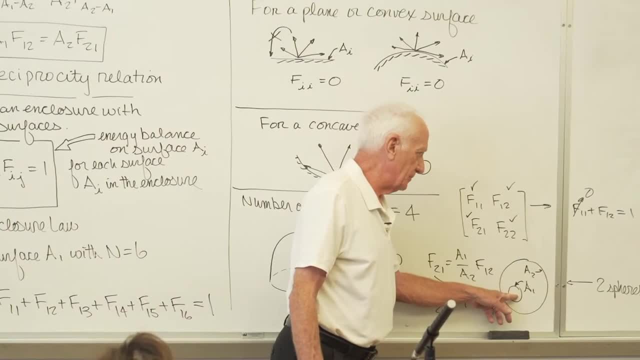 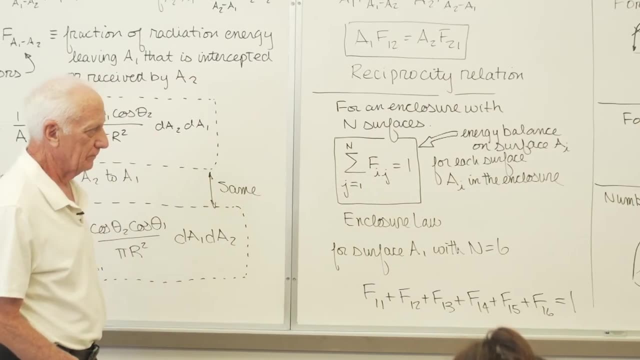 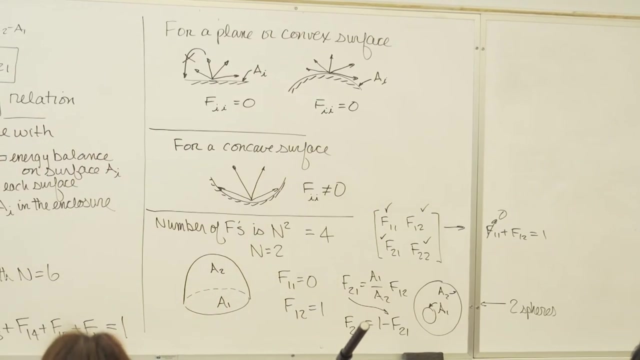 A1, circle A1, area of a small sphere. A2, area of the big sphere: Pi d small square, Pi d big square. So two pictures, but they both are solved the same way. By the way, I didn't put this on the board. 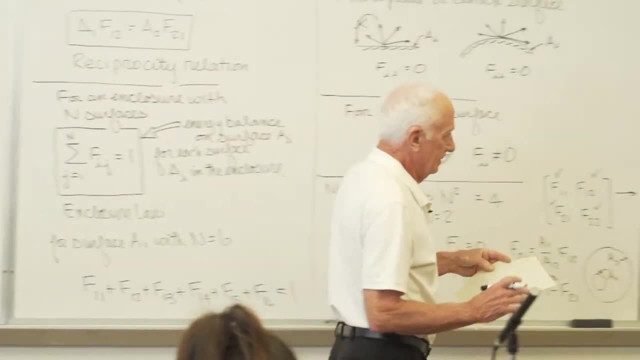 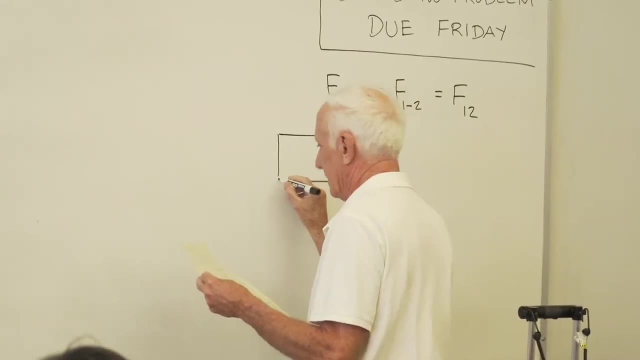 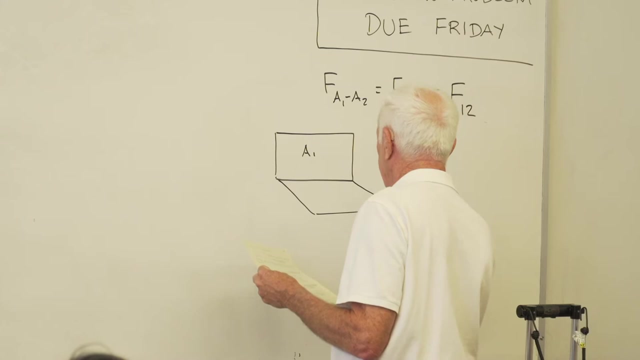 I think probably I should. I'll do it now. This might be useful too sometimes. Let's say, we had this area A1, and then this is at a right angle. here This is an area. we'll just say it's at a right angle. 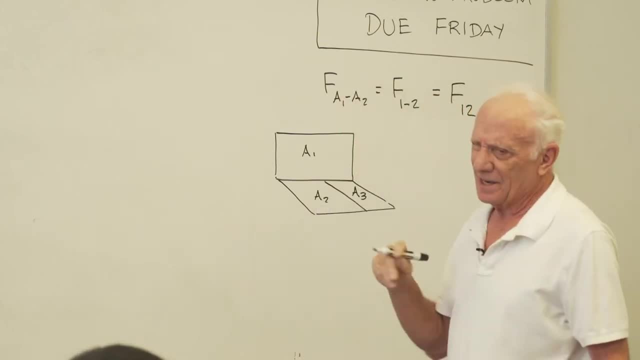 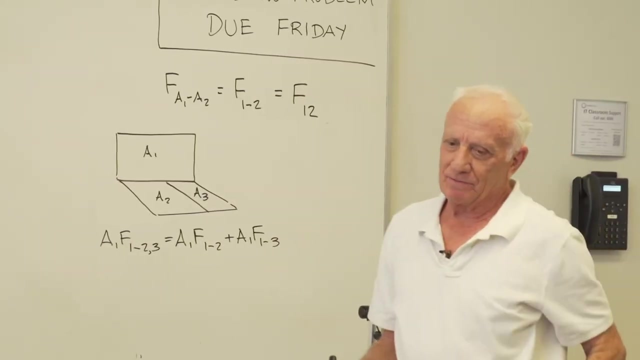 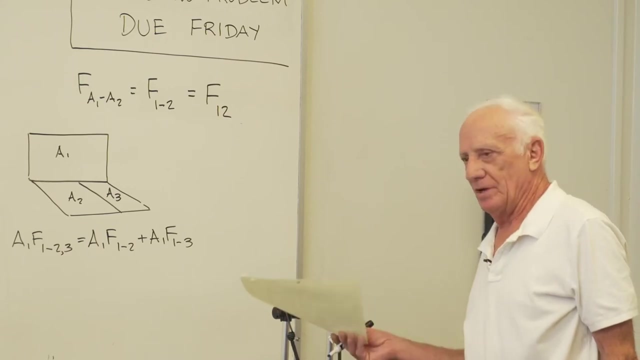 A2, A3.. It's not an enclosure, obviously. They're all plain surfaces, obviously. So here's what we can write down: A1,, F1-2, 3.. Now the subscripts get a little more complicated. By the way, you can see that the A1s will cancel out. 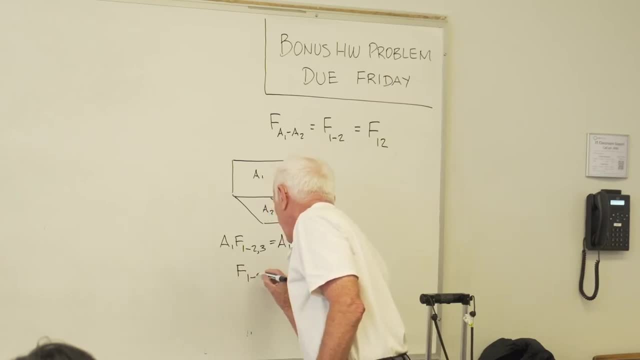 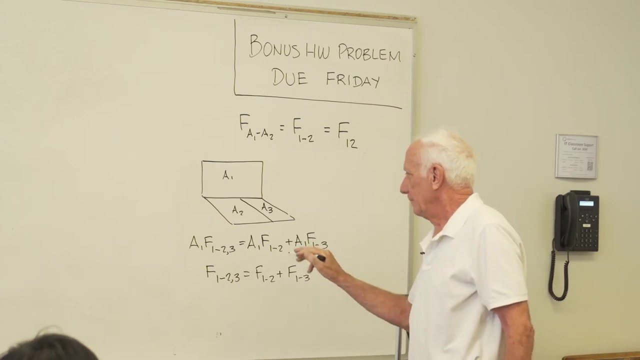 So if you want to write it in shorthand notation, But let's take the top equation, So that's right. Here's what it says in words: The fraction of energy leaving surface 1, that goes to combine surfaces 2 and 3,. 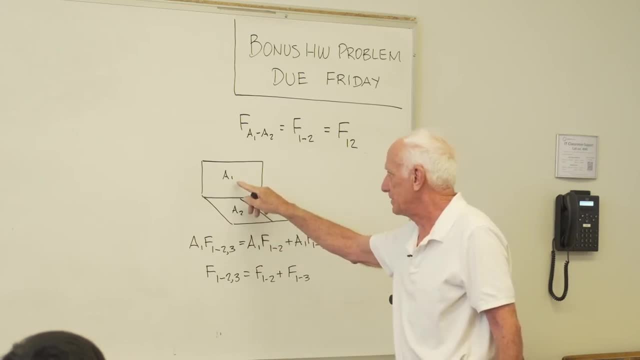 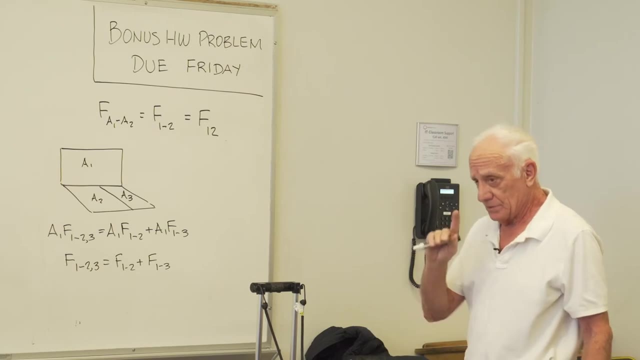 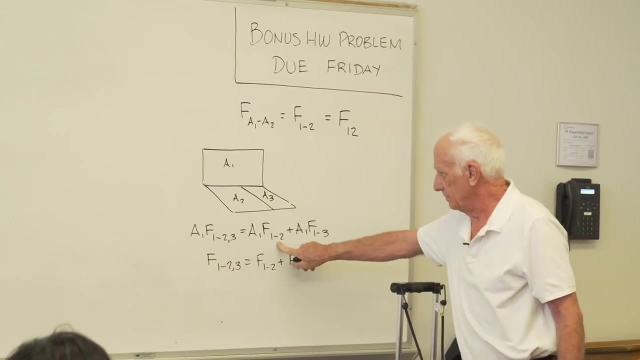 equals the fraction leaving 1 that goes to 2, plus the fraction leaving 1 that goes to 3.. So it makes sense. But the subscripts have a meaning. Here's what they mean. The dash means goes to, So F1-2.. 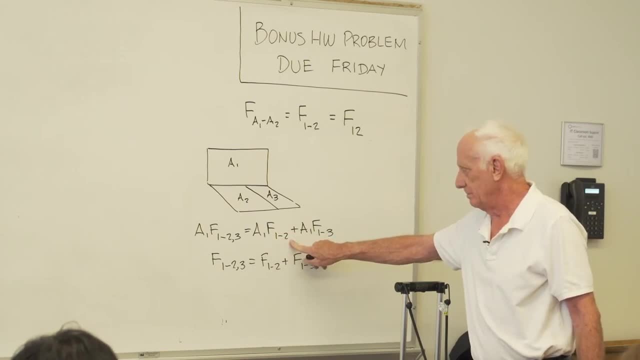 The fraction going from A1 to A2.. Dash means 2.. Comma means and The fraction going from A1 to A2 and A3. That's what the comma means. That's how you say it in words. Fraction of energy leaving surface A1, that goes to combine surfaces. 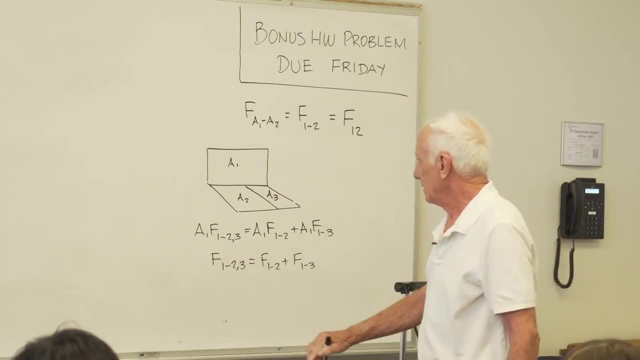 2 and A3.. Now how about the backward one? A2, A3 to 1.. So A2, 3 times a fraction from 2, 3 going to A1. Fraction 2, that was A2.. 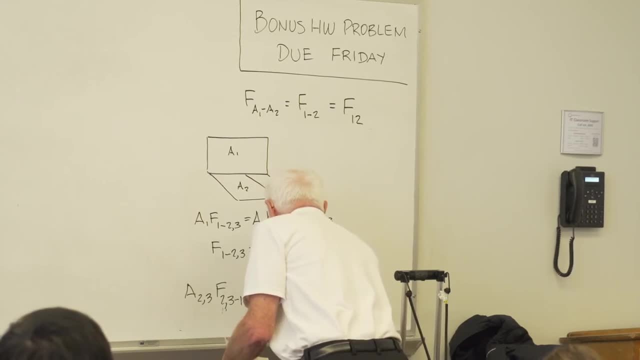 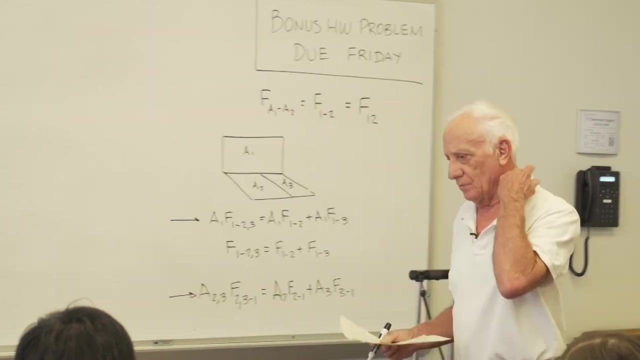 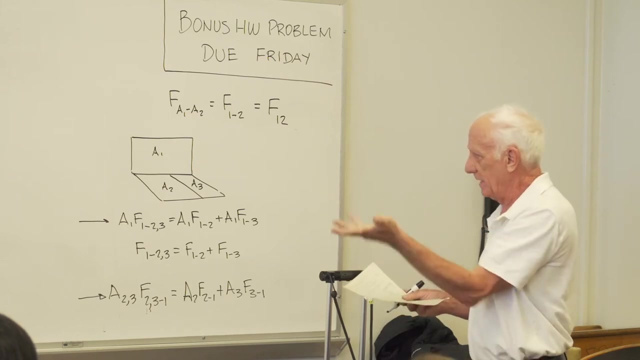 Fraction 2 to 1, plus A3.. Fraction 3 to 1.. So that's going one direction, leaving one going down. Other direction: leaving combined surface 2 and 3, going up to A1. So I think you might need that for one of the homework problems. 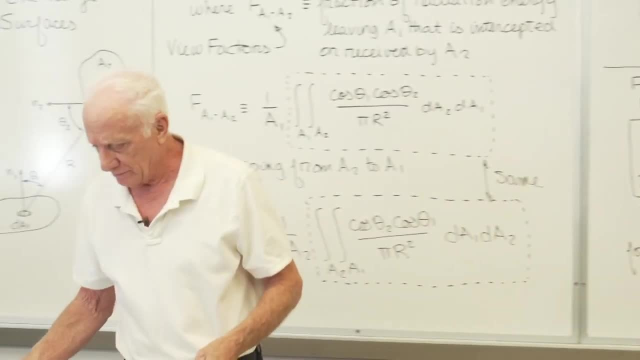 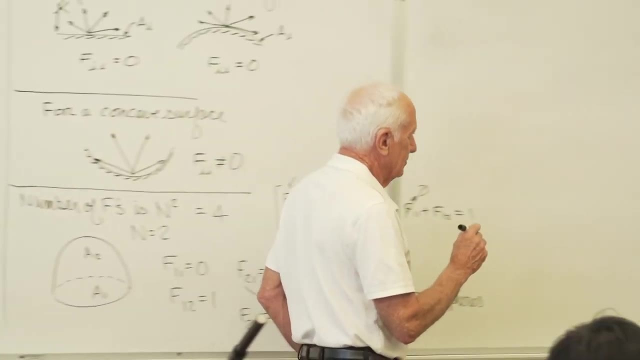 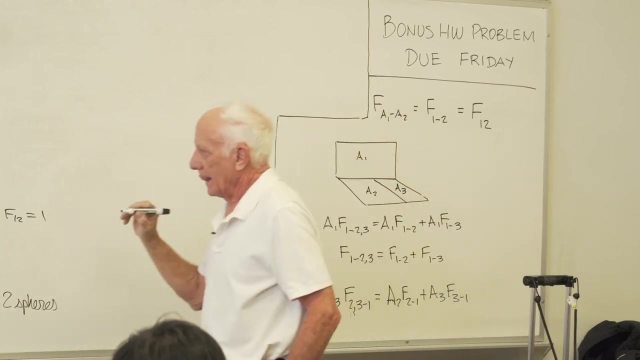 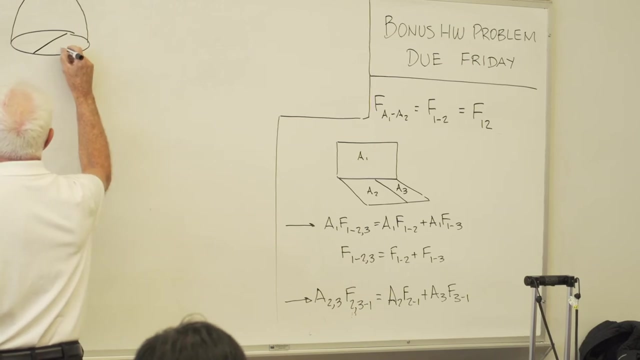 So just keep that in mind. That's why I put that on the board now. Okay, Let's go back and look at another one. Let's take this guy here and break him down. some more Diameter through the center: A1, A2, A3.. 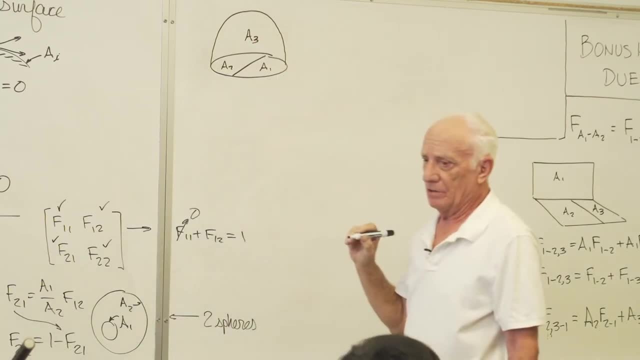 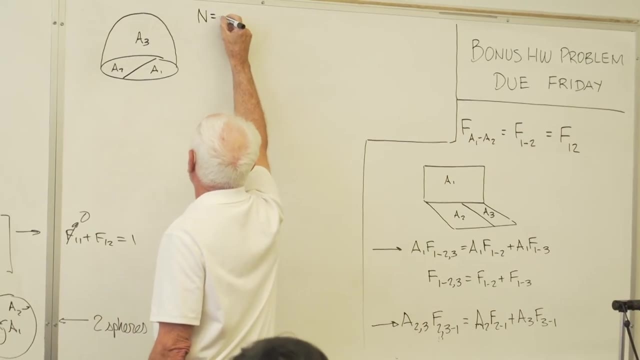 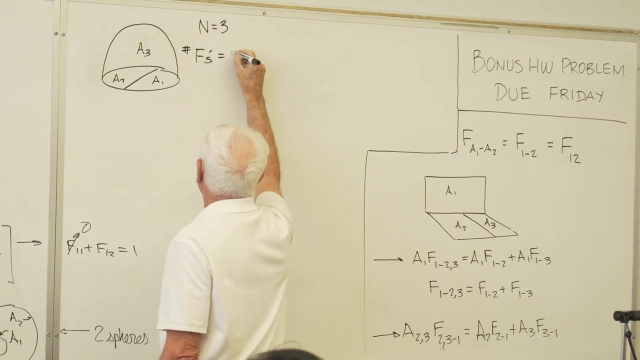 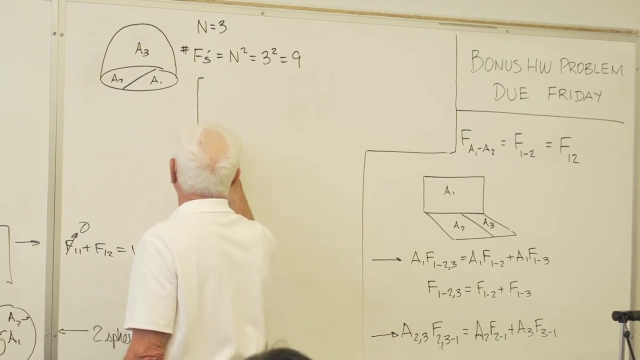 Okay. Is it an enclosure? Yes, it's an enclosure. How many surfaces? Three N equal three. How many view factors F? Number of Fs? N squared three, squared nine. Show them Okay: F11,, F12,, F13.. 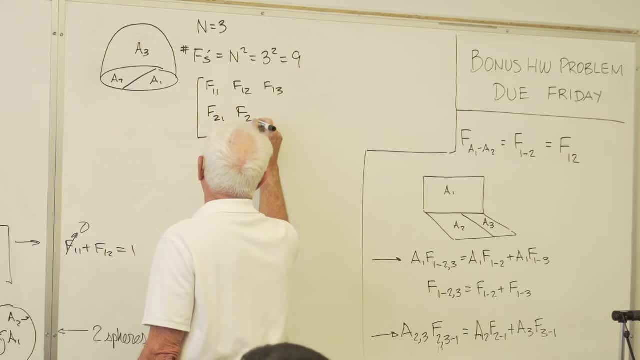 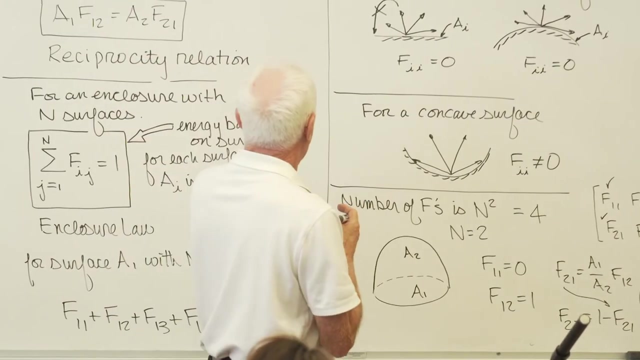 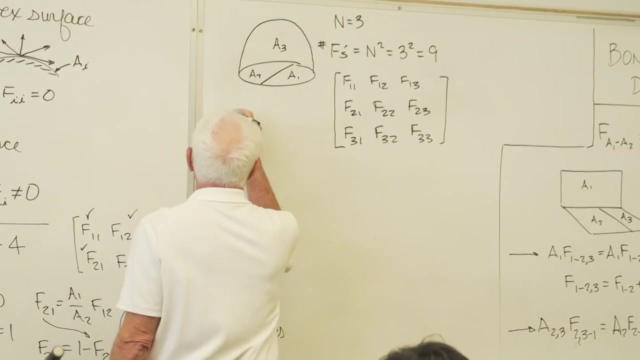 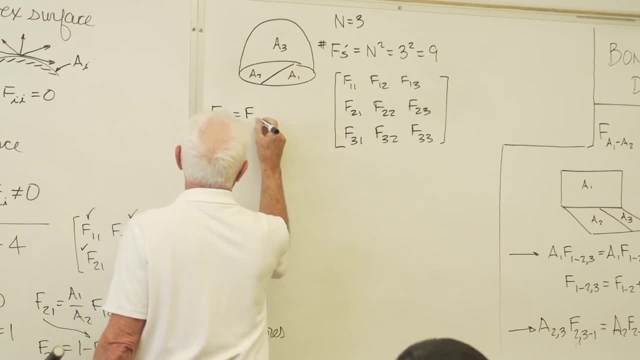 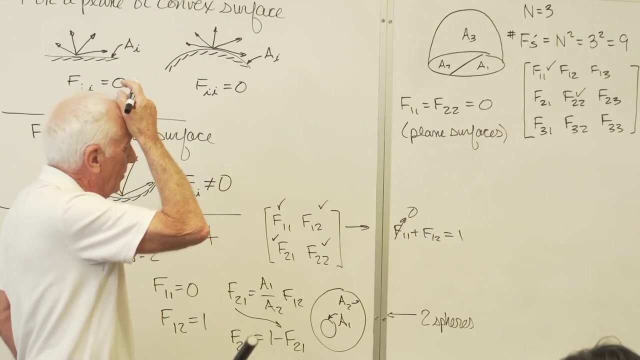 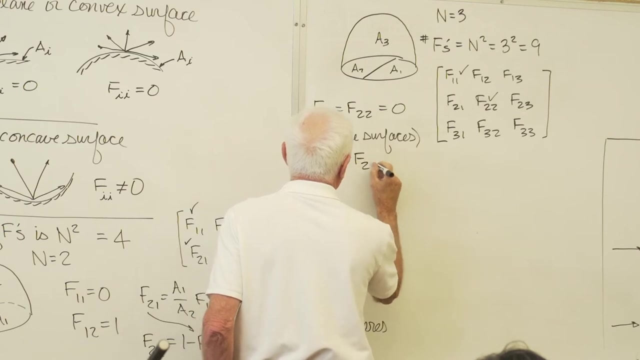 F1,1 equal F2,2 equals zero plane surfaces. Check them off. 1,1,2,2, got them. What else can I see? Obviously, I know that F1,2, equal F2,1 equals zero. 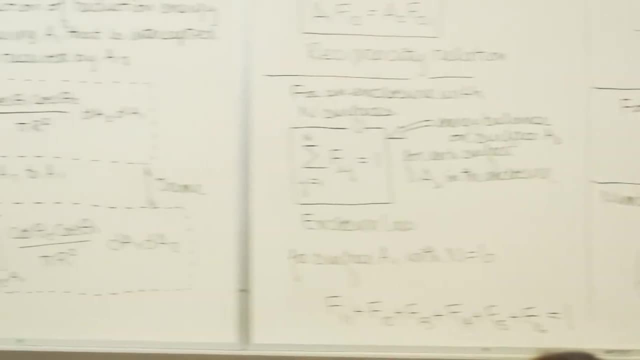 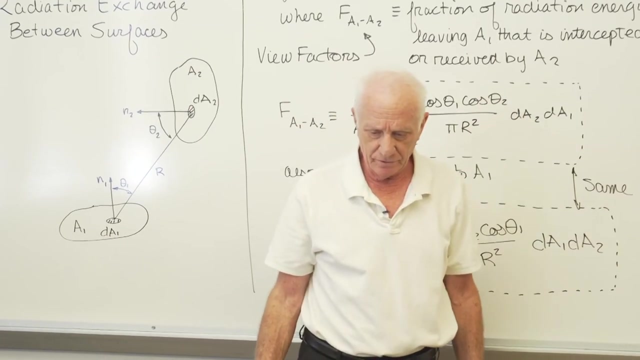 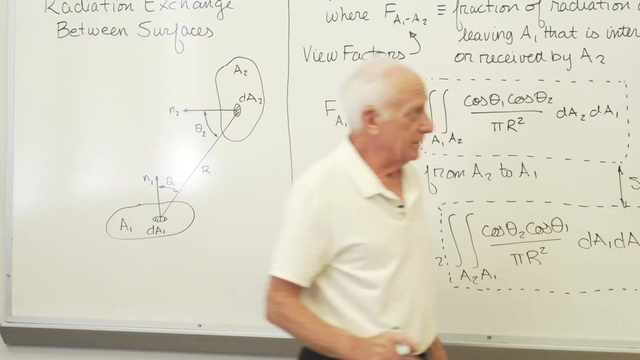 I just said that They're both on the same plane. here they are. Put them down on the table. What's F1,2? Zero? What's F2,1? Zero? So you can say that I see that immediately. 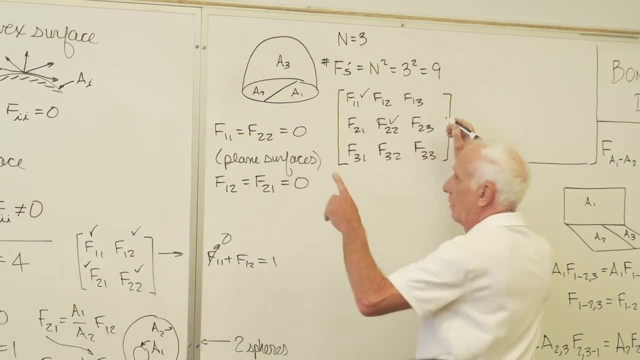 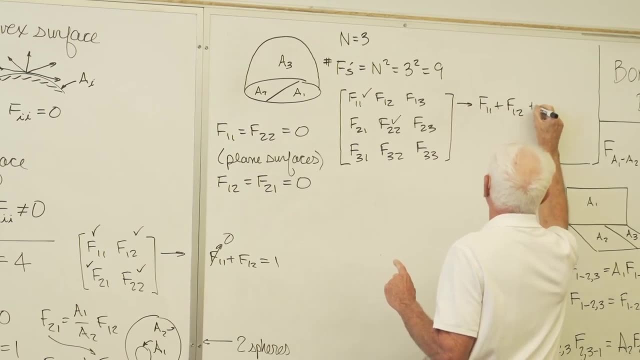 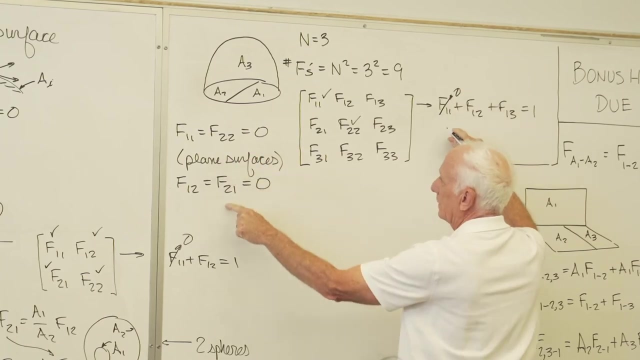 You can do it one of two ways. Every row it's an enclosure. every row you can write: F1,1 plus F1,2 plus F1,3 equal 1.. F1,1, zero. F1,2, zero. 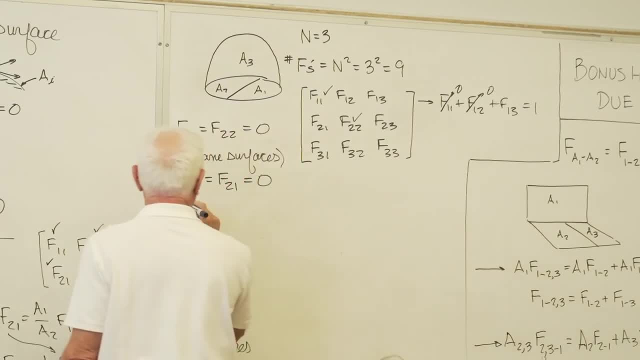 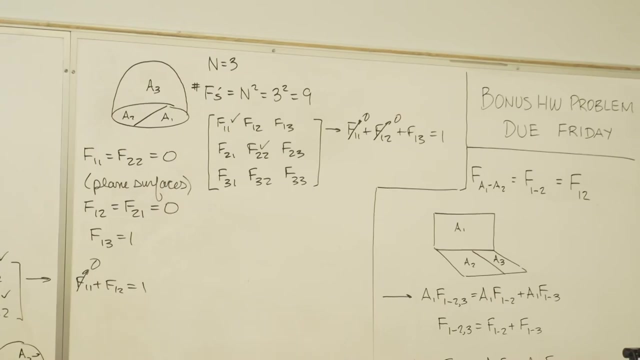 I get it. F1,3 is one. Well, of course I didn't need to do that over there. I can see it's obvious to me: all the energy leaving surface 1 ends up striking surface 3.. It has to. 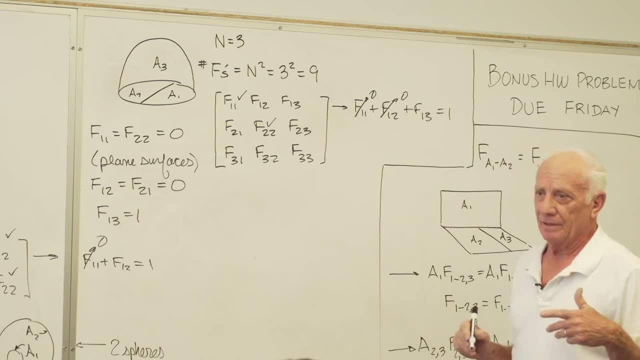 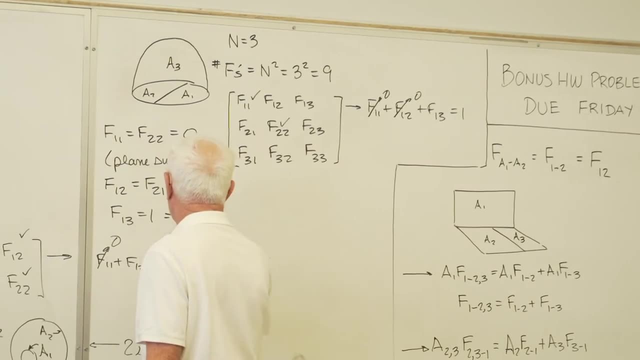 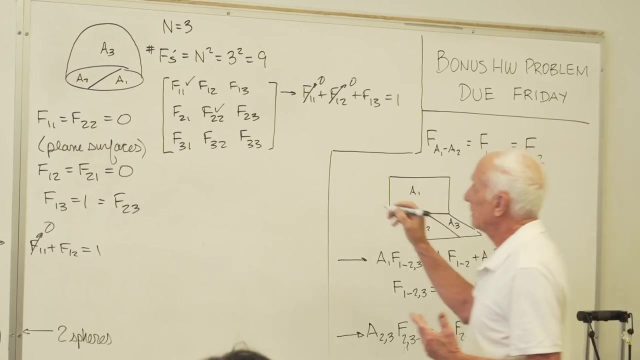 All the energy leaving surface 2, guess what it hits Surface 3, F2,3 is also 1.. How do I know that? By observation, I see it. Or if you want to prove it, go ahead and prove it. 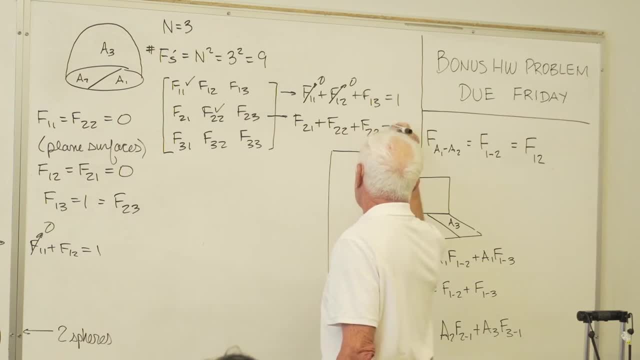 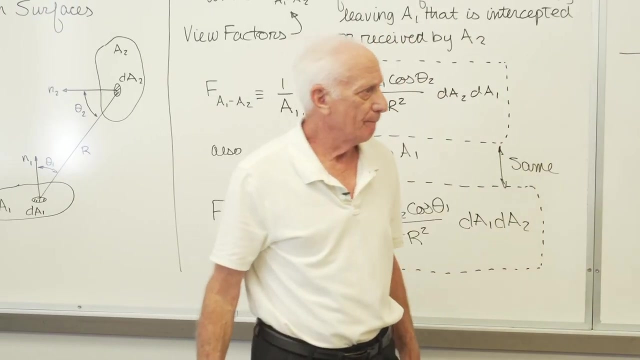 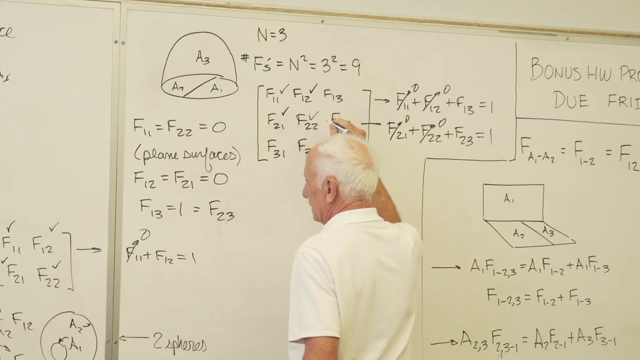 F2,1,0,, F2,2,0,. yeah, F2,3 is 1.. If you don't see it by observation, use the enclosure law. for the second row, Check marks 2,1,1,2,2,1.. 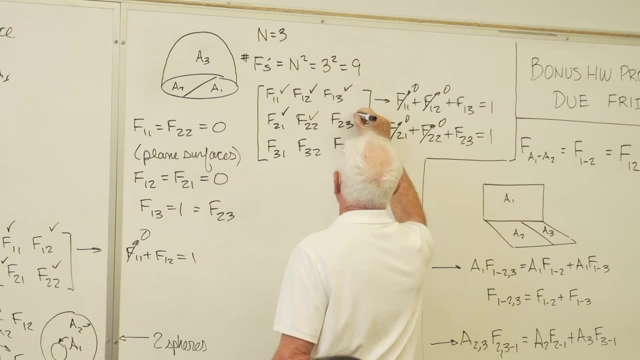 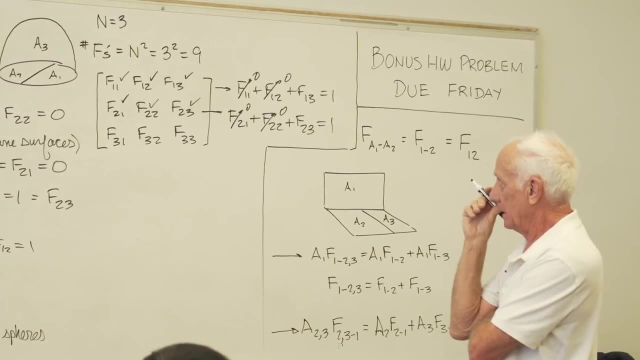 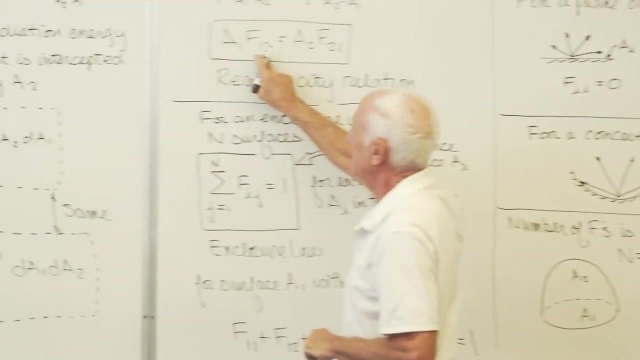 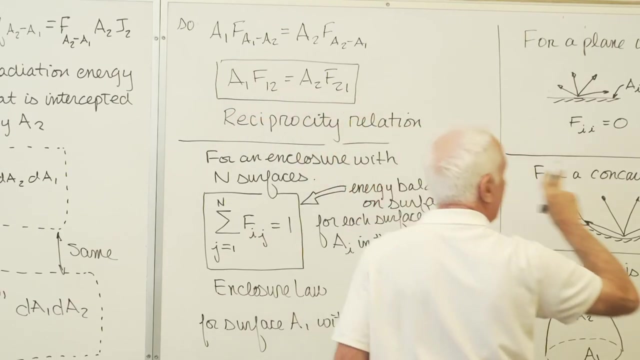 What else do I have? 3,1,3,2,3,. I got the six of the nine. Three to one A3,. F3,1 equal A1,F1,3.. Yeah, Okay, I got it. 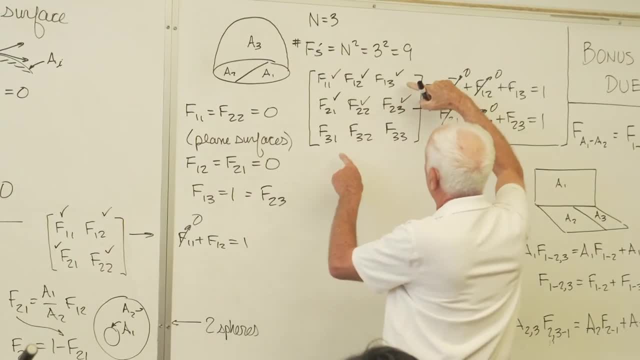 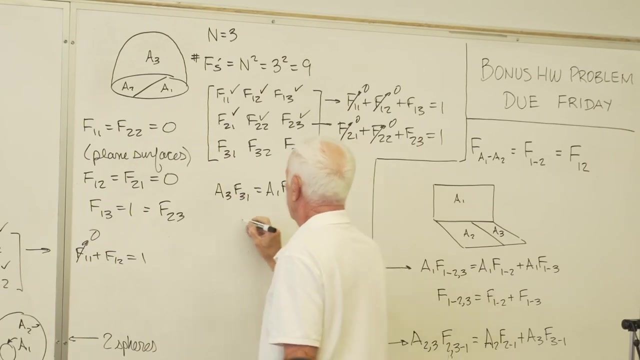 Reciprocity, These two guys, A3, F3 to 1, equal A1, F1 to 3.. I want F3 to 1.. F3 to 1 equal A1 over A3, F1 to 3.. F1 to 3 was 1.. 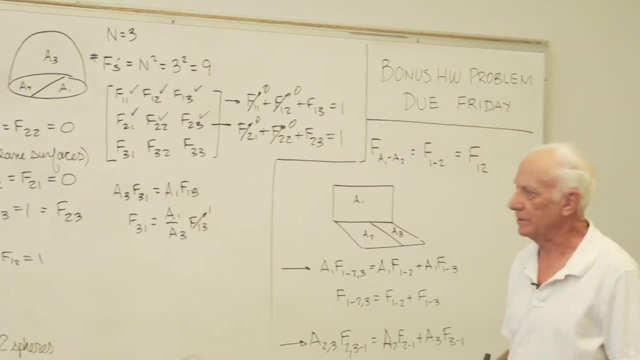 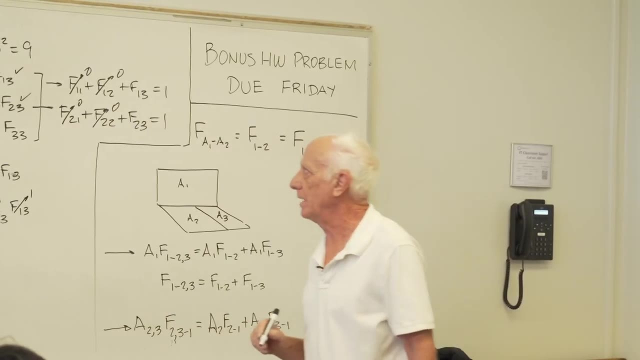 Do I know A1?? Yeah, it's half of a circle, pi r squared. Do I know A3?? Yeah, it's half of a sphere, pi d squared, divided by 2.. I got it: F3 to 1.. 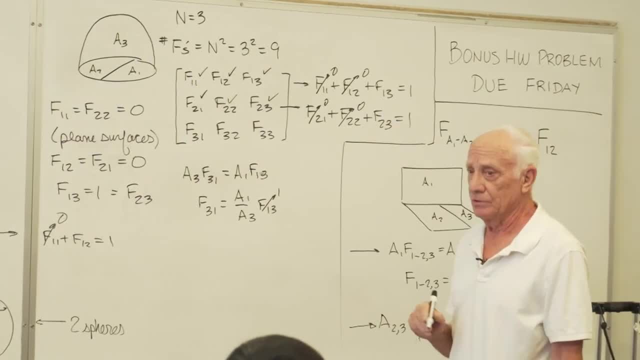 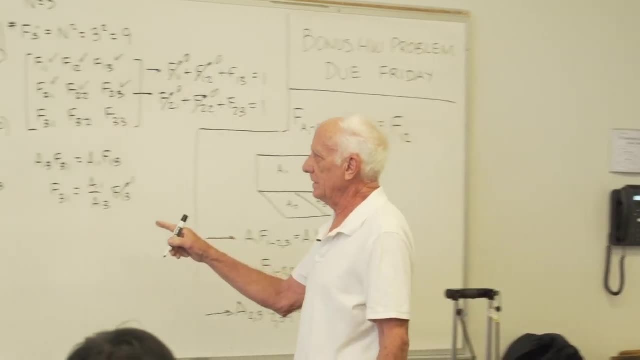 Do you think F3 to 1 is the same as F3 to 2?? Of course it is. What do you say? By observation, it's symmetrical. F3 to 1 is the same as F3 to 2,. 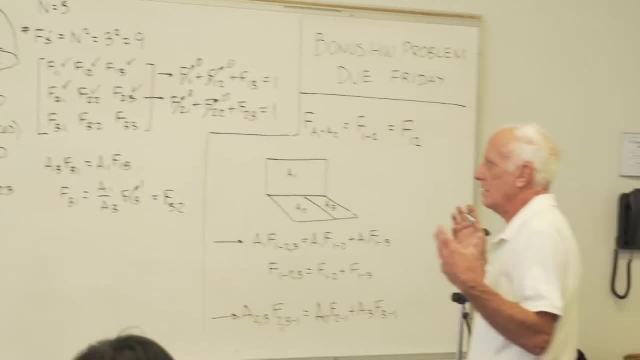 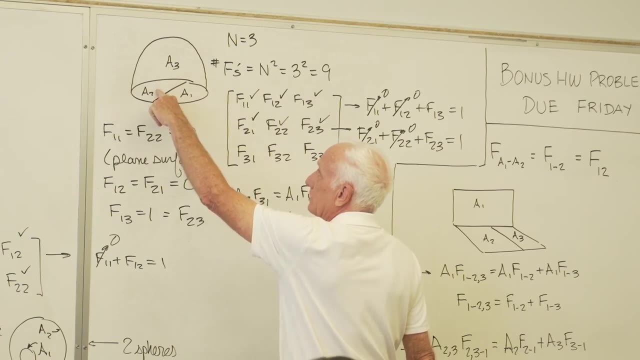 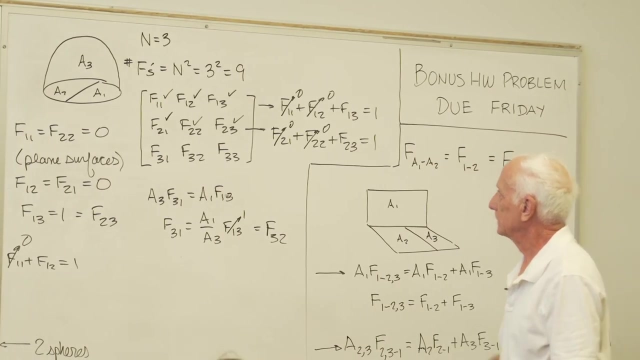 by observation. If you want to prove it, go ahead and prove it. Reciprocity: A3, F3 to 2 equal A2, F2 to 3.. What's F2 to 3? One Got it. 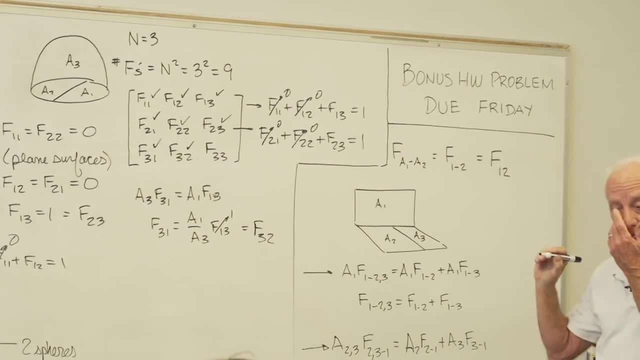 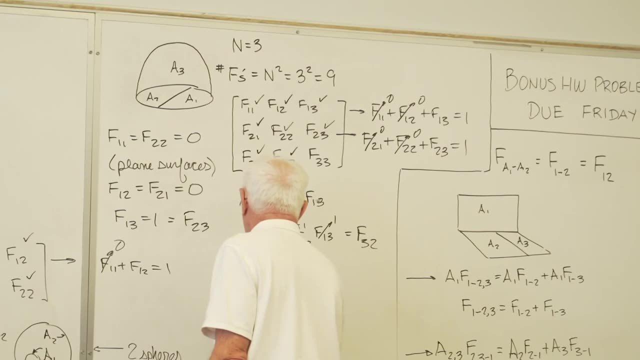 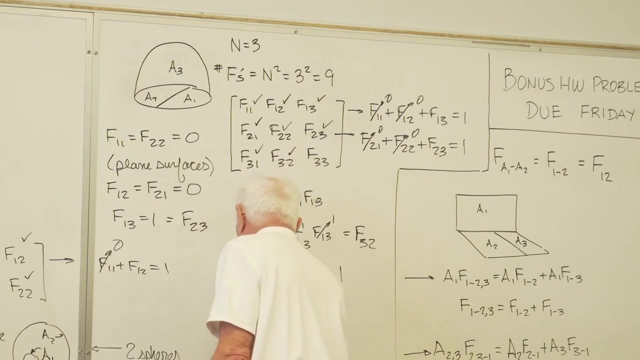 Got eight out of the nine. now One more to go F3 to 3.. I have to use the enclosure law: F3 to 1 plus F3 to 2, plus F3 to 3 equal 1, F3 to 3.. 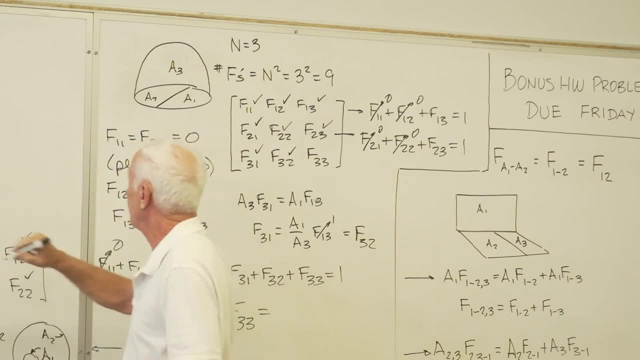 What is surface 3? again, It's concave. It's not zero. F3 to 3 is not zero. One minus 2, F3, 1.. Put that guy in there, Since they're the same, just two times one of them. 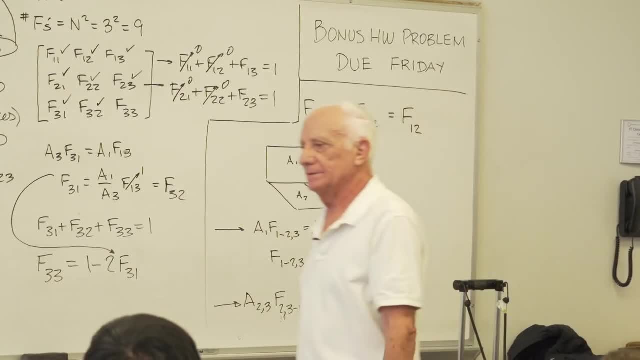 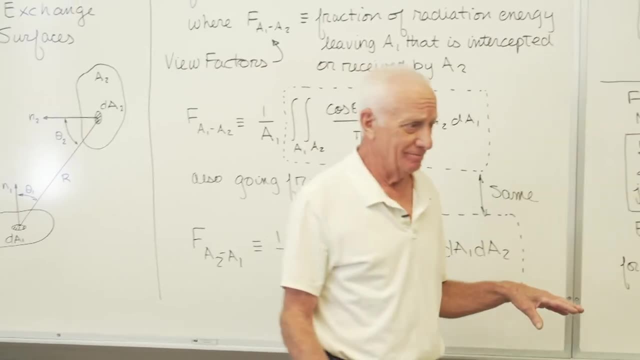 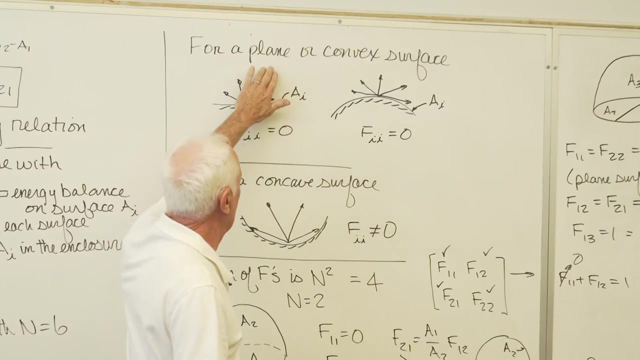 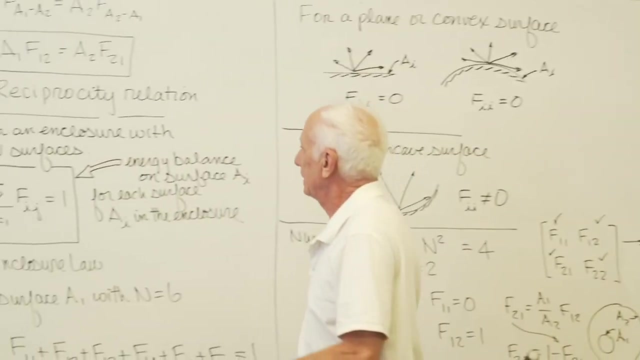 Okay, Six view factors. We didn't use tables, We didn't use graphs, We used bi-observation, The enclosure law, Reciprocity and understanding. is the surface plain, convex or concave? Let's do another one. I'll do it here. 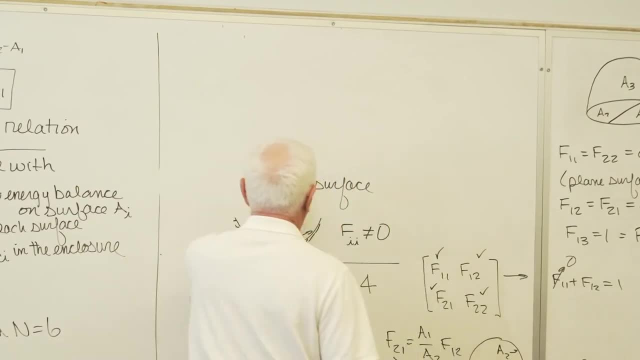 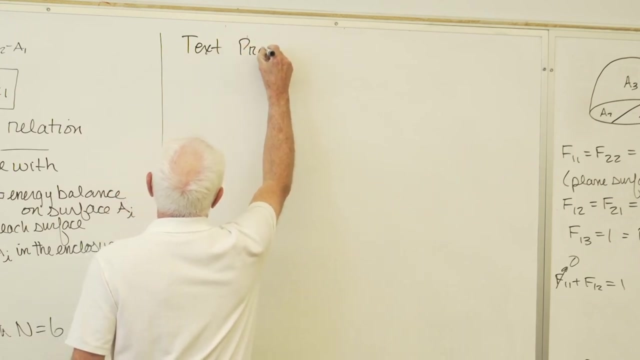 I'm going to look at the end of the chapter and I'm going to work a couple of real simple ones from the very first end of chapter, problem problem 13.1.. Let's see which one I want to work first. I'll work this one. There's 1,, 2,, 3,. 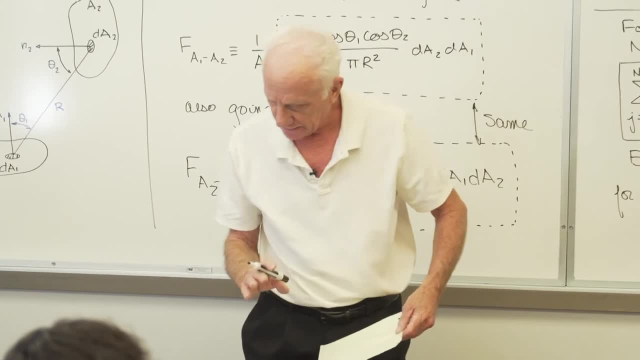 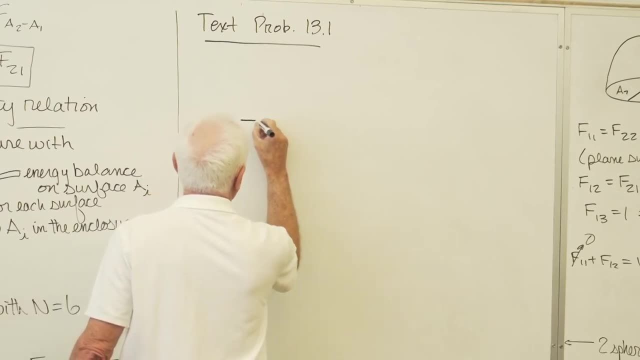 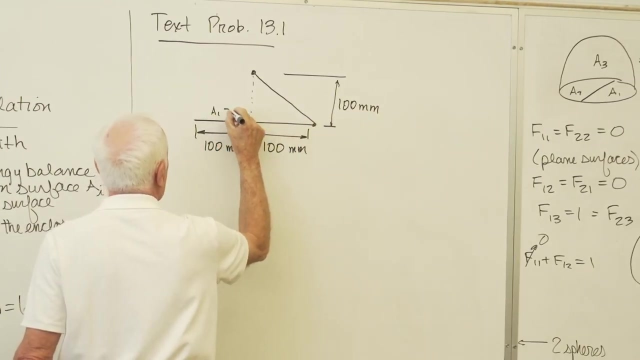 4,, 5,, 6, 8 different pictures. This is what it says: Find F2-1 and F1-2.. So here's a picture Directly above here. this distance is also a 100.. This is surface A1,. 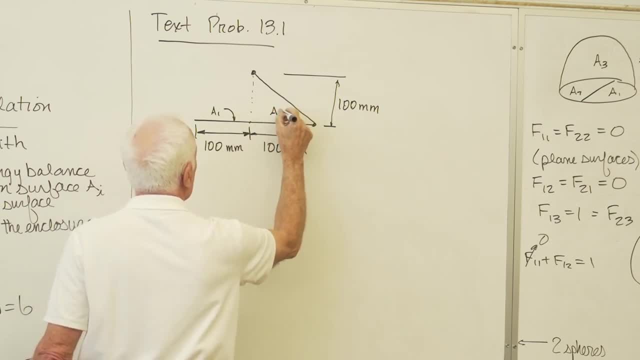 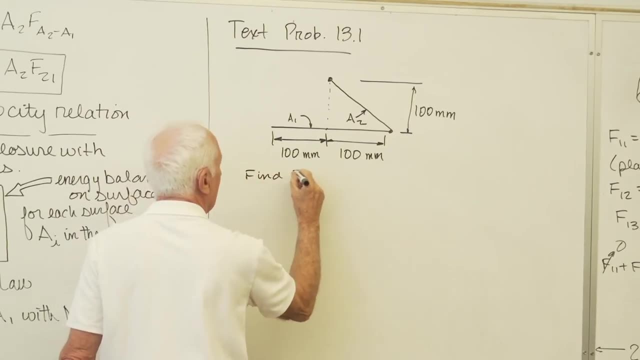 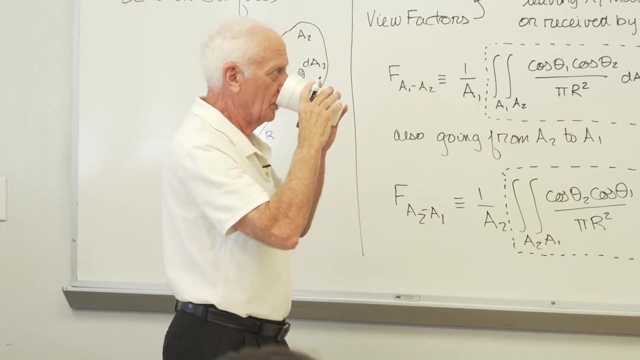 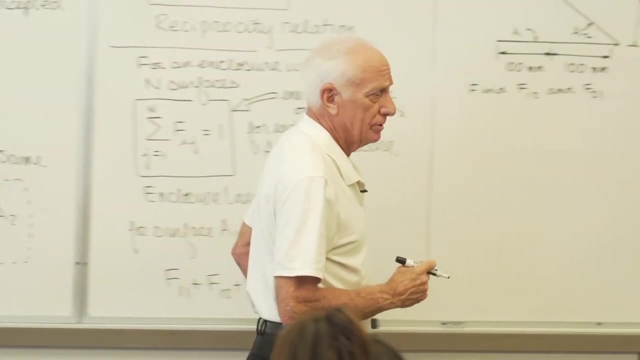 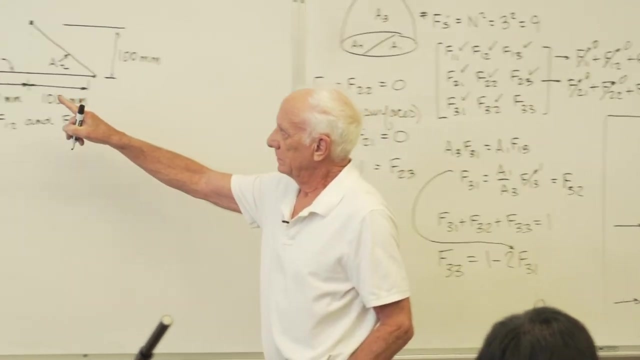 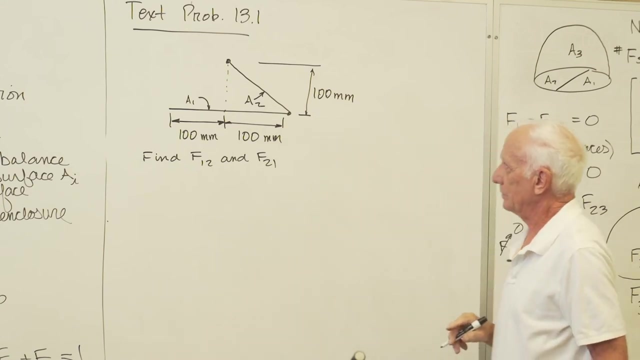 this is surface A2.. Find F1-2 and F2-1.. All right, It's not an enclosure, It's symmetrical: 100, 100, 100, 45 degrees A2, square root 2 times 100.. 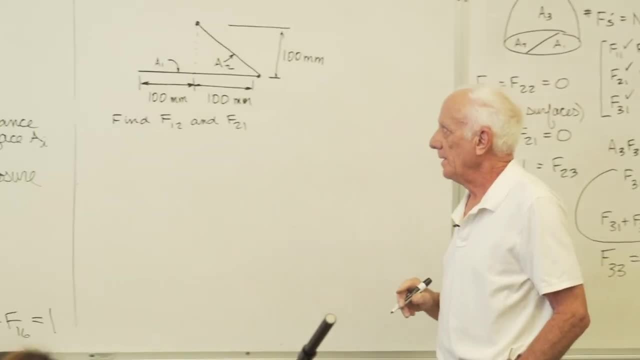 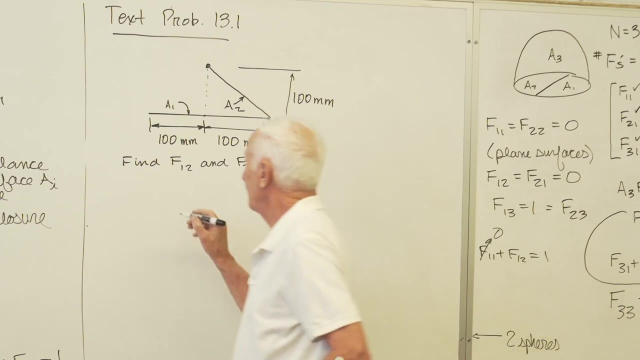 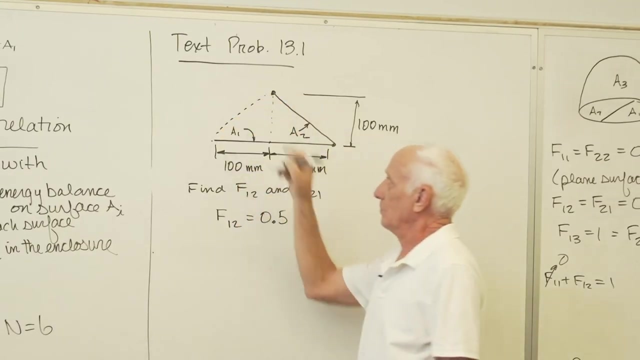 No graphs, no tables. Either you see it or you don't. Either you see it or you don't. F1-2 equals 50 percent, Half the energy leaving surface A1 is going to hit A2 and of course, half of it would go through. 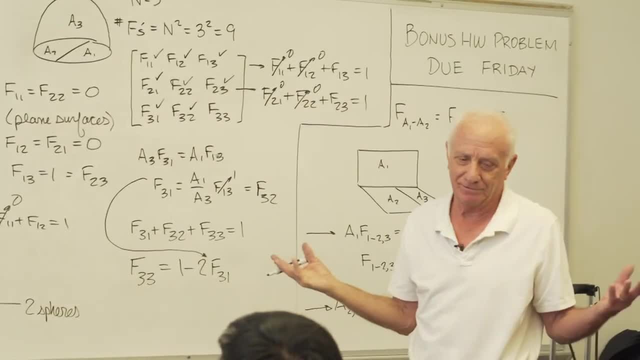 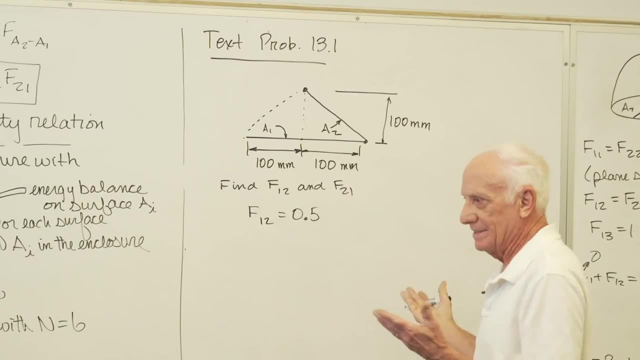 that dashed line right there? Of course it will, That's just 50-50.. But you don't use an equation, You don't use a table or a graph, That's it. You say that by observation F2-1 equal A1 over A2, F1-2.. 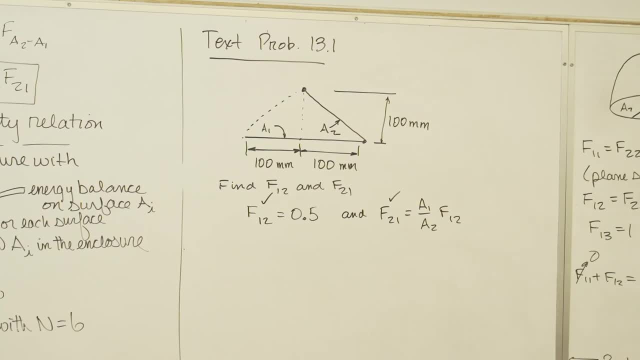 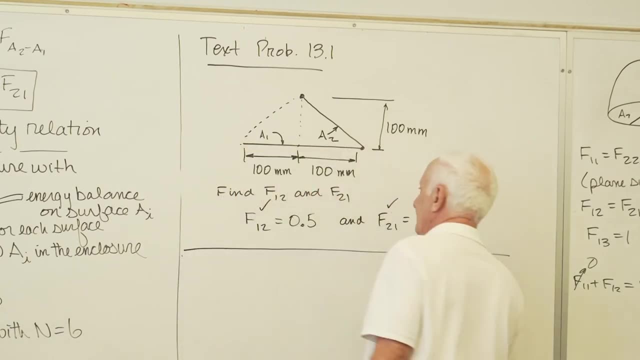 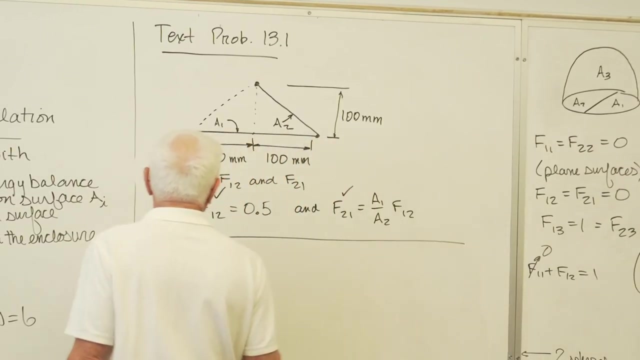 Got it. Got it. Done View factor: algebra plus by observation. Are they plane surfaces? Yeah, So F1-1 is zero, F2-2 is zero. This is D. I think I said Yeah, D. Do it again. 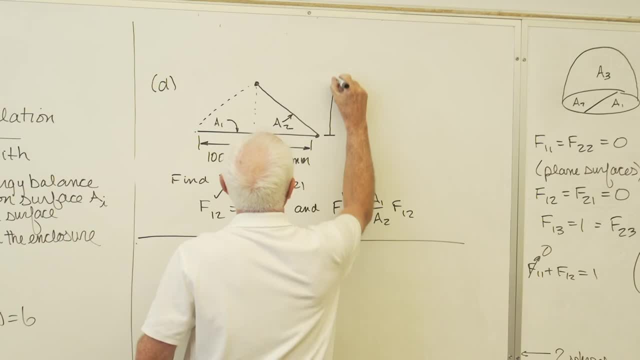 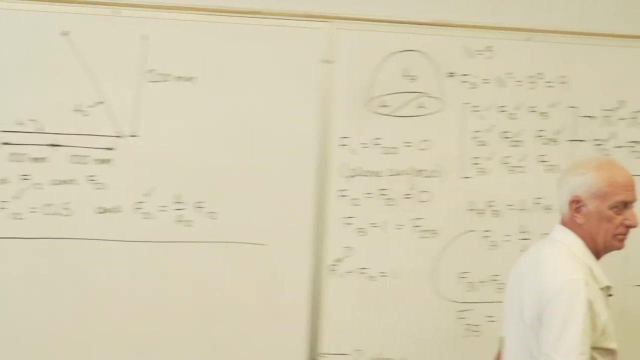 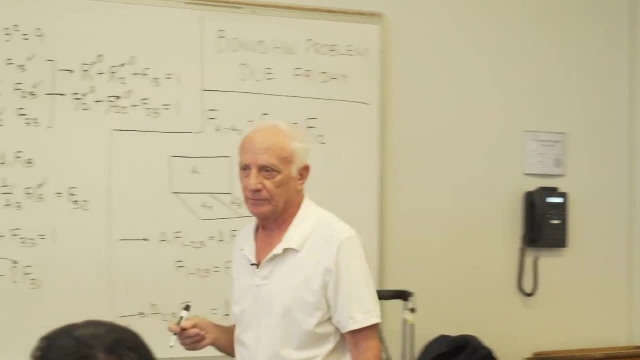 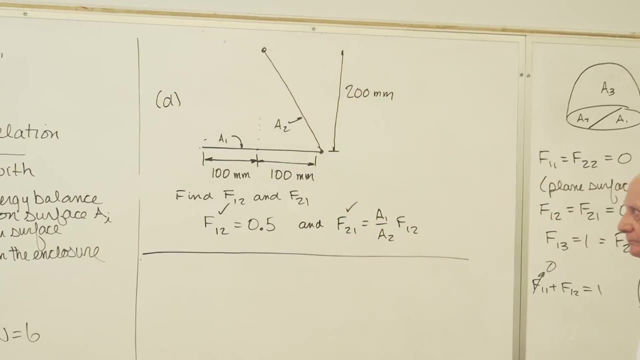 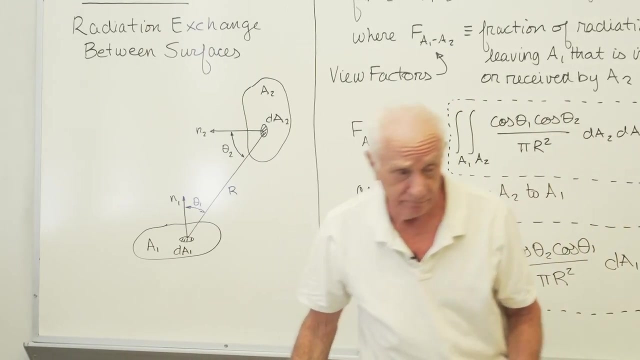 Half goes left, half goes right. Nothing's changed. Doesn't matter where you put that point Way up there by the screen, I don't care. Half goes left, half goes right. Let's try another one. Oh yeah, Okay, This is A. 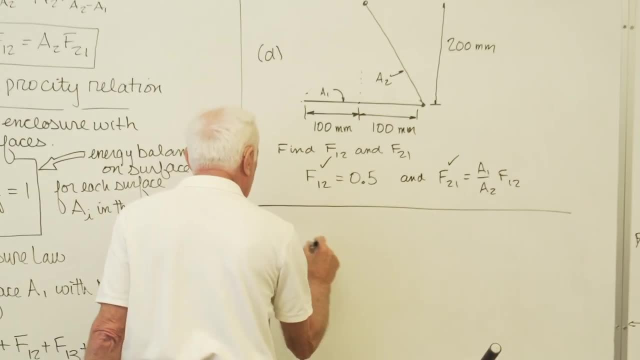 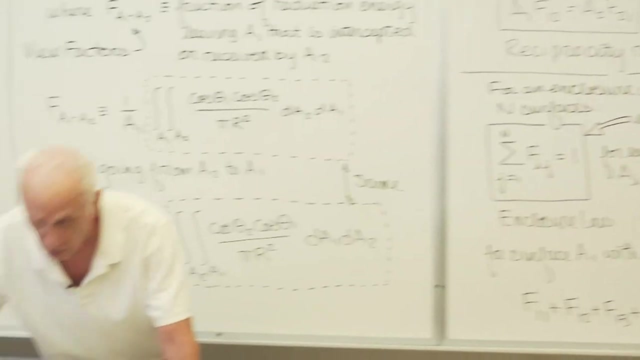 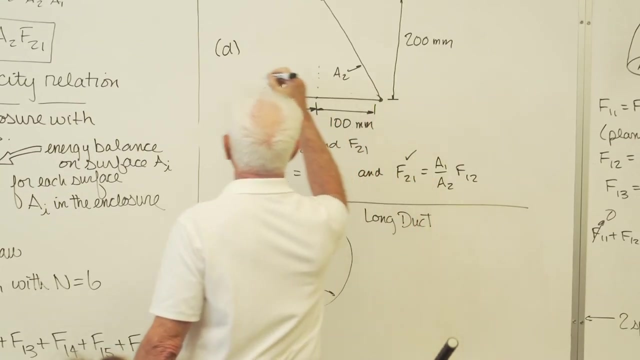 So A Here's A1,, here's A2.. Let me see what he says about this, The words that go with this. This is a long duct, Long duct. I'm going to put the words up here with Part D. 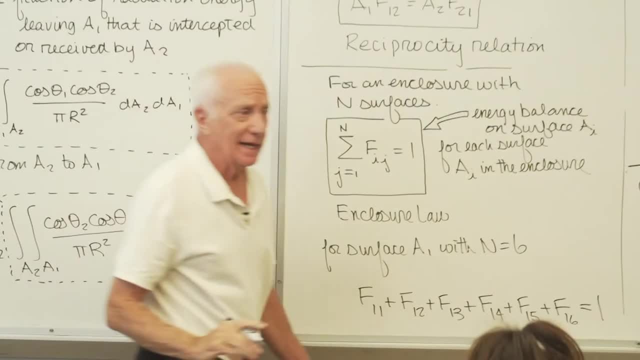 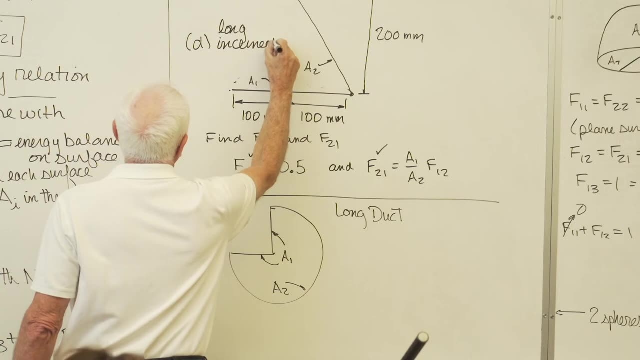 The words for Part D said long planes, long inclined planes. They go out that way a long, long way into the blackboard. that way, a long, long way. A long duct comes out of the blackboard a long, long way. 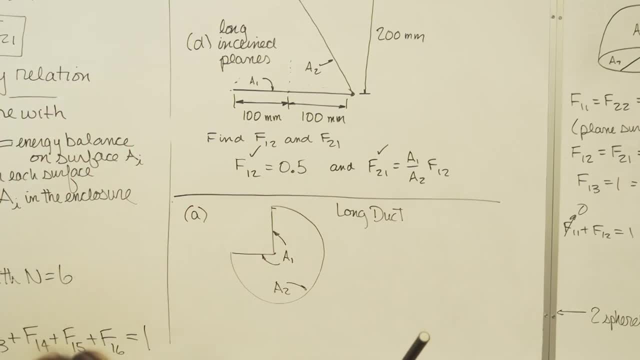 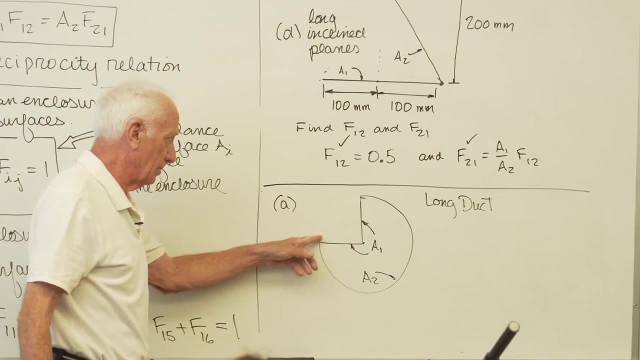 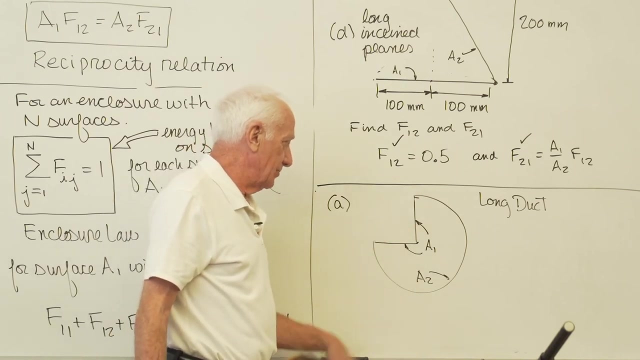 that way, and a long, long way that way. A1 is a combined surface, This area- you see what it is- The vertical area here plus the horizontal area there, Circumference Pi D, A2, three-quarters Pi D, A1, D. 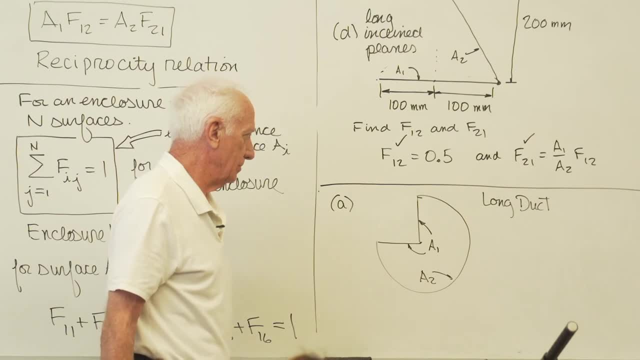 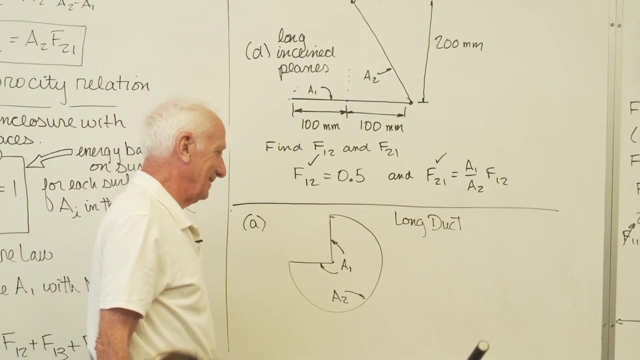 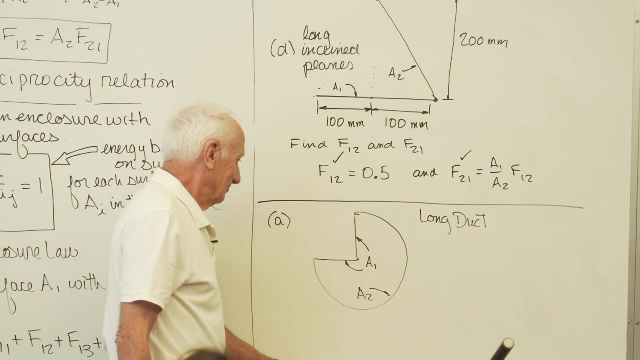 Radius D over 2 plus D over 2, equal D Is A1. a plane surface. Well, it's composed of plane surfaces, but it's not one plane surface. No, Is there something like a convex surface? Kind of like a convex surface? 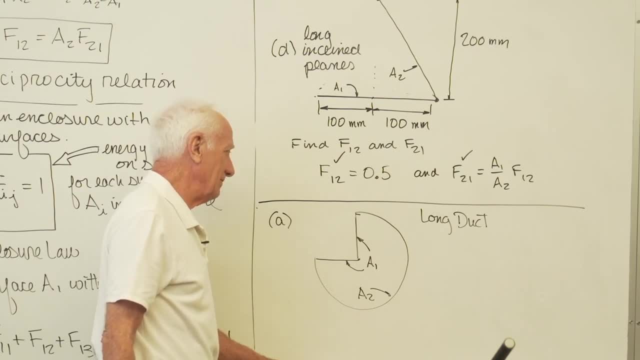 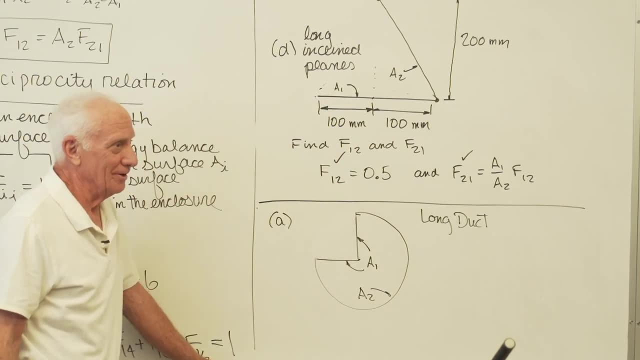 Yeah. What's the fraction of energy leaving A1 that actually hits A1?? Oh, it's 0.. What's the fraction of energy leaving A1 hits A2?? Oh, it's obviously 1.. F1-2 is 1.. 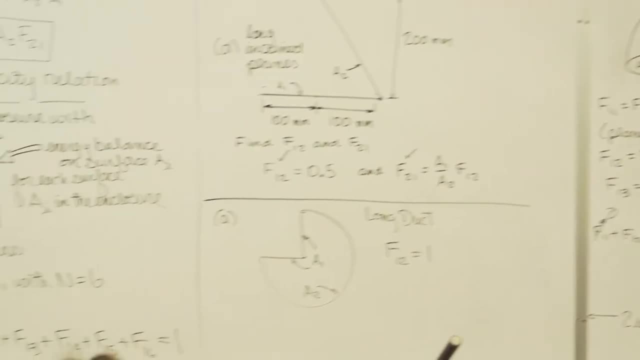 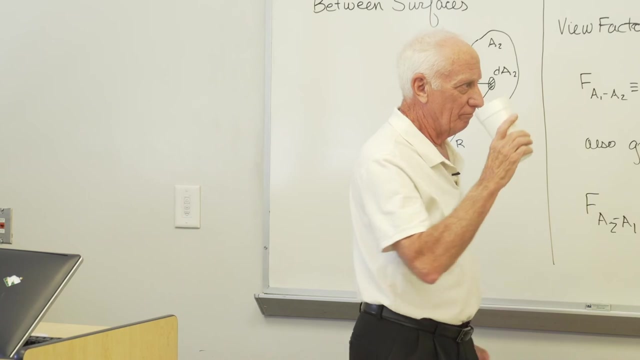 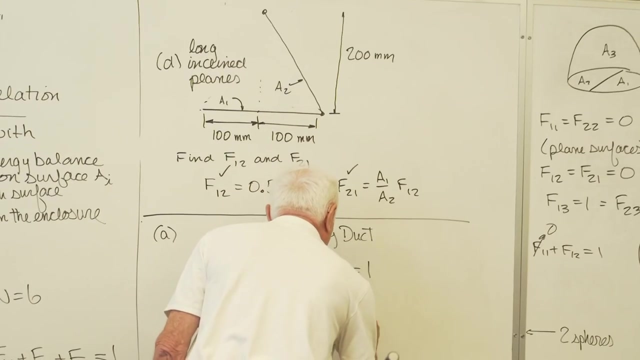 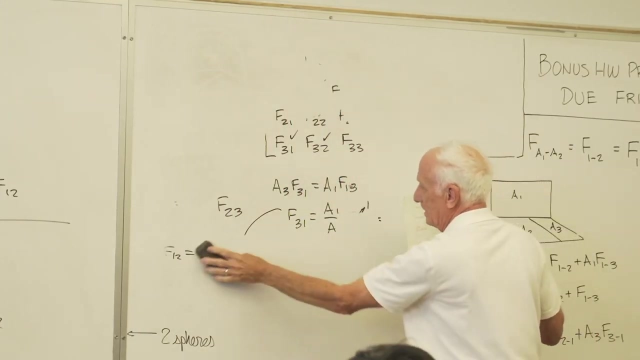 Do I use an equation No A, graph No A, table No, Either you see it or you don't. F2-1,, it's the same thing. Got it? I got them both Pretty much the homework in this part of. 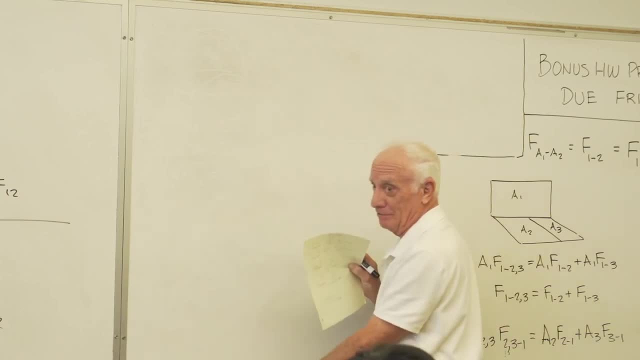 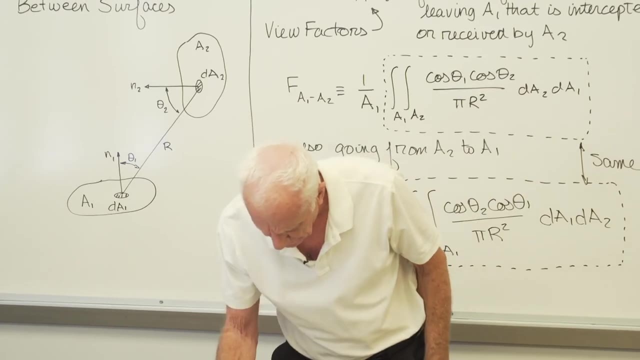 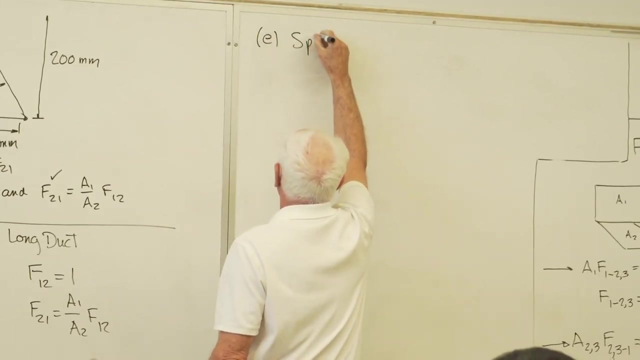 Chapter 13 is find the view factors. I'll do one more. E a sphere lying on an infinite plane. E a sphere lying on an infinite plane. E a sphere lying on an infinite plane. Okay, So here's a plane. 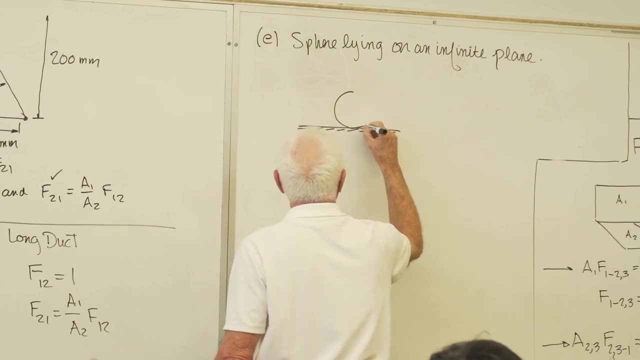 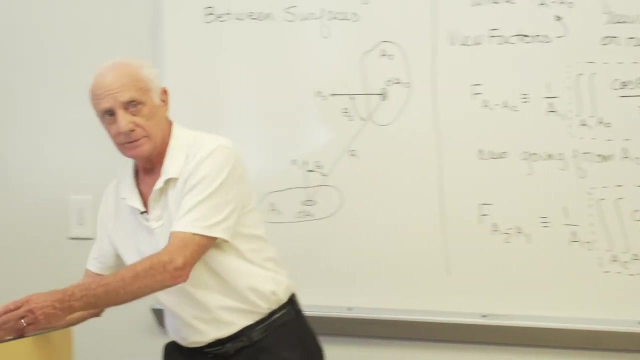 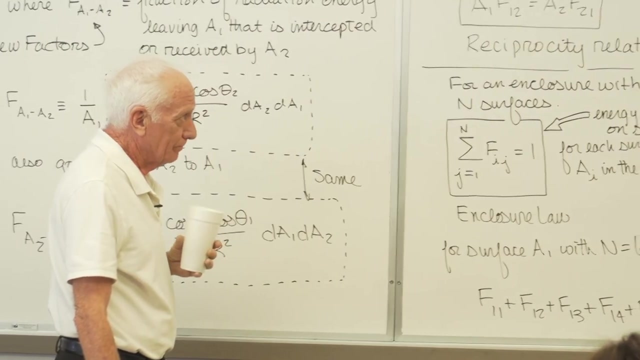 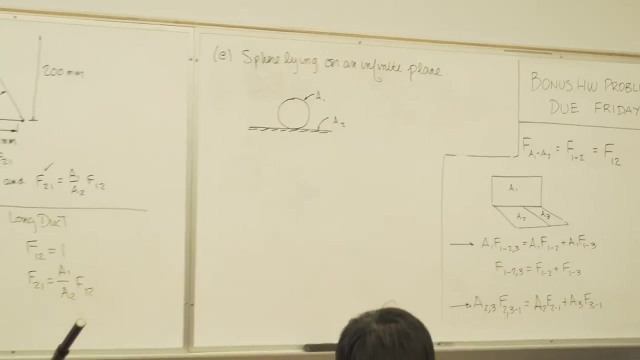 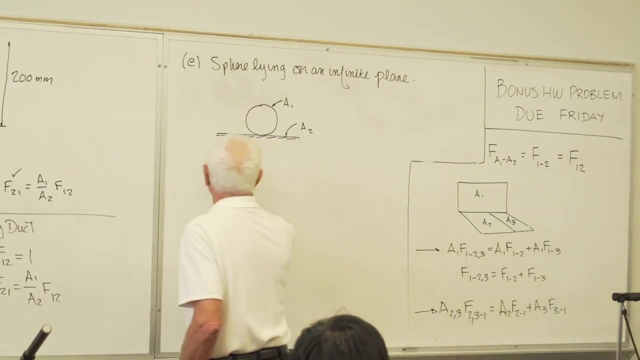 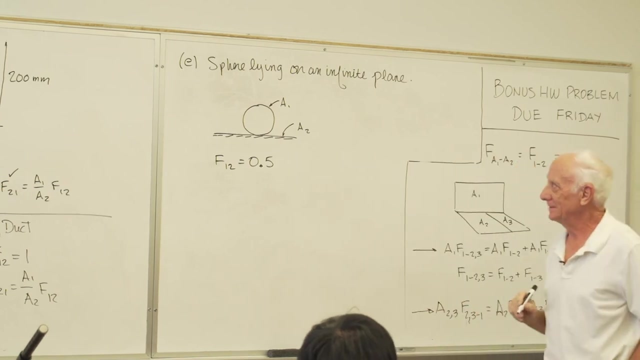 Here's a sphere: A1, A2.. Find F1-2 and F2-1.. This is a tougher one of the three. of course, Either you see it or you don't. Yeah, Half the energy leaving the sphere hits A2,. 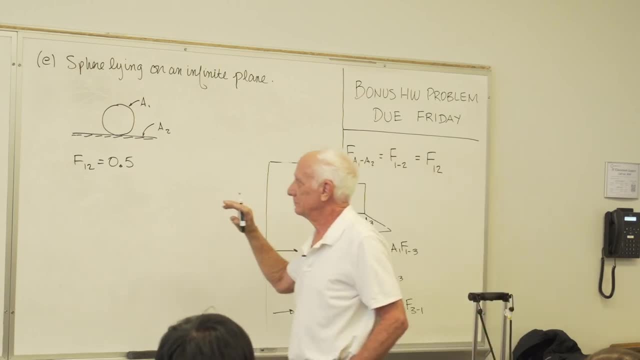 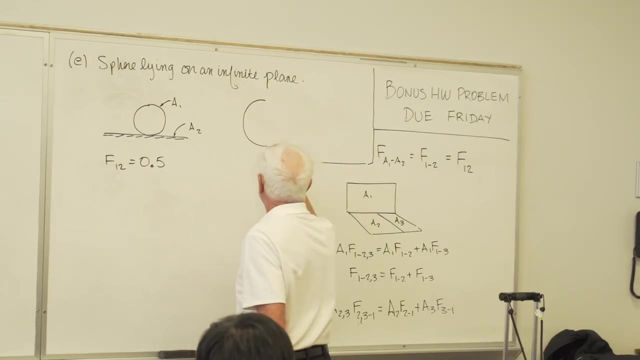 and half goes out. Above it There's a sphere and a bigger sphere. Do you think half the energy of the little sphere ends up striking the top half of the big sphere? Oh yeah, Do you think half it ends up striking the bottom of this big sphere?